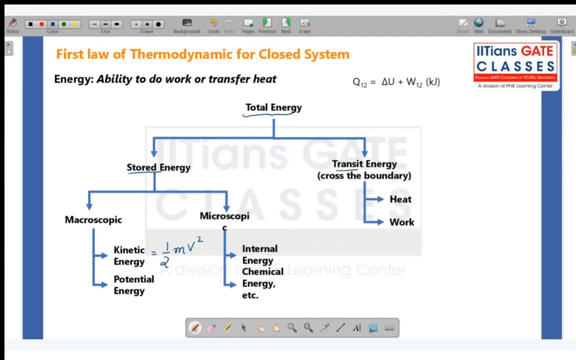 Okay, Thank you so much. Okay, So let me start one more time. Let me Okay. So what I was saying is this diagram you may have seen already. I have already, I think, shown you earlier. Now here, total energy is basically two types of stored energy and transit energy. What 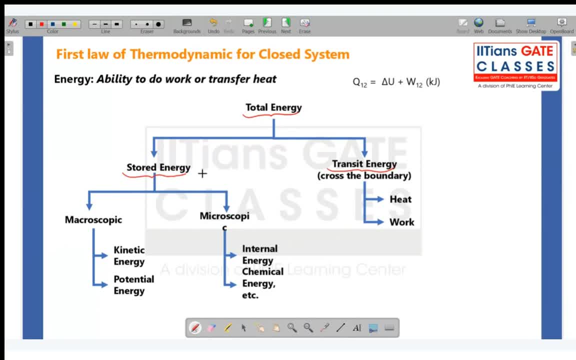 is stored energy. Stored energy is basically: if you have some mass, any mass, then that mass will store energy in the form of kinetic energy, potential energy, internal energy, chemical energy, magnetic energy and other kind of energies. Okay, Now this I am not. 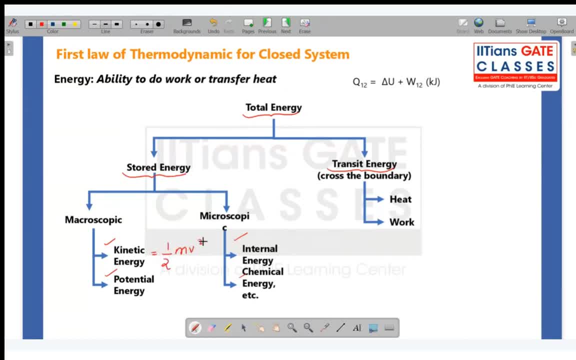 going to discuss. I think you are all aware of what is kinetic energy, mv square. We all have been doing this from 11th and 12th, Okay, And what is potential energy, mgz? What I am going to discuss? I will discuss a bit about internal energy, heat and enthalpy. 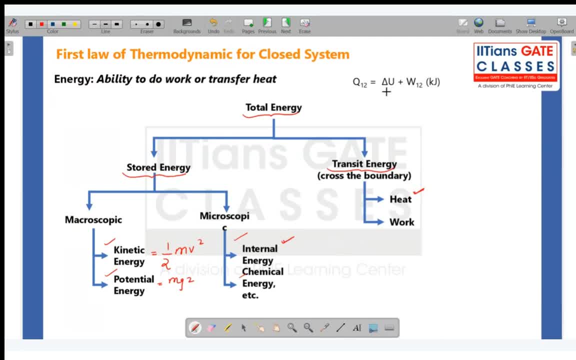 These are the three things I am going to discuss, And then we will move to open system. Okay, So you see. work transfer- we have discussed in detail- Heat transfer, internal energy- we are going to discuss- And anyone can tell me what is this? Quickly tell me what is this. 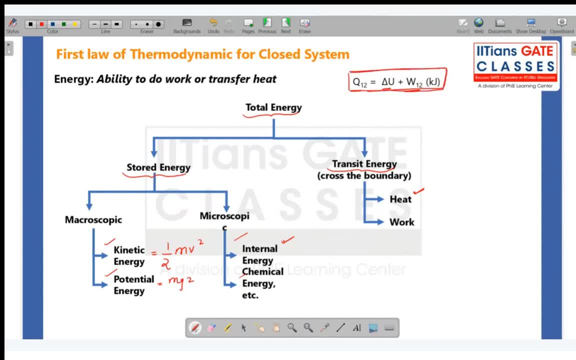 Quickly, What is this box That I have marked? highlighted Anyone First law? for what? For what Process? and for a closed system? Yes, for a closed system, Okay. So be very clear about what we are talking about. Do not get confused about. okay. I mean, you use some, you have some equation. 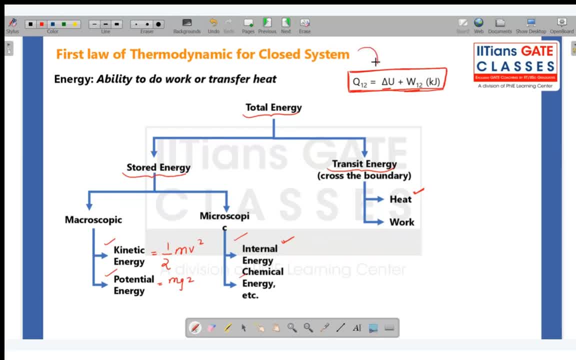 you apply everywhere. You know you can't do that. Okay, So it is basically for a closed system And for a process- I very clearly defined this- And for a cycle. basically, del u becomes zero because it is a property And q12 is equals to w12.. This is first law of thermodynamics. 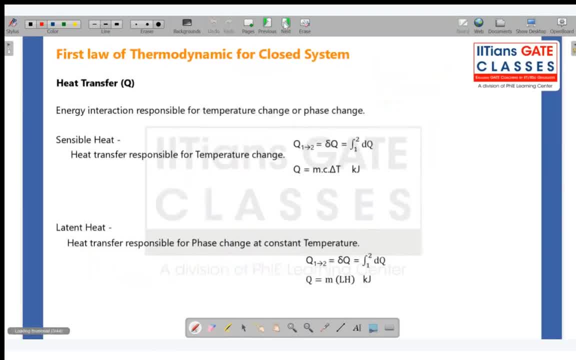 for a cycle. Okay, Let's move ahead Now. what is heat transfer? Basically, heat transfer is whenever energy interaction takes place that is responsible for either temperature change or phase change. Okay, That can cause. So if energy, any energy- is coming inside, okay, Enthalpy comes. Yes, we will discuss. 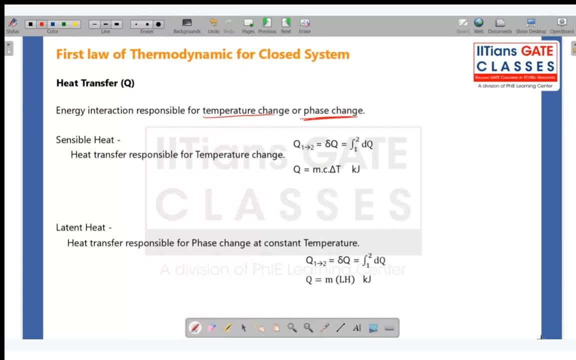 that, Don't worry, Don't go ahead. I mean no, we will discuss that. Okay, And that we will discuss today. So, energy interaction: whenever energy is consumed or it is, I mean it is coming in or going out and it is causing either temperature change or a phase change. you can say that. 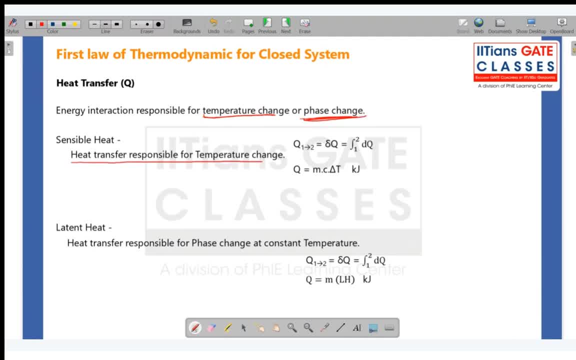 heat transfer is happening, Okay, Okay, for temperature change is called is called a sensible heat. okay, here, heat transfer that is responsible for temperature change is called a sensible heat. now, if heat transfer is causing phase change, then it is called as latent heat. now, let's see, you have this. 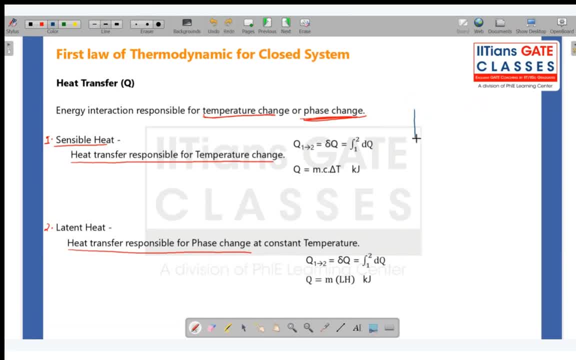 you have this bucket, then in this you have some water. this water is that, let's say, 20 degree Celsius. okay, now I am giving some heat. may be I have put on an electric heater or something- I mean, there can be so many ways- or I am burning some coal here. 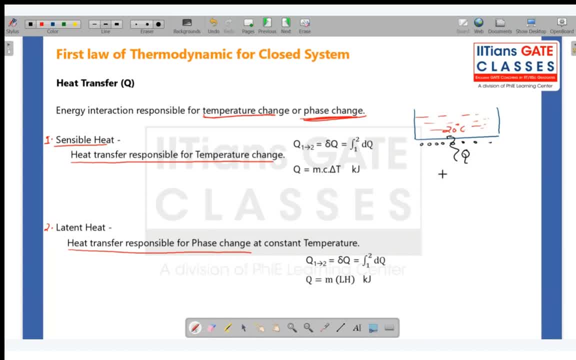 and there are so many way that can give you, so I'm giving some heat and then it's temperature rises to, let us say, 50, so this was its initial temperature. after some time, the final temperature is 50 degree. so which heat is getting? what is? 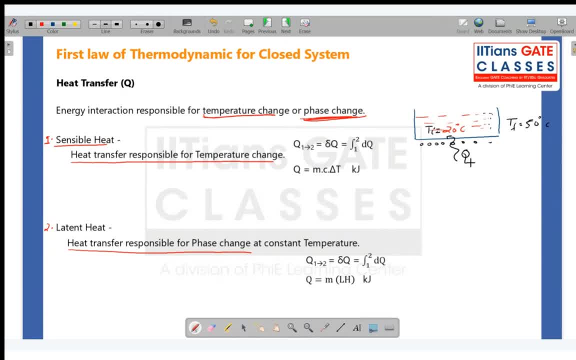 this heat? what is this heat that is getting transferred quickly, quickly? answer in the chat. that is sensible heat. yes, sensible heat, very nice. okay, now I keep giving, I keep giving this heat. I keep giving this heat and let us say, this temperature reaches, this temperature reaches 100 degree Celsius and I still keep giving heat. I 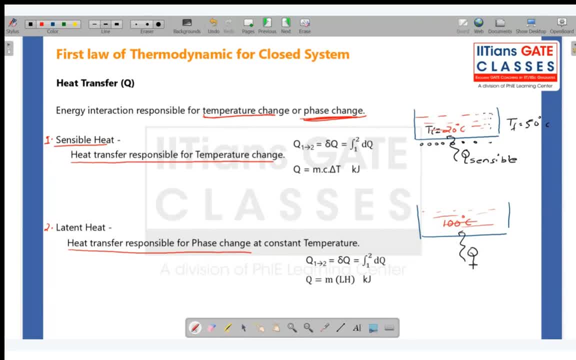 still keep giving here. then tell me what will happen. then tell me quickly what will happen. any idea? yes, so this water will start evaporating. there are so many things that you can say. so it will convert into steam, it will start vaporizing, it will start having phase change, it will start evaporating. so there are so many ways. 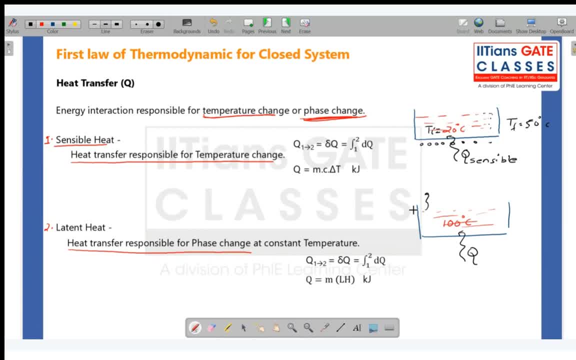 of saying the same thing, but basically it will convert from liquid to vapor in a in very simple way and when that is happening, basically one is converting into gaseous phase. liquid phase, which is water, is getting converted into gaseous phase, which is steam. so phase change is happening and the heat 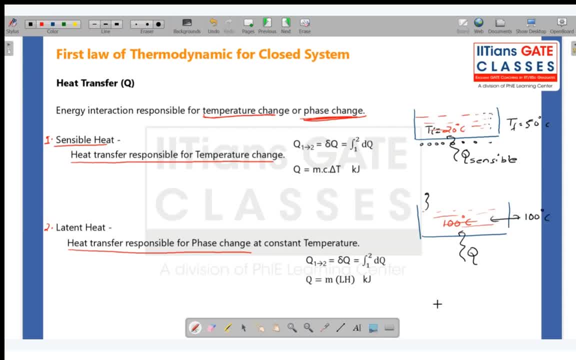 but this phase change of course will happen at 100 degree celsius. okay, it will not change, it will remain at 100. okay, and that heat that i am transferring is called as latent heat is called as latent heat, okay, so, basically, the heat that is involved during phase change is called as latent heat. 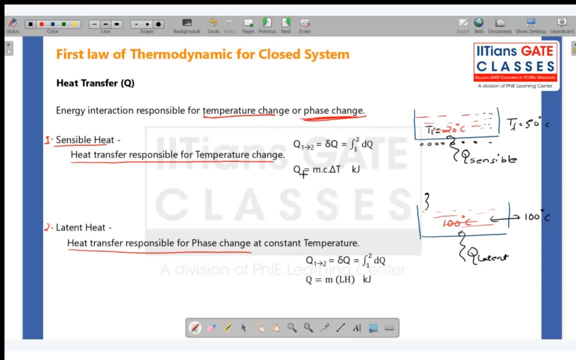 the heat which is responsible for temperature chain is called as sensible heat. okay, so sensible heat you can calculate by this, because it is proportional to mass, specific heat and temperature difference. and latent heat you can calculate by this. you cannot use this formula to calculate latent heat because delta t is zero. you see, when phase change is happening, delta t will be zero. 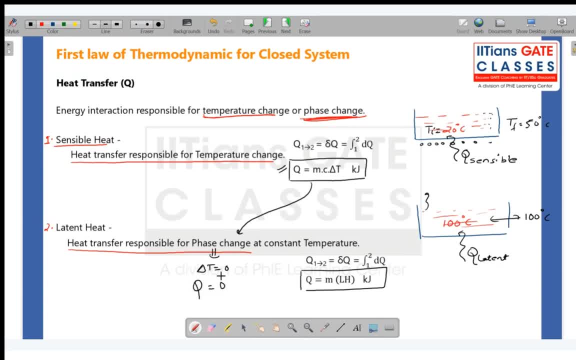 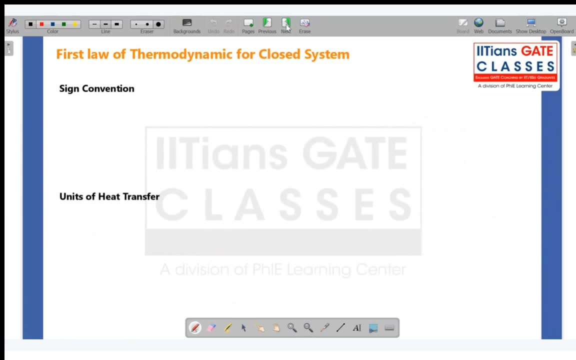 so, if you use this formula, q will be zero, but that is not the case. you are transferring heat, okay. so you cannot use this. you cannot use this. you have to use this formula. okay, now sign convention. i hope you are all aware of sign convention. now, when let's say, you have, this is your system. 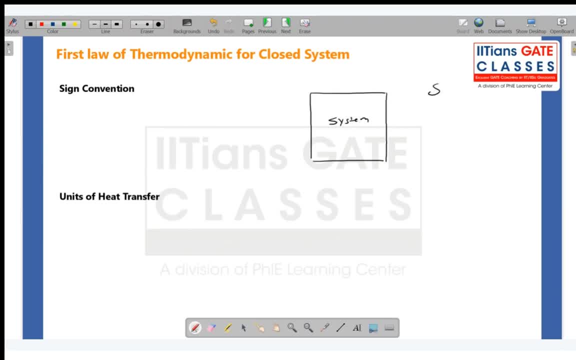 and outside it is surrounding. okay, now i am transferring heat to the system q in. heat is getting transferred, so this heat transfer q in is basically positive. it is always considered as positive. heat supplied to the system is taken as positive and it is just a random assumption. okay, you can take it negative as well. 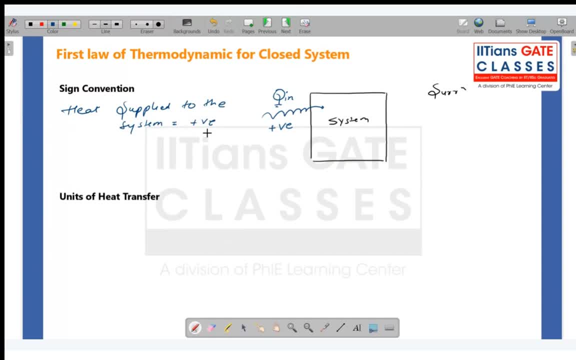 but whenever you are solving a question, you have to always assume a particular sign. okay, you cannot. you know, in the same question you cannot take q in somewhere negative and q out somewhere negative. okay, so you have to follow this one, follow only one convention. now, if heat is going out, if this system is rejecting heat, 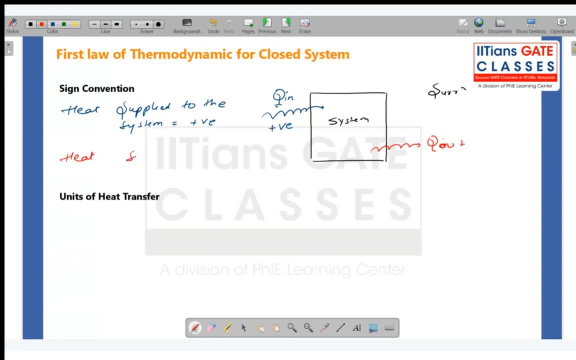 then heat supplied. we say heat supplied by the system, by the system, and it is negative. so it is negative, very simple. okay, now what are units? q is equals to m, c, d, t. what is mass? this is kg specific heat, kilojoule per kg kelvin and temperature difference is kelvin. 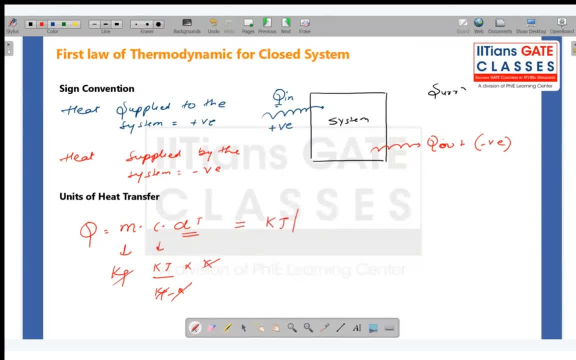 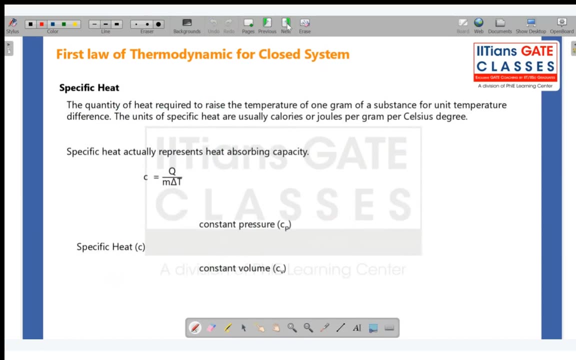 so this will get cancelled and basically units are kilojoule, mega joule or these things. okay, so these are basically the unit. the mostly used unit is kilojoule. okay, now, what is specific heat? so basically, you see, your main equation is: q is equals to. 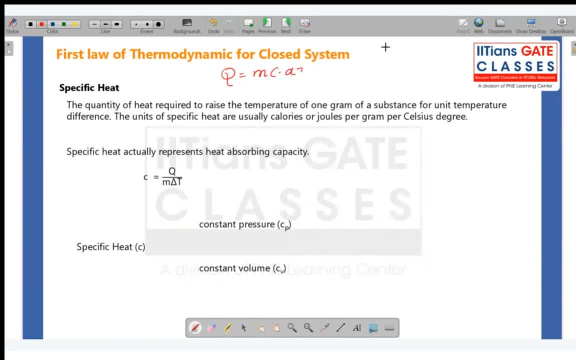 m, c, d, t. okay, how did it come? we saw that q is proportional to mass experimentally, and q is also proportional to temperature difference. if mass is more, we need more heat for the same temperature difference. or if temperature difference is more, then for the same mass you are transferring more heat. so experimentally we have seen, and then we added: 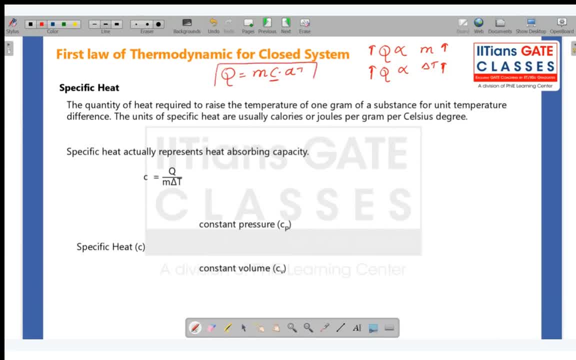 a proportionality constant c here. okay, so that's it. that is how we got this equation. now this is the defining equation for specific heat. so specific heat is basically represents the heat absorbing capacity. now I don't know if you okay heat transfer. if you have done, you may have already aware of heat thermal conductivity. so, like we define, 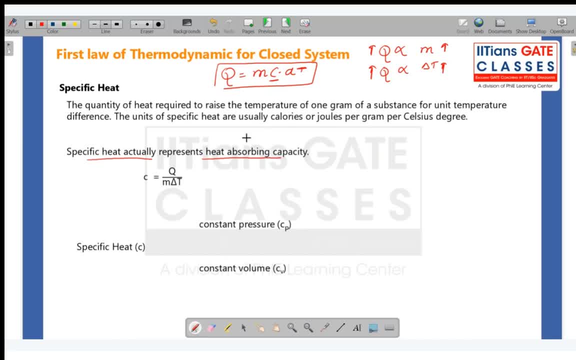 it there. similarly we define it here that what do we do? we say specific heat very clearly. you know very I mean what I am saying. just pay a little more attention here. specific heat is the quantity of heat required to raise the temperature of one gram of substance. so let's say you have some mass of. 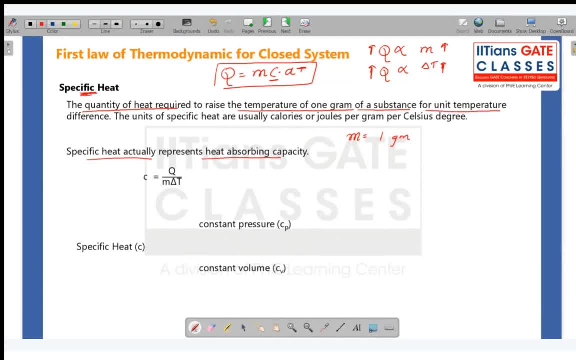 one gram, okay, and you are raising one unit temperature, difference of Delta, T is equals to one. so if you put in this equation, so c is equals to Q upon one into one, so basically, if you have one gram of mass and you are changing its temperature to one degree Celsius, okay, or? 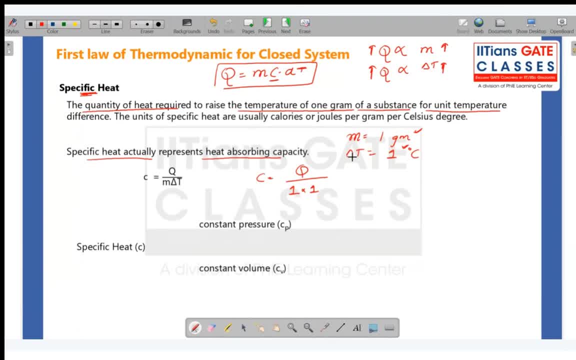 what unit, whatever, because Delta T Calvin in degrees Celsius will remain same. it will not matter. so whatever amount of heat that you require, whatever amount of heat that is required is called as sensible heat, is called as sensible heat. okay, so it is not. i mean, i'm just telling you this, but 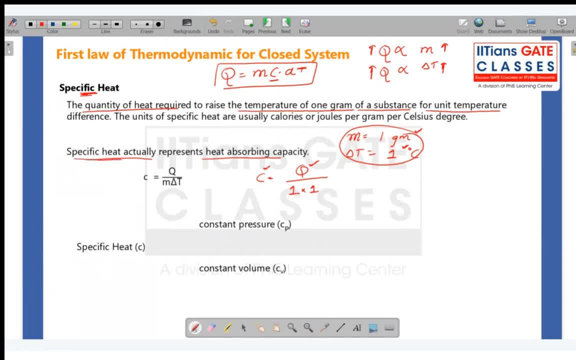 basically, to understand its significance, you have to understand that it gives you the heat absorption capacity. you see, look, q is equals to m, c, dt. so let us say mass is constant. okay, so when mass is constant now, uh, if you are giving, for example, you are giving. 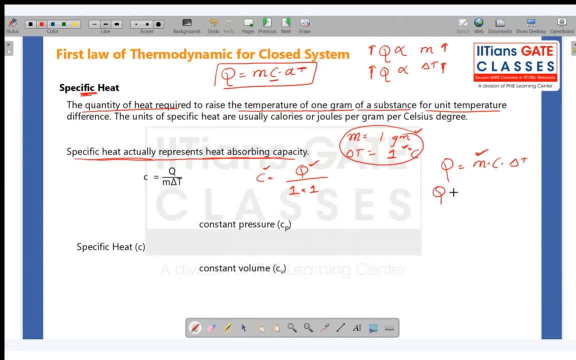 just one second. let me explain it by numbers. if q, you are giving 100 units, okay, so c, let's say it's 50, it's 60, okay, so what will be delta t? what will be delta t? delta t will be- uh, let me write it- 10, actually not 60, so that you can directly divide it if i say it is. 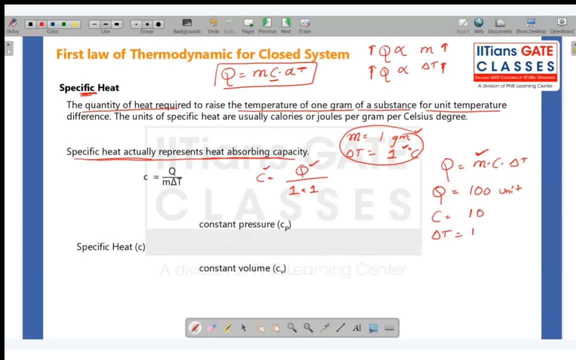 10. then what is delta t? delta t will be 10. okay, now, if i say q is same, c is, let us say 20, so what is delta t? delta t is 5. what does this mean? let me explain. what does this mean. it means if a body has higher specific heat capacity, if a value, if a body has 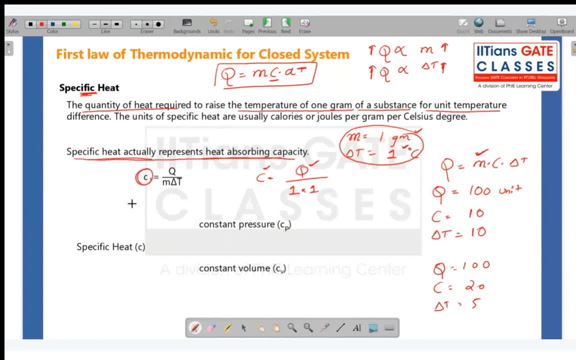 high c. it means it you keep giving it heat, it will keep absorbing heat, it will not allow the temperature difference. i will repeat it again: okay, if a body has higher specific heat, then if you keep giving heat, it will keep absorbing heat and it will not allow a temper higher temperature difference, okay. and if it has, 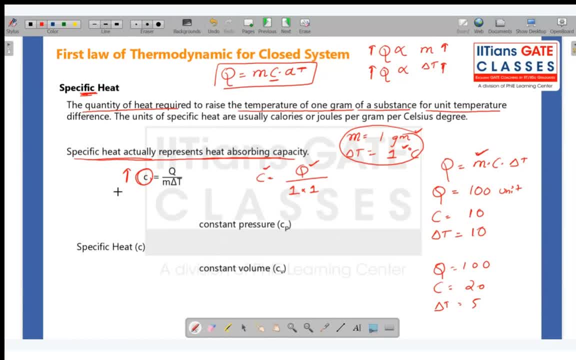 low specific heat, then the temperature difference will be higher. okay, so if i ask you one first of all, tell me, is this clear? this much is clear: if a body has high specific heat, then for the same heat transfer, temperature difference will be less. okay now, and can anyone tell me? can anyone tell me that? 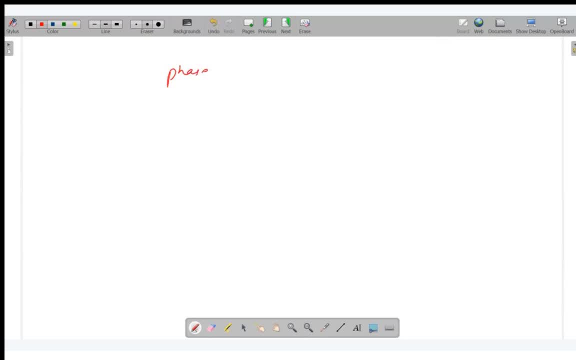 when phase change is happening, when phase change is happening, phase change, then what is the specific heat of the fluid? what is the specific heat of the fluid? any guess? no, not zero. zero means very high temperature difference by, you see, delta q, which equals to c, into delta t. i am not saying zero, but let us say: 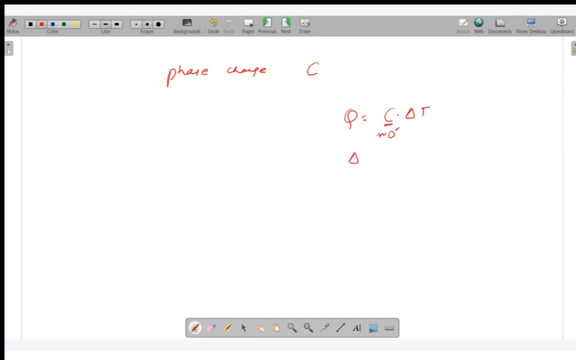 tends to zero. so if it tends to zero, that means delta t will be tends to infinite, okay, basically, when phase change is happening, c is infinite. so basically, you see, if it is water, you keep giving heat, you are giving. yeah, yes, infinite, okay, so you keep giving heat, you keep giving heat. 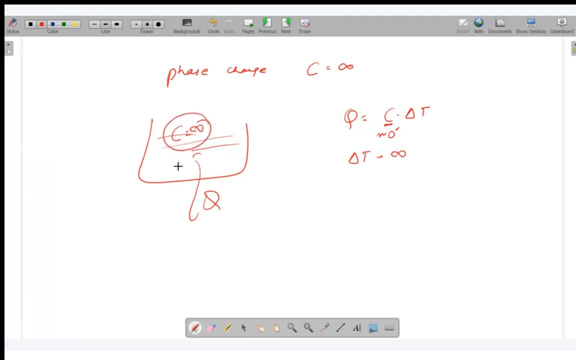 it's c is infinite, very high c it is. it keep absorbing heat and it is not letting any temperature say change, so it is equal to zero, okay. so again, if c is high, delta t is low. for say: okay. so again, if c is high, delta t is high, so it is equal to zero. okay, so for same heat transfer, c is 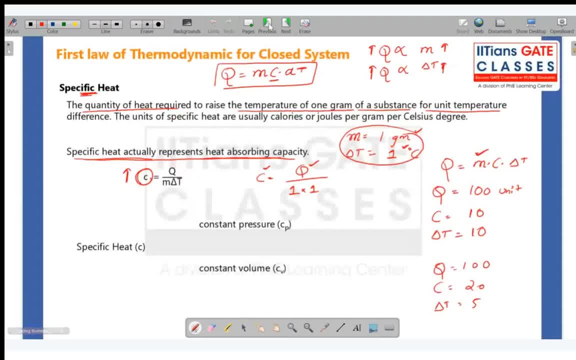 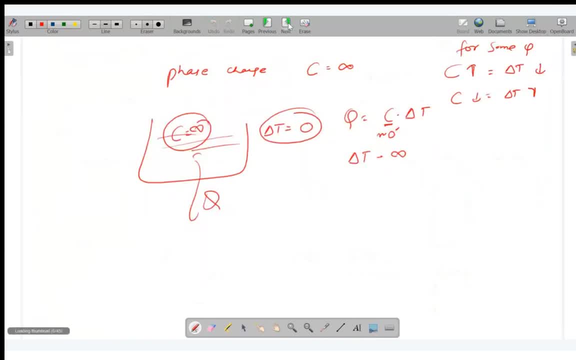 low, okay, for corn and plant heat transfer high. I hope now it is making sense. okay, now, specific heat is basically two types: constant pressure and constant correct. okay, let's see them. how about constant volume? so i hope you. how about constant volume? so i hope you remember. 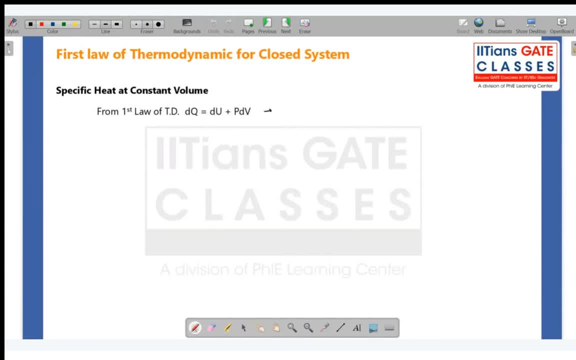 this formula: first law of thermodynamics for a process. now I am talking about constant volume. I am talking about constant volume. So tell me constant volume. DW is zero, right, Because DV is zero. Yes, Quickly, You have to be more, because 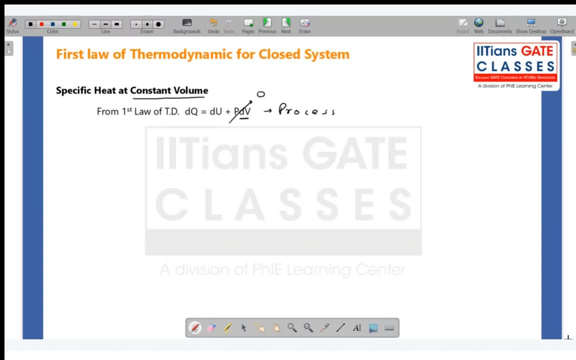 I don't want to wait for your answers. You have to say yes, no if it's clear. Constant volume process: DW DV is zero, So this term will be zero. Yes, If this is zero, then that means DQ is equals to DU, So I can write heat transferred. 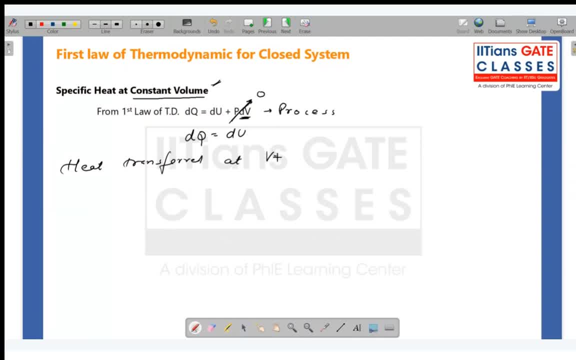 at constant volume increases the internal energy of the system. It is only if you are giving heat. it is only Changing the internal energy, because the work- no, it is not doing any work, Work is zero. Okay, So basically C is equals to DQ, upon. basically I can write here: DU is equals. 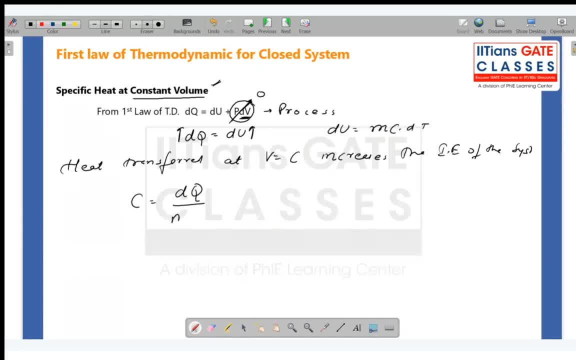 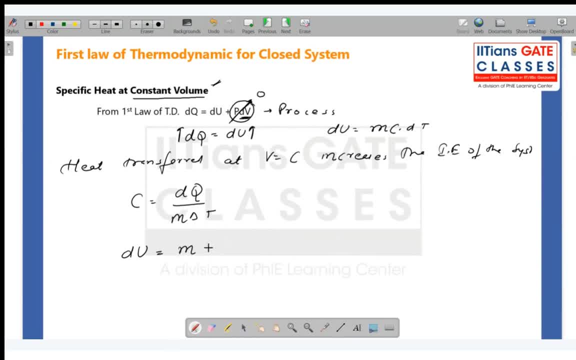 So DQ is equal to DU is equals to MCV. This is basically: if I put here CV, this will be this constant volume. sorry, constant volume, Okay, CV. delta T, Okay, T1 to T2.. So this is basically heat transfer for constant volume. I have already proved this for you in the 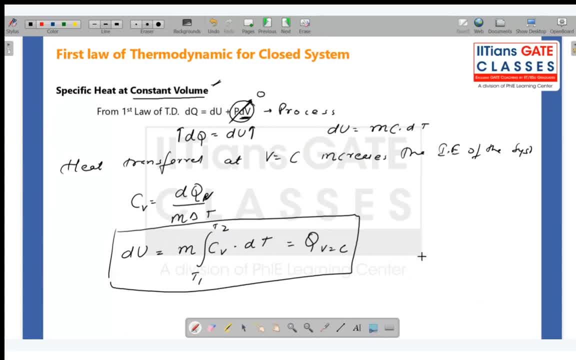 last given you this equation in the last class as well, that for constant volume, q is equals to delta u. but i am just moving this for you, okay. now what about constant pressure? so constant pressure is again. this is also. i have done it for you, okay, du plus, i know it is constant pressure, so i can. 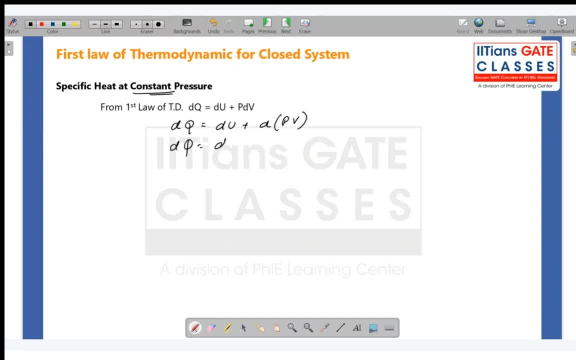 take p inside. in this last class i have done the same thing. dq is equals to d, u plus pv, dq is equals to dh. so can i write here that heat transferred at constant pressure increases, increases the enthalpy of the system. now, what is dh? dh is equals to m, cp, dt, so i can write t1 to t2 and this is: 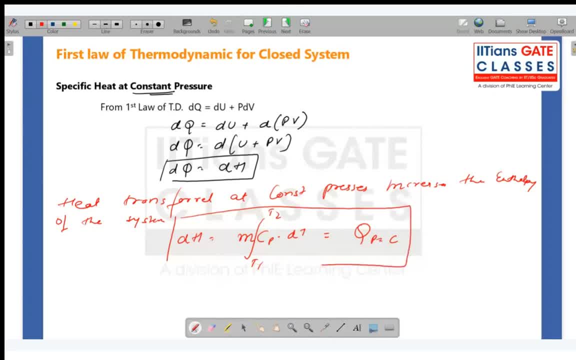 basically heat transfer at constant pressure. this much is clear. this thing we have already seen in the last class. actually, this i have defined it for you in the last class, so i am just elaborating on the last class. so i am just elaborating on the last class, so i am just 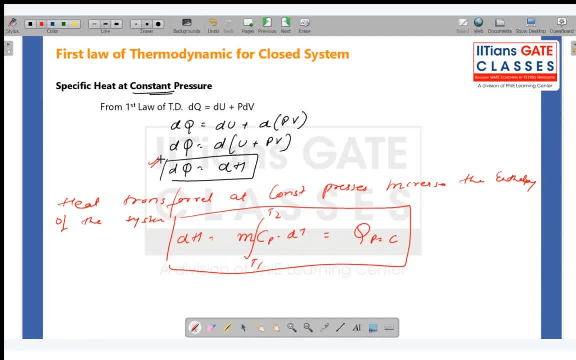 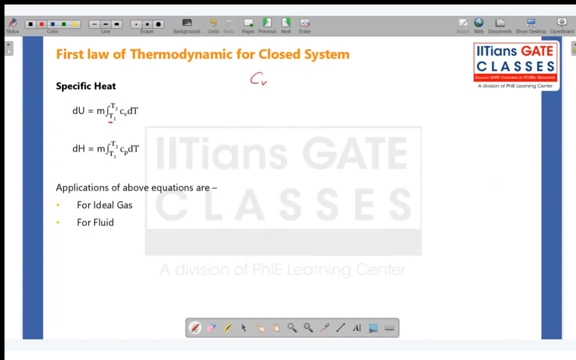 elaborating on the same concept. yes or no? is it clear? yes, no, anyone? okay now, so these are the formulas. basically, du is equals to. now, why i have written it little? i did because cv and cp they are, they are a function of temp isista. these are the formulas, basically because then we have to write v and that is because cv and 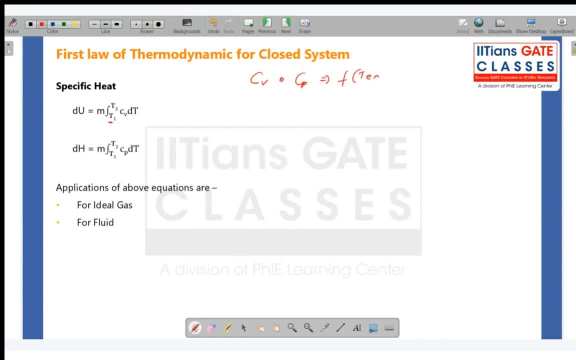 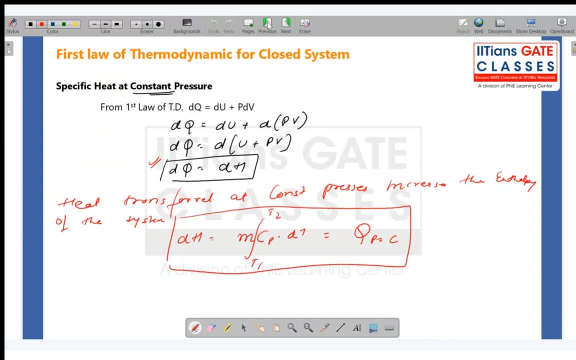 cpe they are, they are a function of temperature. so if we write this in this last class here, so logos this in cool flat. so if you go any, you please repeat: last one, which one, last one, this one, it's very simple. no, look, DH, what? what we have we done? we have assumed here, here we 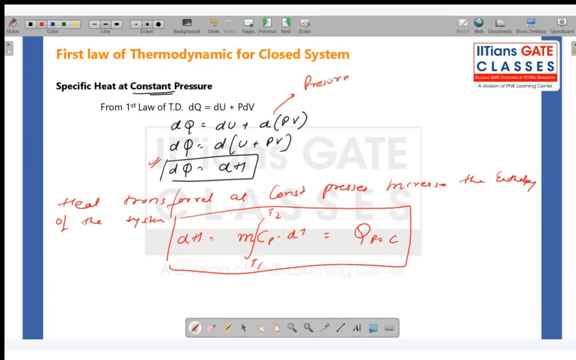 have assumed that pressure is constant. so we have taken pressure inside. okay, I know pressure spelling is wrong, but I am NOT repeating it again. pressure is constant, so so just one second. okay, so I have taken P inside, I have simplified it and I have gotten this. but this equation is only valid for constant pressure, because this: 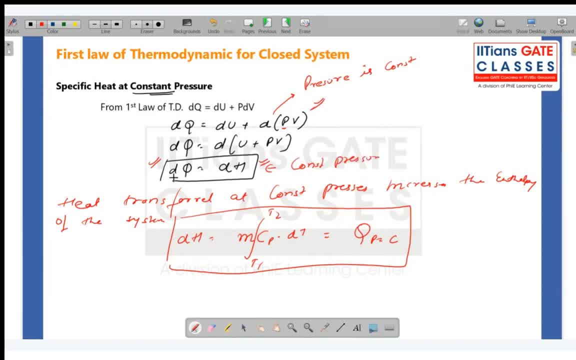 is what I have assumed in the beginning and then I have just written because I know what is dq- dq is equals to M C C. but I have just written because I know what is dq- dq is equals to M C C. but I have it in CP by P because I am using this for this pressure equation 12 specified. 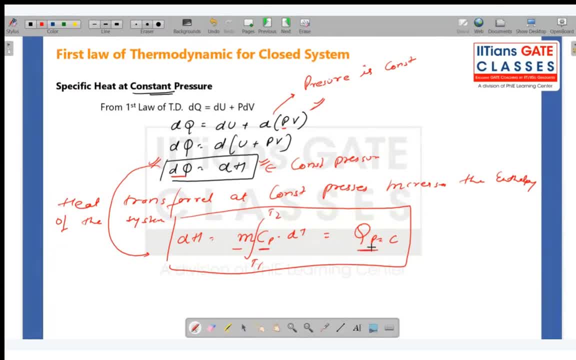 for constant pressure only. okay, and it is equals to heat transfer. okay, so basically, what you will be using is Q, dq for constant pressure is equals to d, H is equals to M, C, P, D, T. this is what you will be using, okay. okay, so what? first slide? 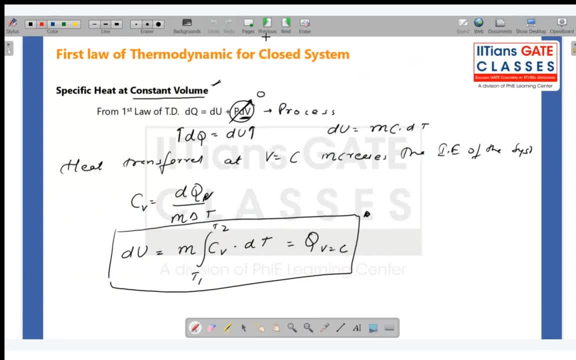 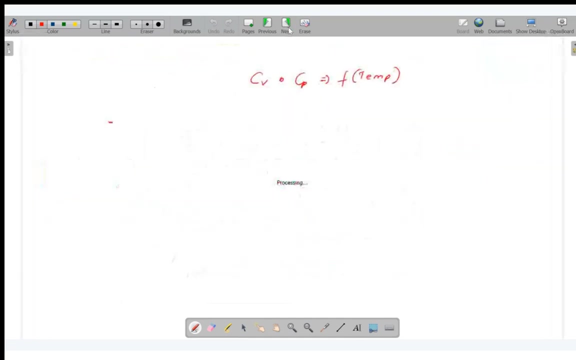 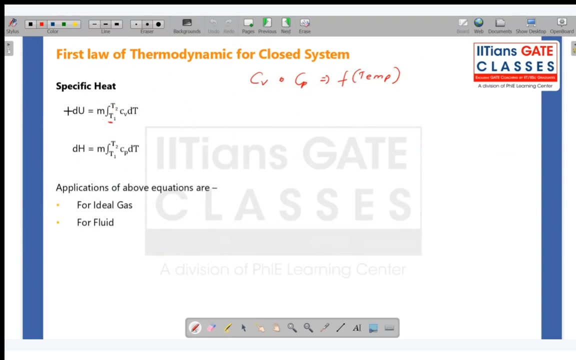 so what first slide? so what first slide? this one, okay, shivender raj, can we move ahead, or do you? are you writing something? shivender raj, can we move ahead or do you? are you writing something? something, okay. so now this is a equation that we'll be using. uh, and this is equals to heat transfer at constant. 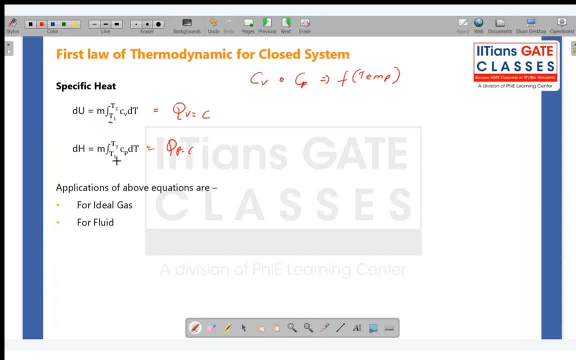 volume. this is equals to heat transfer at constant pressure. now you say, sir, why are? why are you integrating cp and cv with temperature? because basically they are a function of temperature. if you go and see your, you know uh books, what you study in your btech. so on the back of those books, 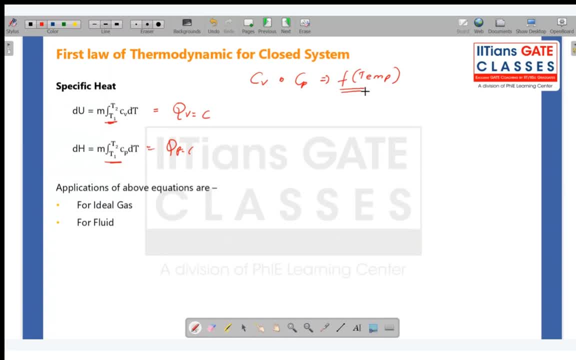 you will see cp and cv tables and you see that those basically will be changing with temperature. so you will be getting some, you know, like uh, something like this, some equation that cp is equals to, and some constant will be given to you and 1 plus at plus bt square plus c by t cube. 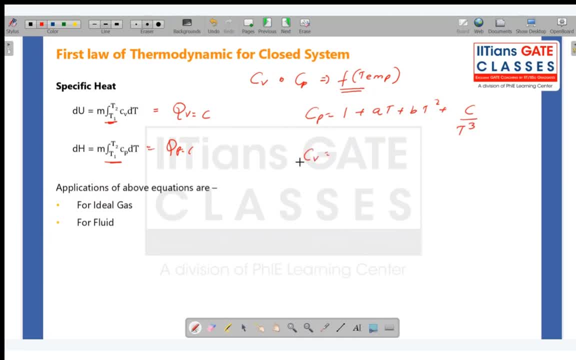 something like this: okay, but- and similarly, for cv as well, some relationship. so basically, it is saying that cp is a function of temperature and how it? how it is a function of temperature through this equation. okay, it can be linear, it can be polynomial, it can be hyperbolic, whatever relationship it could be. now, but most of 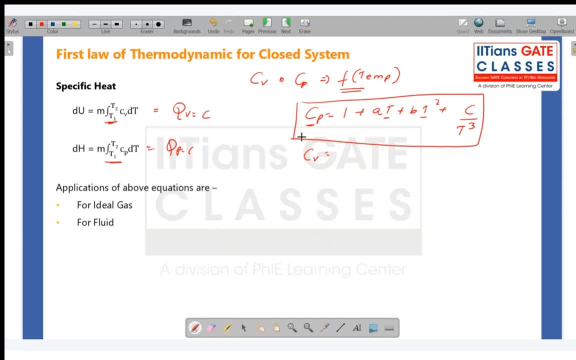 our applications, most of our problems in any competitive exam. we assume that cp and cv are not changing much with respect to temperature, so we take their average values. we take their average values, for example, for ideal gas. we can just take heat transfer. constant volume is equals to du. 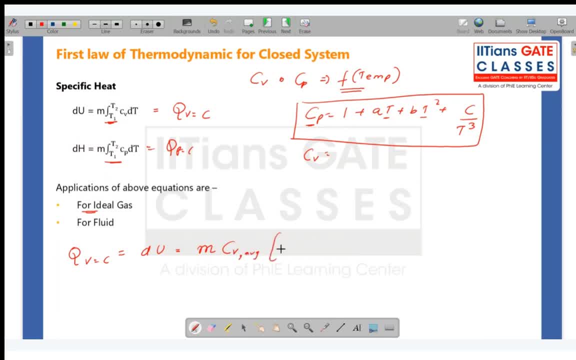 is equals to mcv average at t2 minus t1. simple. we will talk about internal energy in some time. then i'll talk about this as well. but yes, that is because of the vibration, that rotation, vibrational motion, translation motion of the molecules. so internal energy is basically what by this is coming from. internal energy, right, u is equals to: 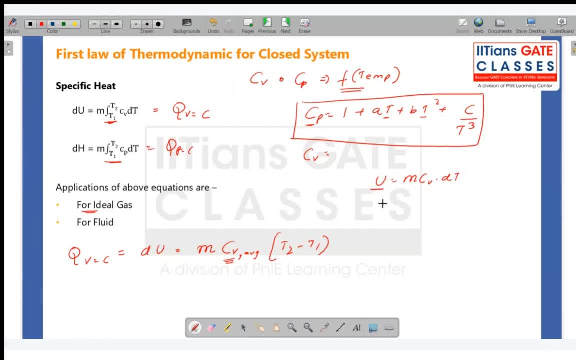 mcv dt. this is internal energy, is what it is, because of the rotational, translational and vibrational energy of the molecules. okay so, and if temperature is higher, that vibration is higher. okay so, u cp cv will change and it is identified by u. okay, so anyway. 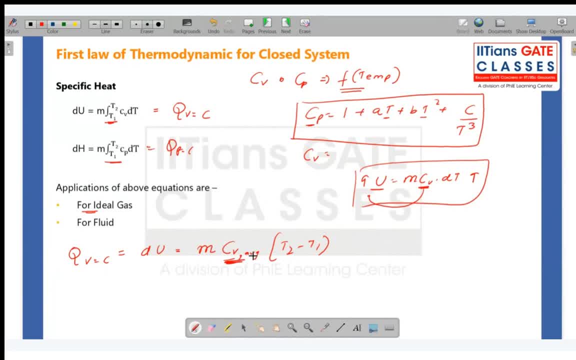 so, but you can take average values for your problem solving okay. similarly, p is equals to c, is equals to dh, is equals to mcp average t2 minus t1. so you can basically whatever values you will get in your exam for cp and cv, those are average values. for example, if you have a 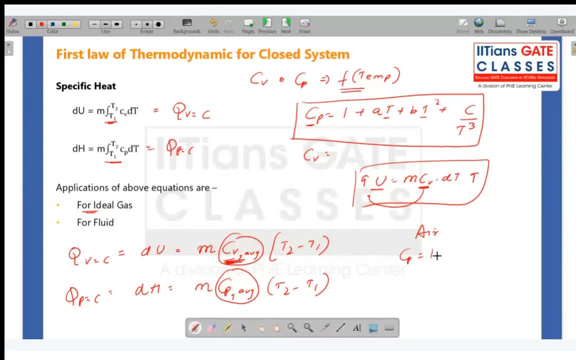 example, for air we take, cp is equals to 1.013, i think, if i am correct. okay, kilojoule per kg kelvin, cv is equals to 0.718 kilojoule per kg kelvin. but are these fixed? no, they depend on. 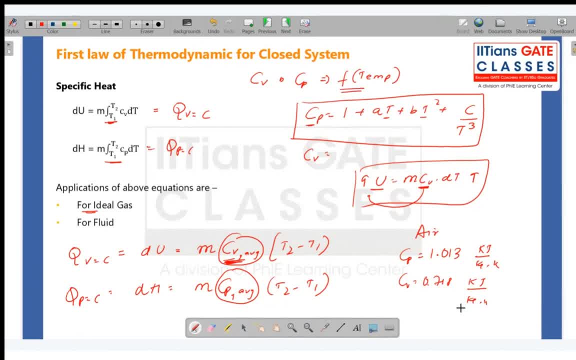 temperature, but basically the temperature that we deal with. okay, so 0.005, yeah, i think that is. uh, that is more correct. yes, but he can let me. i mean, i think it's approximate value. so what i am trying to say is that, whatever temperatures that we deal with for, 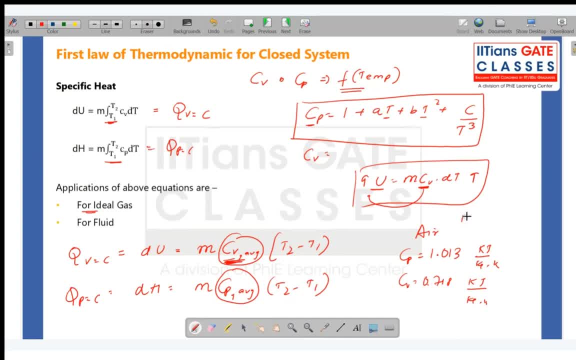 example, we usually deal around, uh, deal with around, you know, uh, let us say minus 10 to let us say minus 400, uh, plus 400 degree or 500 degree celsius. okay, so in that temperature range the values of cp and cv is not changing. 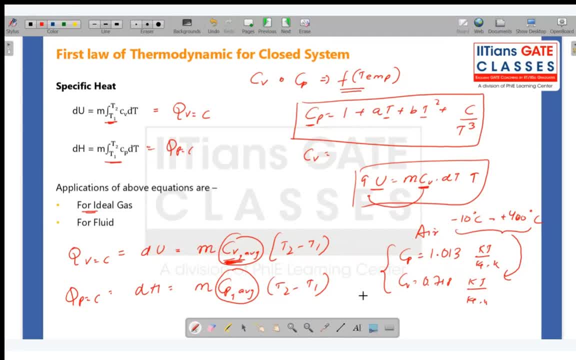 much. i mean they will be changing for sure, but not much. so we can assume that it is the average value that we can take. okay, so, and we use this continuously, we do not use the relationship. we just directly put cv and cp. is that okay? can we move ahead quickly? 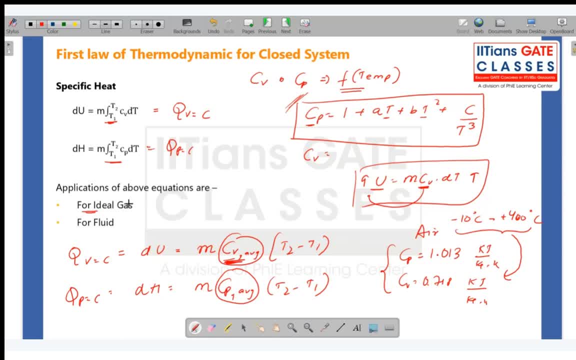 okay, so basically cp and cv values are for. it is applicable for ideal gases and for fluids and solids. fluids, liquids and solids- okay now, yeah, so basically in solids and liquid, what happens is here, so you have to use both of them. so for air we always define cv and cv, but for 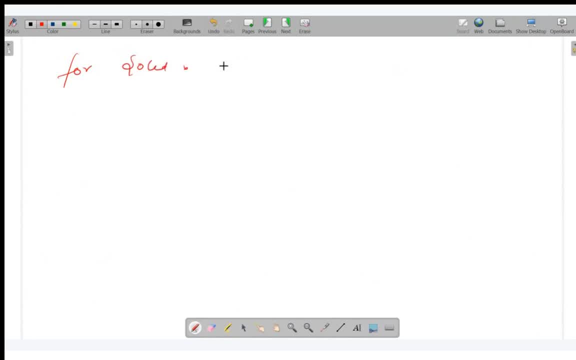 for solids and liquids. basically, what happens is, let's say h is equals to u plus pv. okay, so dh is equals to du plus pdv plus vdp. now you see, for solids, for a given pressure, for a given pressure, dv is almost zero. let's say for solids: 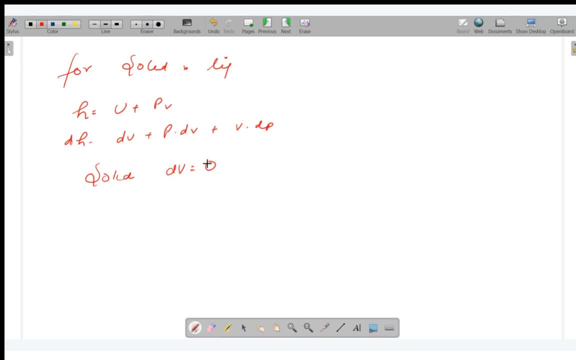 and liquid. they're incompressible. okay, you cannot compress them. gases are compressible. so for a given pressure- for if you are applying some pressure, dv is equals to zero. so these terms will be equal to zero, and also change in pressure. for a given volume, change in pressure will also be. 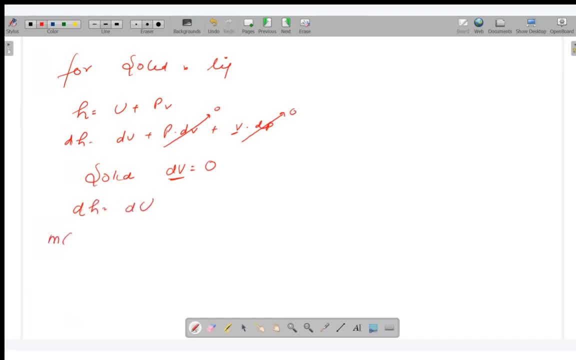 zero. so basically dh is equals to du, so mcp dt is equals to mcv dt. everything will get cancelled if mass and dt are constant. they are same. i mean, we are assuming they are same. so cp is equals to cv. in what case? in solids and liquids, but in gases again, you see, when we talk about water. so i'll just give. 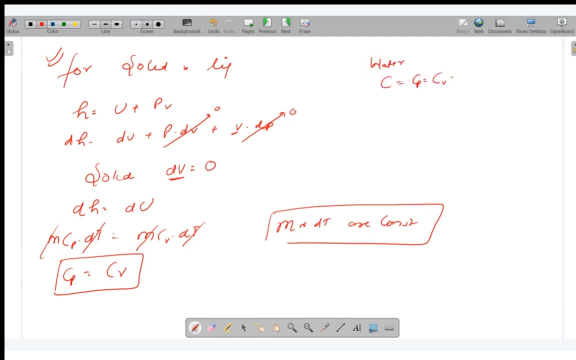 you one value c which you can use as cp cv, but it is 4.18 kilojoule per kg kelvin. similarly, if i talk about any solid- now i don't remember any values- for example, ice you can take, i don't remember the values, but basically i will give you a single value. okay, but when i talk about air or i, 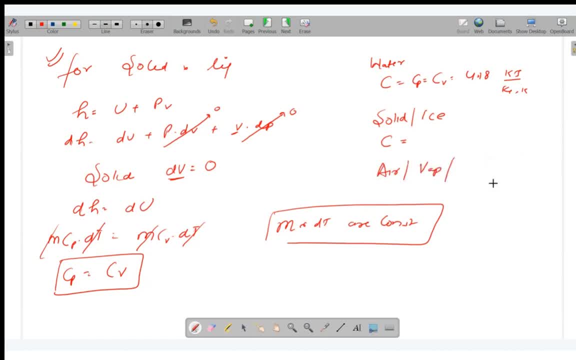 talk about vapor, or i talk about, uh, some other gas. okay, then i will give you cp, i'll give you cv. got it, because a lot of people remain confused. sir, water, the uh, they have given water. should i apply cv or cv, cp, it does not matter. dh is equals to du. you apply whatever you want. 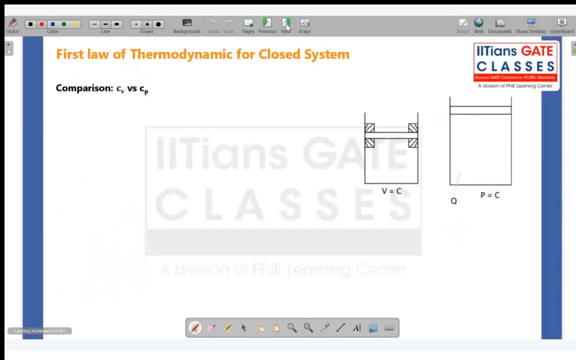 not, doesn't matter. okay, now let's compare the values of cp and cv. okay, so we have two systems. so in this also we are giving some heat and in this also we are giving some heat. so we have: one is constant volume process, one is constant pressure. 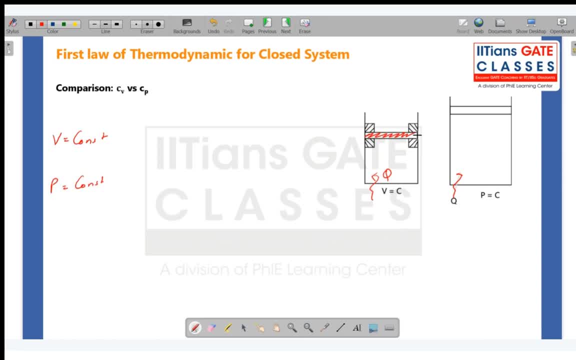 so here our piston is fixed. so volume will remain constant. volume will remain constant. now i am giving some heat, and you know, dq is equals to du plus dw. so we have du, we have dw. okay, now i know, for constant volume, dw is zero. this is what i know. 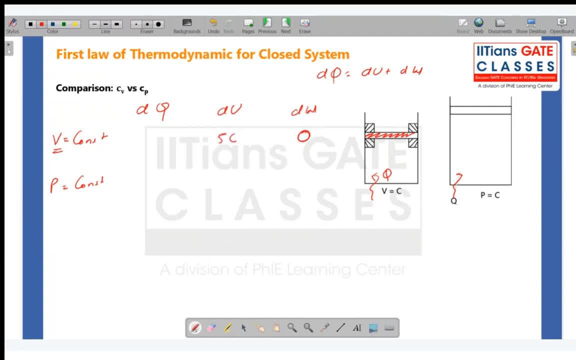 also, i want same internal energy change. for example, i want fuel 50 or 50.. Okay, So now you see here, if I am for this 50 internal energy change, I only need to give 50 heat. So this will be 50, because everything is converted into DU by for constant. 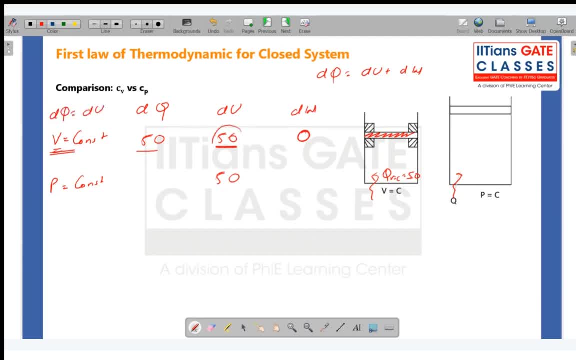 volume. DQ is equals to DU. So for this 50 change in internal energy I just need to give 50 heat units of heat. But in order to get this 50, if I give here 50, then that means work will be zero. But in constant pressure work is non-zero. So let us say: your work. 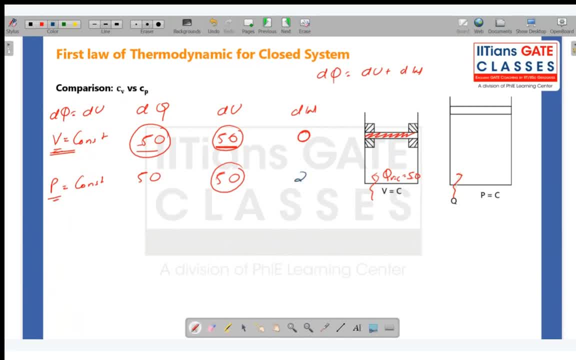 is, let us say, 20, whatever some value, some non-zero value, Okay, So basically, in this time in constant pressure, you would be needing 50.. You would be needing 70 heat transfer. When you put 70 constant pressure, then change. 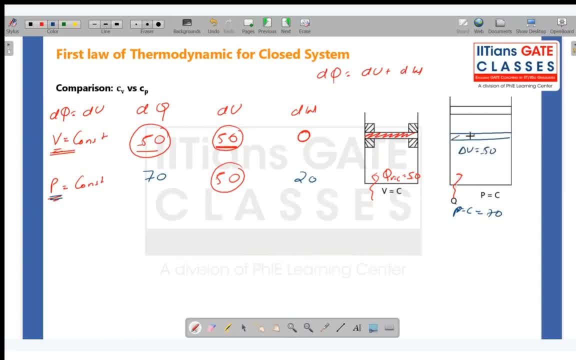 in internal energy will be 50 and the piston has moved. You see, piston has moved from here to here. So the work transfer that is involved is what? PV2 minus V1 is basically 20.. These are some random values I am giving, but I just want to tell you that this is a constant. 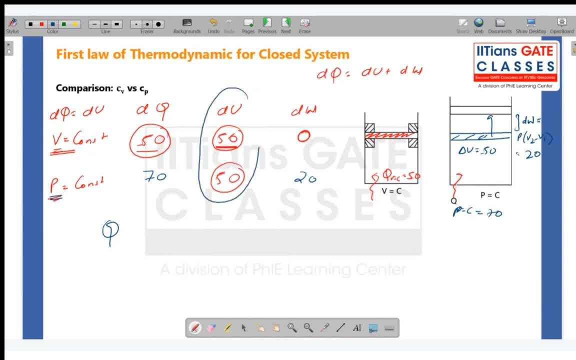 pressure. This is a constant pressure. This is a constant heat transfer. I just want to tell you that always for same change in internal energy, you have to give more heat transfer for constant pressure than constant volume. So mCPDT will be greater than mCVDT. And if 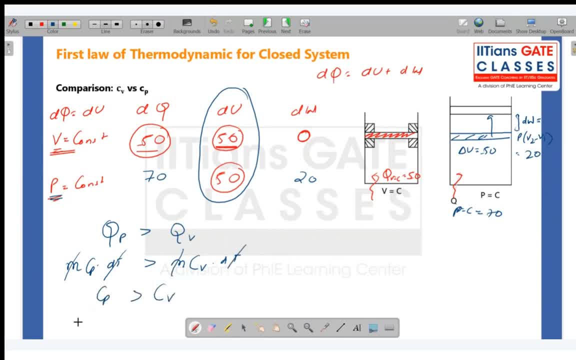 for same mass transfer and delta T, CP is always greater than CV And the ratio between them is called as gamma. Okay, Yeah, Okay, So that is a constant pressure. So then I have to give more heat transfer, called as gamma. So I always know gamma is always greater than 1 because CP is greater than CB. 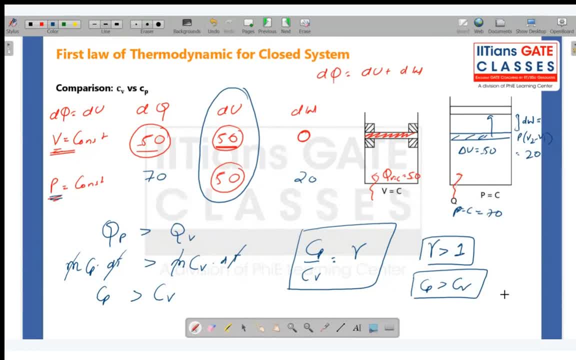 always. No doubt about it. No doubt about it. Okay, Is it clear? Should we move ahead? It changes with other properties, but okay, just wait, Devendra, We will discuss this, Okay. So basically, just briefly, I'll tell you for ideal gas. 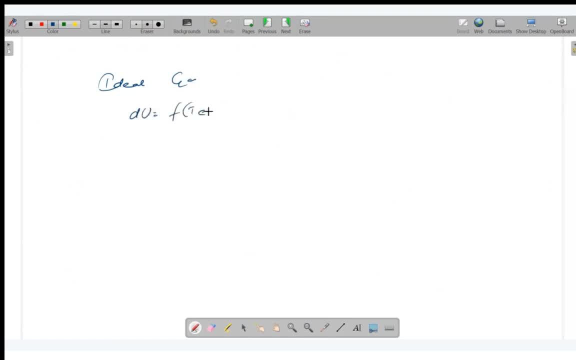 ideal gas. internal energy is a function of temperature only. Okay, This is also called a Joule's law. It is also called a Joule's law only for temperature, because internal energy is basically- again, I am deviating from the topic. I'll explain this later. Okay, Don't worry about. 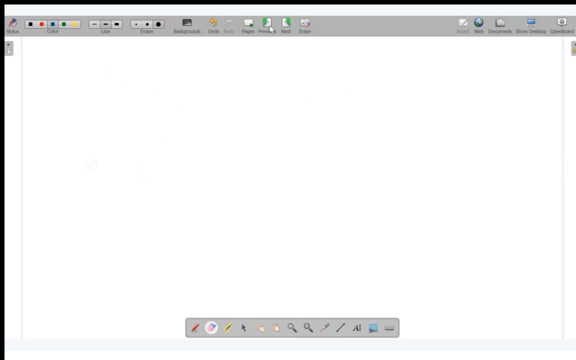 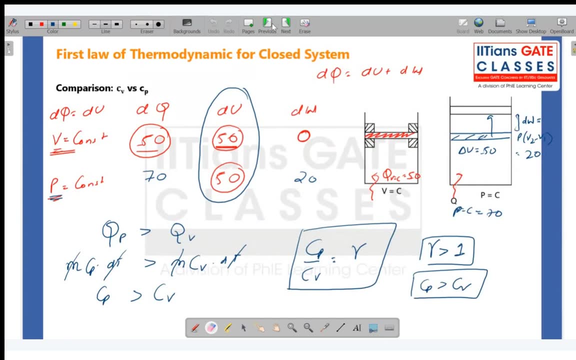 it. I'll explain it in a while. Today, only I'll explain: Yes, Yes, Yes, Yes, Okay. So let's not deviate, because if I deviate, I will have to explain again and again. Okay, So this much is clear, or not? First of all, you tell me. 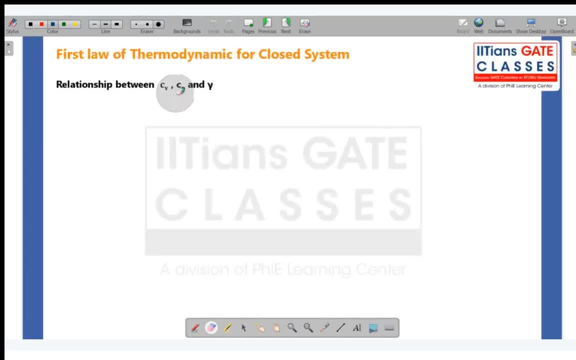 Okay Now. so what is the relationship between CP, CV and C gamma? Okay Now. you see, H is equals to U plus PV. Now what is the ideal gas equation? Ideal gas equation: PV is equals to MRT. So I can write. 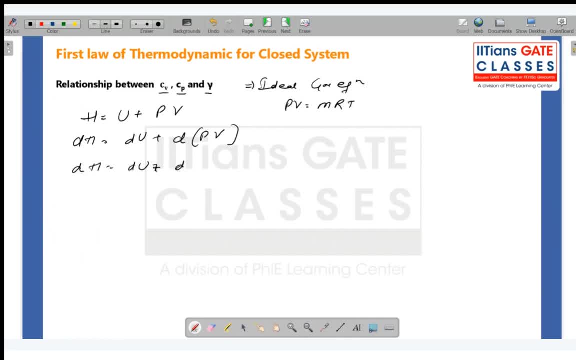 DH is equals to DU plus DMRT. So now I can expand this: CP, DT, MCV, DT plus MRDT. I can cancel this. So CP minus CV is equals to R, CP minus CV. So this is the relationship between CP and CV. Now, CP minus CV. Okay, CP minus CV is equals to MRT. 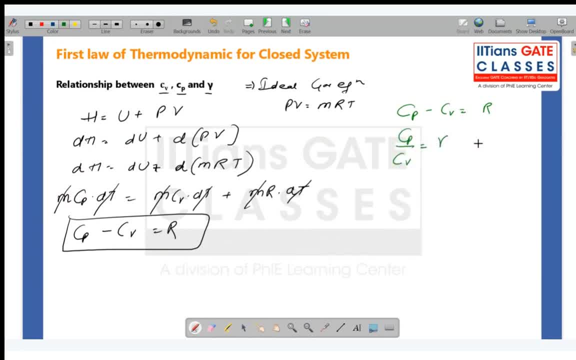 And we have. we also know that CP by CV is equals to gamma. So can I say: CP is equals to gamma CV And let me substitute it here. So gamma CV minus CV is equals to R CV. gamma minus one is equals to R. CV is equals to R upon gamma minus one. Okay, And now let 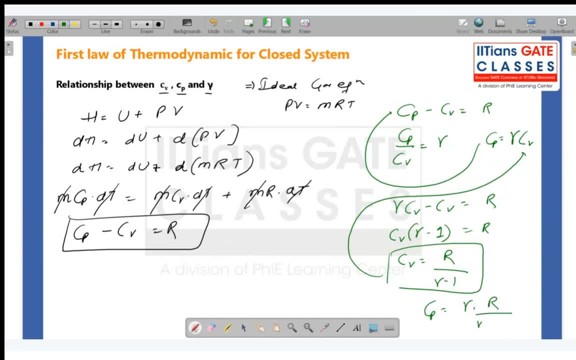 me substitute it here. So CP is equals to gamma R upon gamma minus one. Okay, So very rarely we use these two equations. The most we use is basically these two equations. This is very frequently used, very, very frequently used. 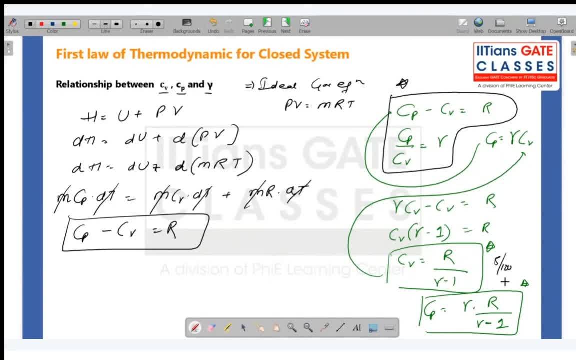 This. I think, let us say, maybe five times out of a hundred. we use this very rarely And anyway, it came from here itself. So basically, if you are using this, you are fine. Okay, Clear, Let us know quickly. Just be with me, answer quickly so that we can cover enough, Okay. 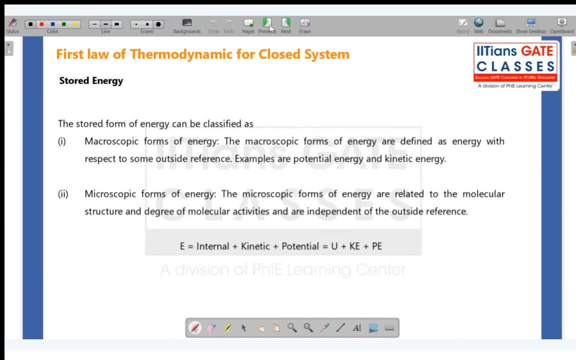 Hello Now. so we have seen what I, if you remember that thing- So energy is basically stored- and terms that He'd. we have discussed work We have discussed in this. We have Machines, macroscopic and microscopic, but we have kinetic energy, potential energy, internal energy and 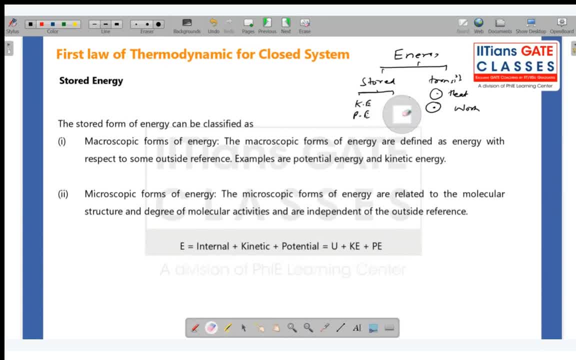 chemical energy. so this is what chemical energy we are not going to discuss. and also, i have already told you, kinetic and potential energy is. basically we all know kinetic energy is what? because of the velocity, half mv square. what is potential energy, mgz. okay, so our focus is internal energy. now just i have written it here- the stored energy. 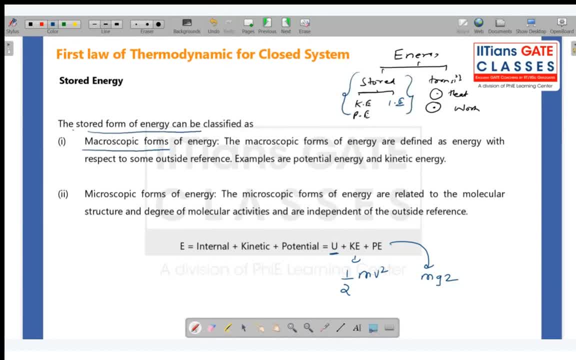 this portion can be classified as macroscopic form. so macroscopic form of energy are defined as the energy with respect to some outside reference. okay, so you see, potential energy is basically always potential energy is defined with respect to a reference. so if you take some reference, you see this is z1, this is z2 or whatever. 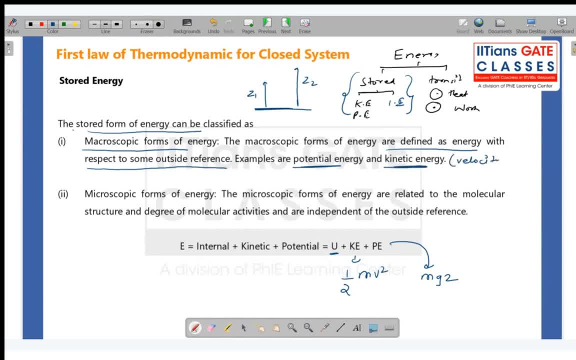 and also kinetic energy. that means velocity is always defined with respect to something. okay, there is no absolute velocity, okay, so you define with respect to this body. this body has some velocity, okay, so this basically depends on outside references. that's why they are called as macroscopic form. microscopic is basically: that depends only on the system, only on the system. 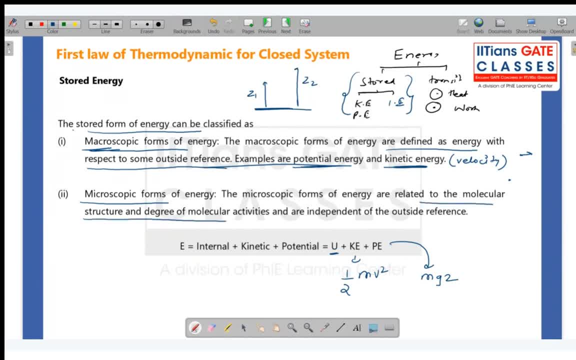 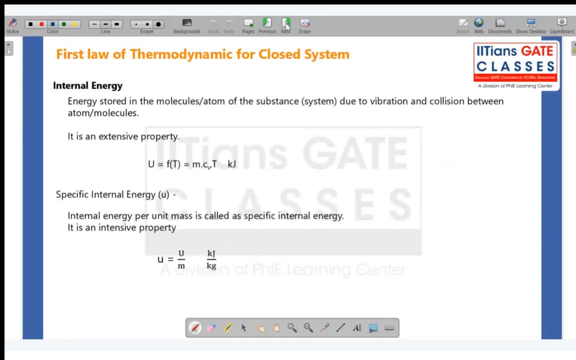 so basically related to the molecular structure and degree of molecular activities and are independent of outside reference. so these are based. internal energy is a microscopic energy and total energy is basically in totally stored energy is internal energy, kinetic energy and potential energy. okay, now what is internal energy? so energy. 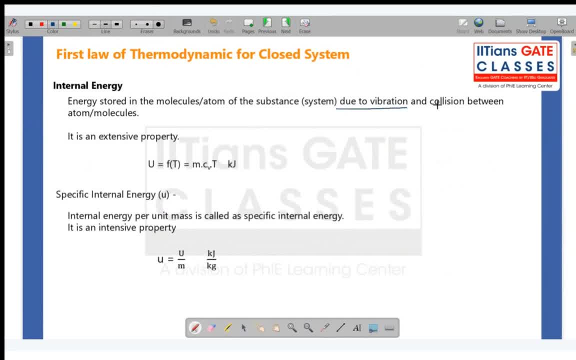 is stored in the molecules of the substance due to vibration and collision between the atoms and molecules. that's why i was not explaining it there, because it was anyway coming, okay. so energy stored in the molecules due to the vibration and collision. now why this vibration in molecules happens? it happens because of the temperatures. so basically, 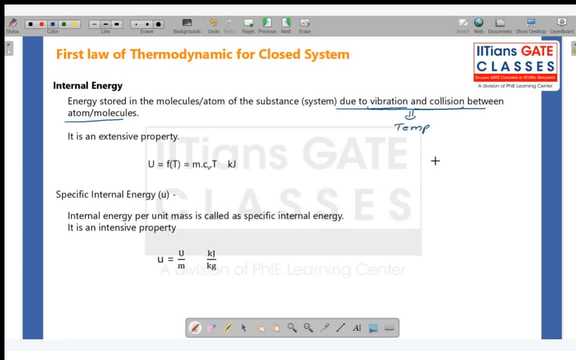 you see, molecules have some molecules have some translation. okay, some they will move from one place to, so that is called as translation motion. they can also have some rotation with respect to each other. okay, so they can rotate. so rotation or rotation, or they also have vibration with respect to each other. so because 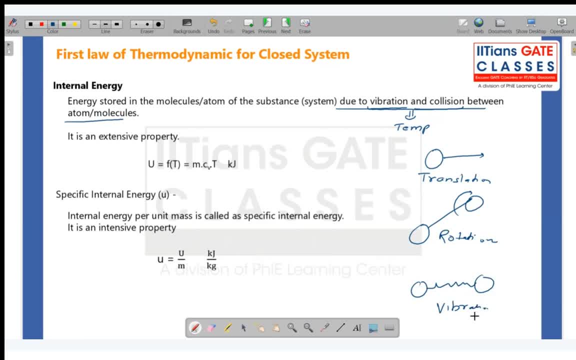 of this. higher the temperature, higher these motions, okay, higher the temperature, higher the translation, higher the rotation, higher the vibration. so the energy that is because of this is called as internal energy. so basically the energy stored by the. okay, is it just for you or everyone else? can everyone else hear me like? am i clear to everyone? 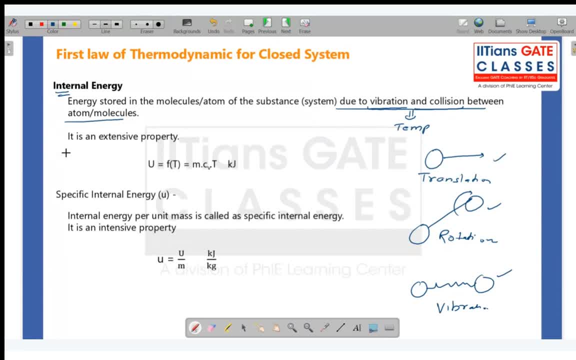 okay, okay. so, ravi teja, i think it's from your side, okay. so, whatever energy is because of the what, whatever? okay, thank you, thank you, thank you everyone. okay, so, whatever energy is possessed by the molecules, so if some mass is there, mass will have what molecules will. 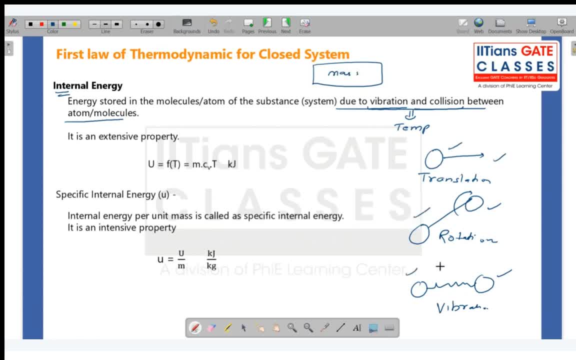 have molecules will have some translation energy, rotational energy, vibration energy. if you give more heat, more temperature, that means higher energy, higher translation, higher rotation, higher vibration. but the energy possessed or stored by this mass is called as- and okay, let me write it one more time- energy possessed by this mass due to temperature, due to temperature, because this mass. 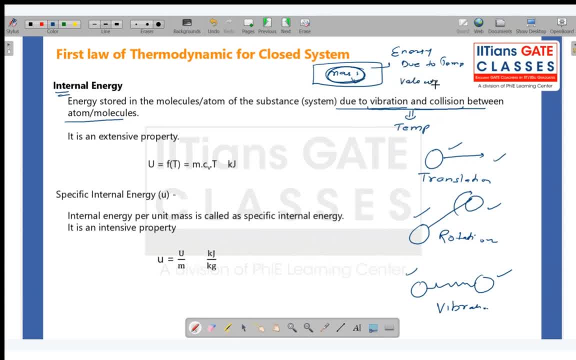 will have some energy, due to velocity as well, that is kinetic energy. due to position as well- that is potential energy. but due to temperature, the energy that is possessed is called as internal energy. is it clear to everyone quickly? okay, so it is internal energy is an extensive property. I have already 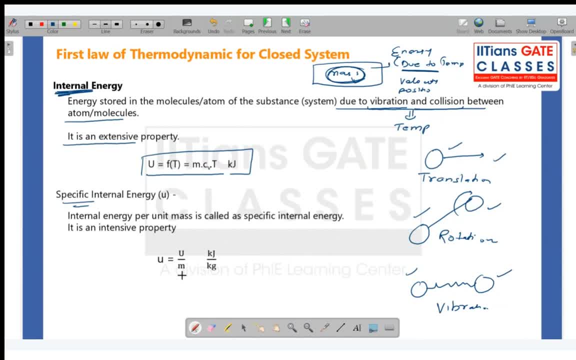 explained this, and a specific internal energy is basically internal energy divided by mass, so it's a intensive property. all these things we have discussed in the first class. I am just repeating it again so that it will. you will get some revision as well, okay, and I have explained you here that there is. 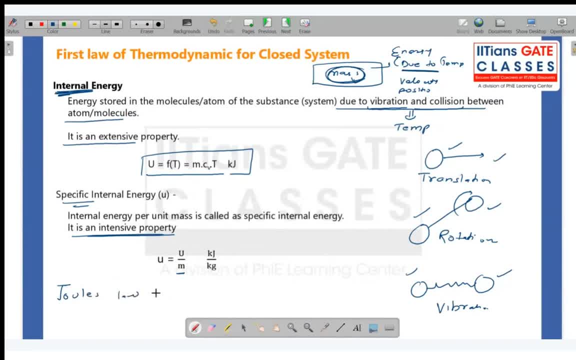 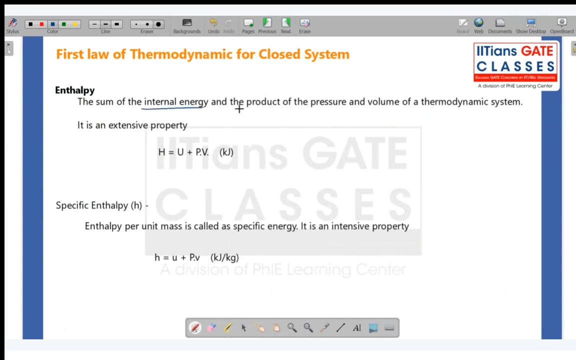 a Joule's law. this basically tells you that internal energy for a ideal gas is a function of temperature only. so this can be objective. objective question as well. internal energy for ideal gas is a function of temperature only. okay, now what is enthalpy? the sum of internal energy and the product of the pressure. 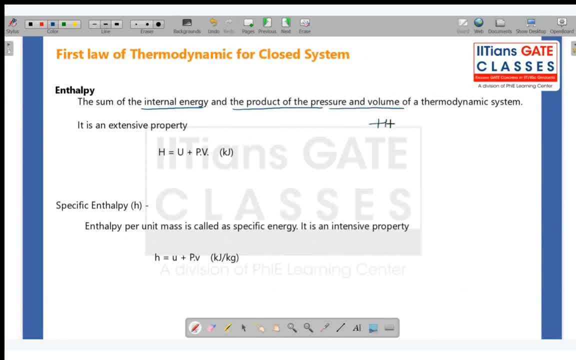 and volume of a thermodynamic system is called, so enthalpy is basically more of a convenient term. so we have this term we use very frequently, and this is basically determined by the energy processing exercised by open system. now, right now, I am NOT explaining this. I will. 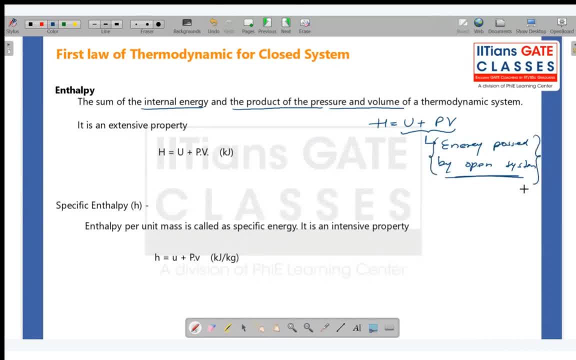 today come to open system and again I will explain this, okay, because if I approximate here it will take some time and I have do any varyn later on, so I not explaining right now, but just remember: u plus pv is the energy possessed. i know this spelling is. 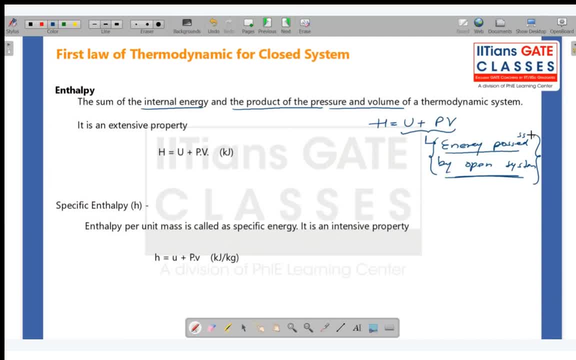 wrong. okay, possessed by open system flow. work at open. look, sanjeev, wait, that's what i am saying. wait, we will come to that. whatever i am saying, just try to, because we are on closed system, you see. so don't worry about this, we will come to open system. we will discuss this okay now, but what i am? 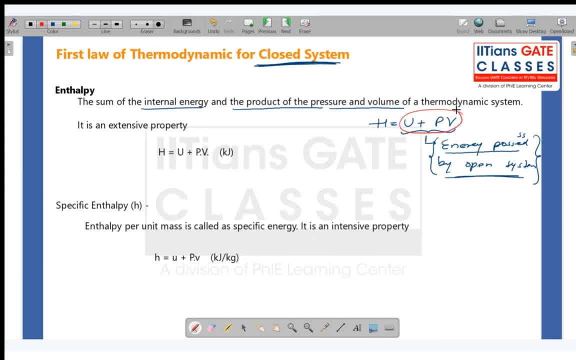 trying to say is: this is one term that we use very frequently and just for convenience, we have given it a name h, and h is called as enthalpy. now, enthalpy is an extensive property. if you divide it by mass, then it will be specific enthalpy and it is an intensive property. okay, so again, this i. 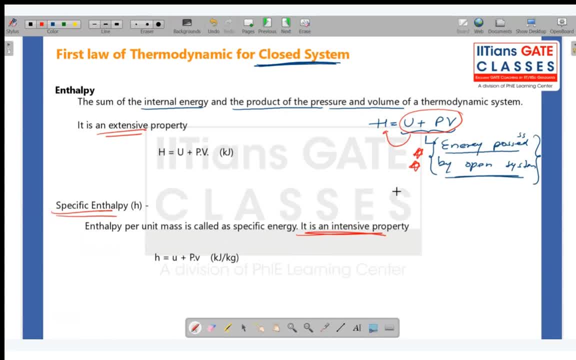 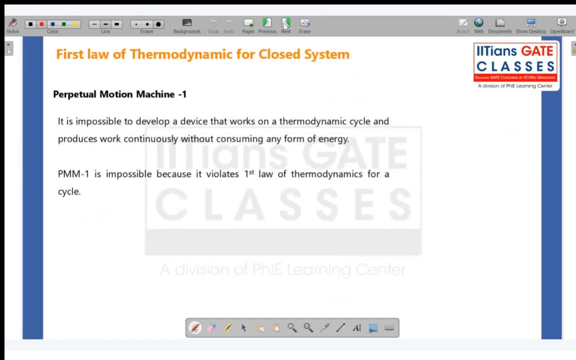 will explain in some time, do not worry about it. okay, i hope internal energy is clear. enthalpy will be clear in some time, but right now, just understand: h is equals to u plus pv. okay, can we move ahead quickly? okay, let's go now. perpetual motion machine of kind first. so it says it is impossible to develop a. 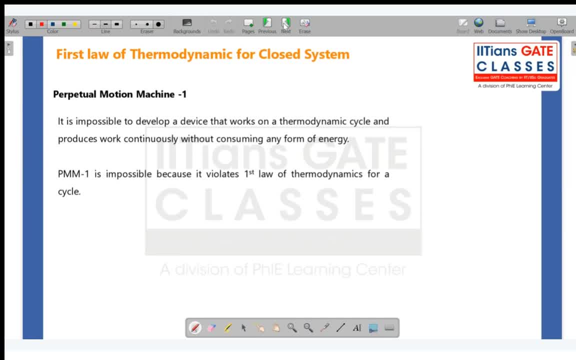 device that works on a thermodynamic cycle and produces work continuously without consuming any form of energy. so basically it is saying you have a device. let us say you have a device and it works on a thermodynamic cycle and it produces work continuously. that means it is. 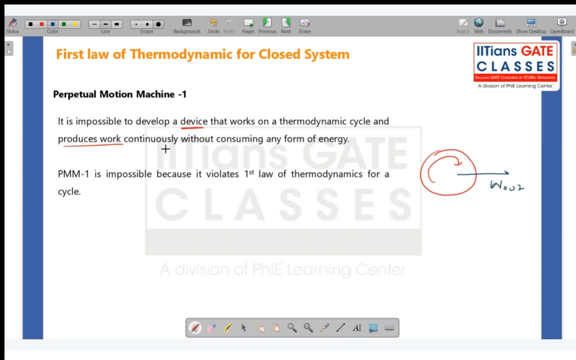 giving you work, continuously, work, output without consuming any form of energy. that means it is not interacting with anything, nothing is coming in, but work is going out. but if you see, according to first law of thermodynamics, for a cycle q12 will be equal to w12. right, that means i am saying i am not giving it anything. 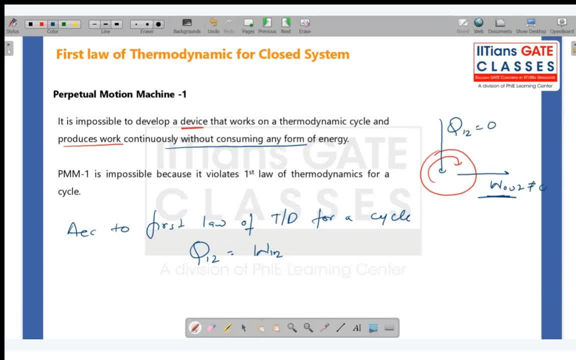 that means q12 is zero and i am saying work output is not zero. it is giving me work output. but first law is saying: if this is zero, then this must be zero. so that is the first law. means this device, whatever device this is, it is not possible because it is. 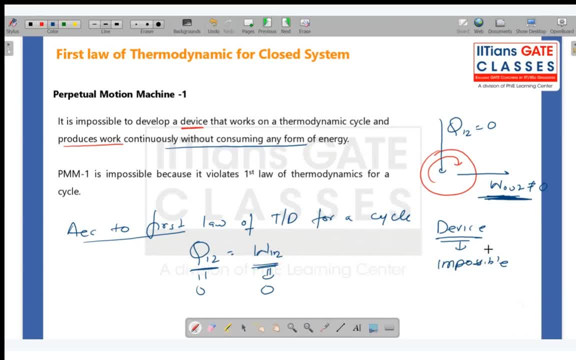 violating first law of thermodynamics. and if this device is possible somehow, it is called as pmm1 perpetual motion machine. i hope you all understand what is perpetual, perpetual. can anyone tell me what is the meaning of perfection, like in physical? what is the perpetual meaning, like in? 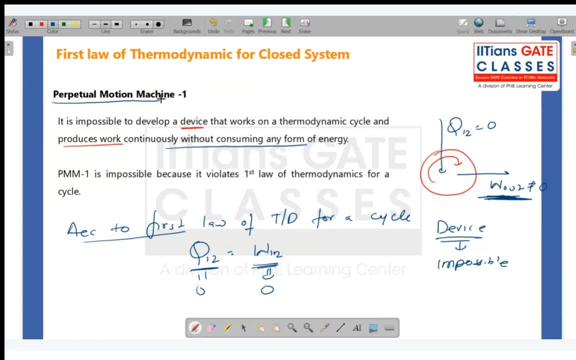 general continuous, yeah, continuous or always, or whatever you want to call it. so basically, a machine that can always be in motion. it does not matter you are giving some heat or not, but it's always in motion. okay, so this is not possible. this is because it is violating the first law. this machine is saying: 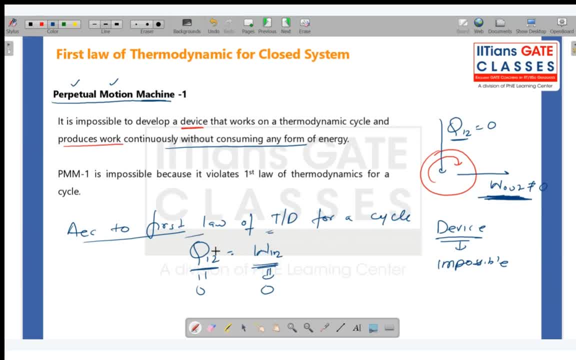 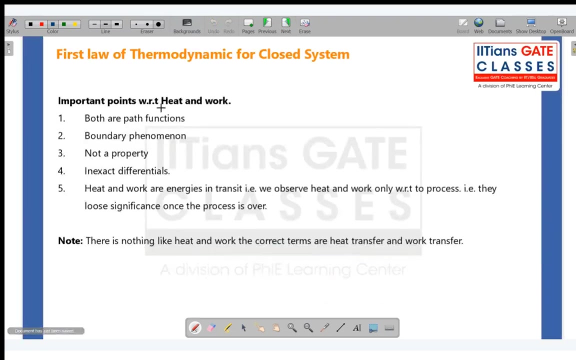 that work output you are getting, but you are not giving anything. but first law is saying: you have to give work, then only you have to give heat, then only you will get work. okay, clear, yes, no, okay, now, very, uh, some important points. so heat and work. okay, so heat and. 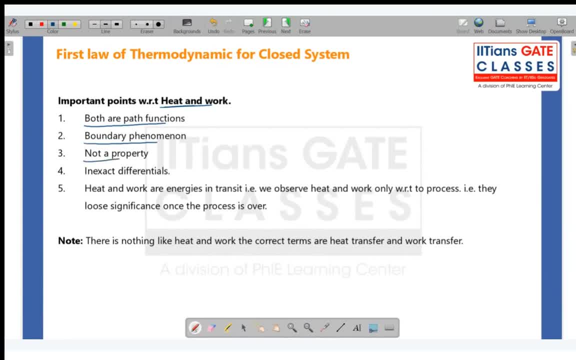 work, both are path function, they both are boundary phenomena, they are not a property, inexact, differential, and they are energy in transit. okay, and there is nothing like heat and work. it's always heat transfer or work transfer. we- i mean he- there is no absolute value of work or heat. 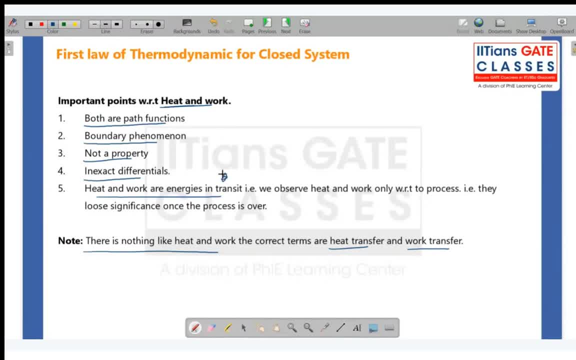 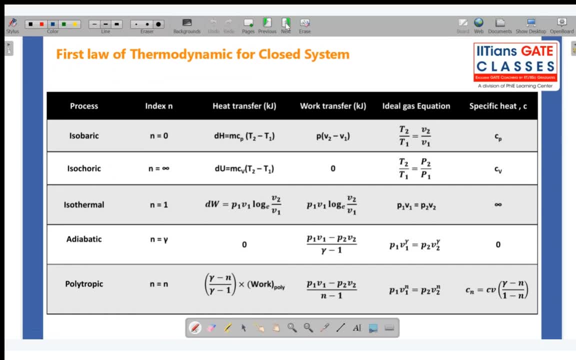 okay, it's always because it's an energy in transit. so we always say heat transfer or work transfer, always okay now. so i have summarized everything for you. this is a idle gas index. okay, we discuss about k value, right? so this is that value: isobaric. so we have everything in terms of you see, uh, if you 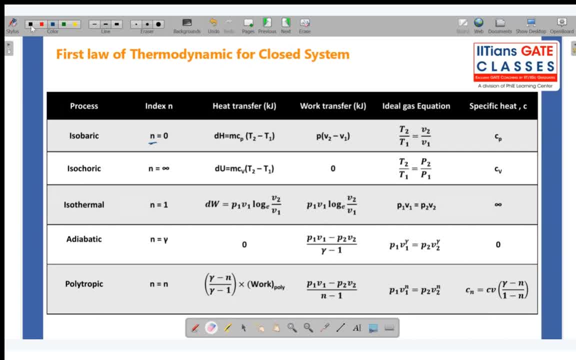 remember, we have everything in terms of you see, if you remember, we have everything in terms of you see, uh, if you remember just one second, we defined everything in terms of pvk, or n is equals to constant. so n value is this: n is equals to zero for constant volume. it's infinite, isothermal, it's one. 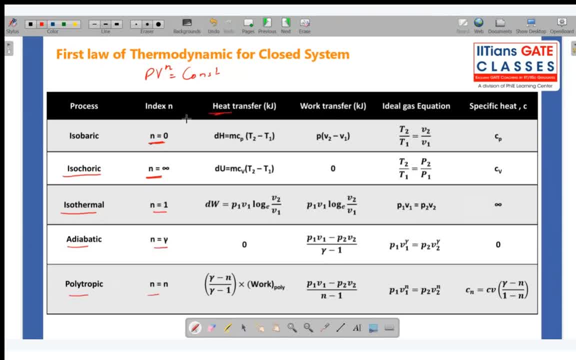 adiabatic, it's gamma, polytropic it's m. heat transfer. isobaric- we have just discussed this today- is equals to dh. isochoric du isobaric- we have just discussed this today- is equals to dh. isochoric du isothermal, we have discussed by dq, is equals to du plus dw. 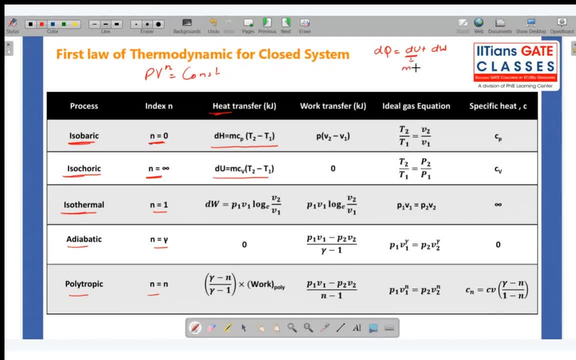 now it is isothermal. so this is what mcdt isothermal means. this is zero. that means this is zero. so dq is equals to dw, already discussed in the last class. okay, so here heat transfer is equals to work transfer, adiabatic heat transfer is zero and polytropic is zero. we very rarely use this so i have not defined it. 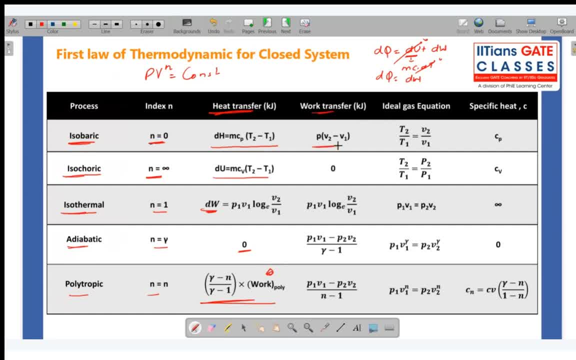 so i have not defined this. okay, work transfer: isobaric pv2 minus v1: this is zero. this is work transfer. this everything we have defined. ideal gas equation also: we have defined everything we have discussed. i have just summarized you because i know i have covered so many formulas, so at some 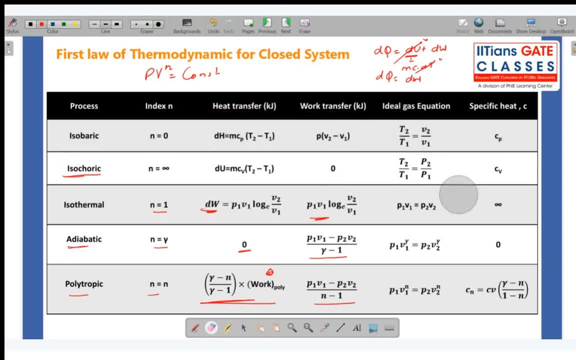 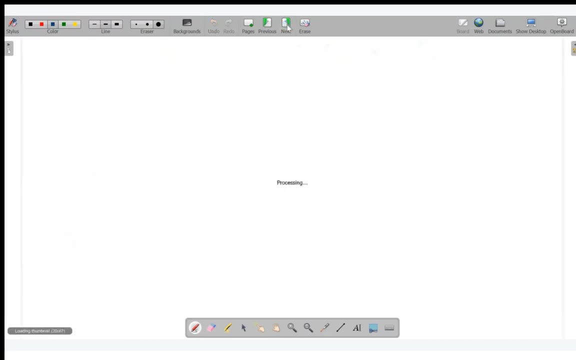 point of time you will get confused. so you can refer to this table and maybe it will clarify a few things for you. got it? nothing new i am teaching here. it's just the same thing we have discussed in now, yes, no, okay, very nice, let's move ahead. let's move ahead. so till now, what we were discussing is: 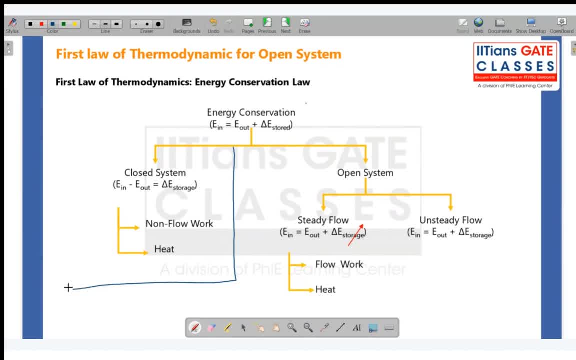 this portion of the first law of thermodynamic closed system. now we will move ahead to open system. now, in open system, there are two classifications: steady flow and unsteady flow. i think i already explained what is steady flow and what is unsteady flow. okay, we will discuss again. but anyway, i think i hope i have discussed this. so steady flow is: 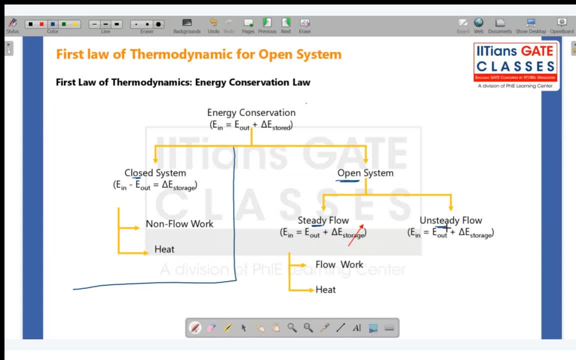 where mass flow rate in is equals to mass flow out, energy flow rate in is equals to energy flow rate out and there is nothing is stored into the system but in unsteady flow. so steady flow, this is zero, but in unsteady flow, this is not non-zero. okay, so we will discuss this. 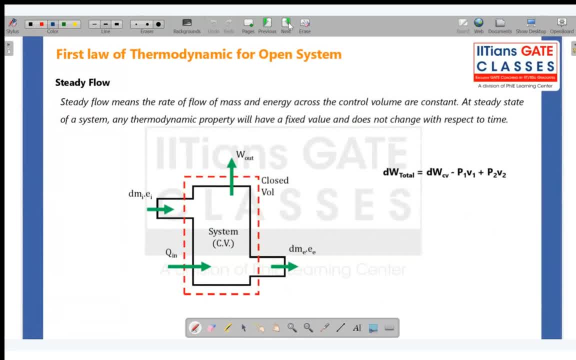 now let's start with steady flow. so, as i said, steady flow means rate of work rate, rate of flow of mass and energy across the control volume are constant. it is simply telling you that whatever mass is going in, or what is the mass flow rate in is equals to mass flow rate out. okay, so let us say i will drop this. 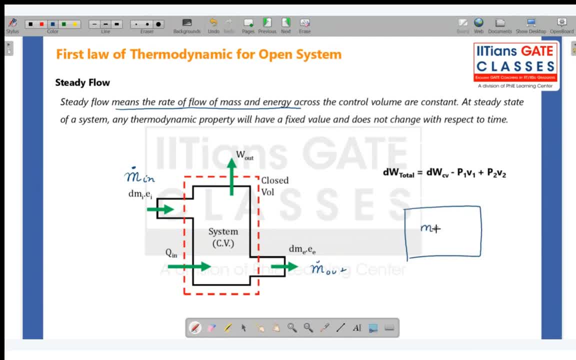 I'm just explaining this and then I'll rub this. If inside mass of this system is, let us say, 100 kg- OK, now I am sending in m dot in is equals to 10 kg per second And with the same rate I am taking it out, 10 kg per second. 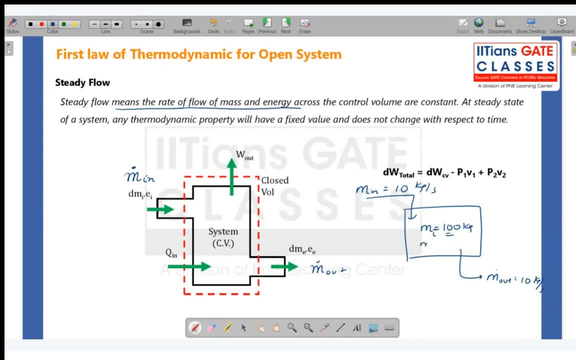 So if the initial is 100 kg, what will be final Mass inside the system? quickly, Yes, So basically, finally, there will not be any change because whatever is coming in is same thing is going out. So basically The change of mass inside the system or storage. 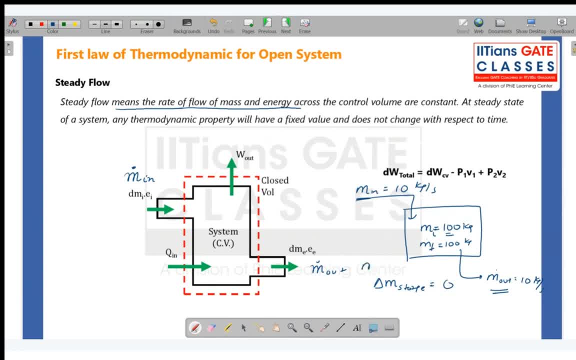 Is equals to zero. OK, Because m dot in is equals to m dot out. OK, In fact, let me write this here because I will drop this figure. So M dot in. This is the condition for a city flow. OK. 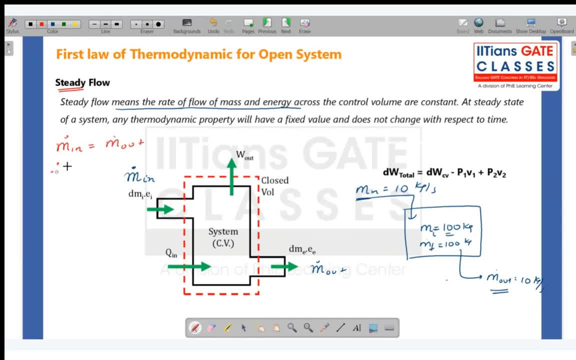 I am not making it up myself- And therefore change of mass inside the system storage is equals to zero. Same thing happens with energy. So energy be whatever is In is equals to energy out And therefore change in energy inside the system will be zero. 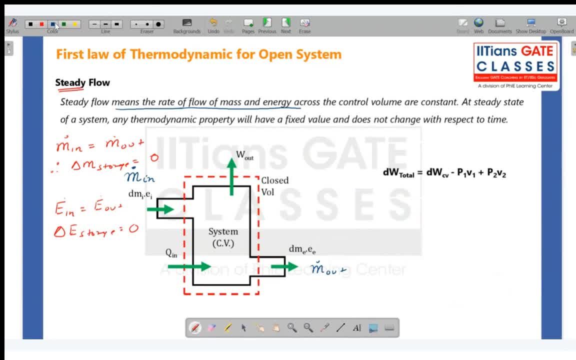 OK, Now What is happening here? You see, look, mass is flowing inside, Some mass is coming from outside, Some mass is coming from here, And this system has already some mass. You see, this system is already filled with some mass. 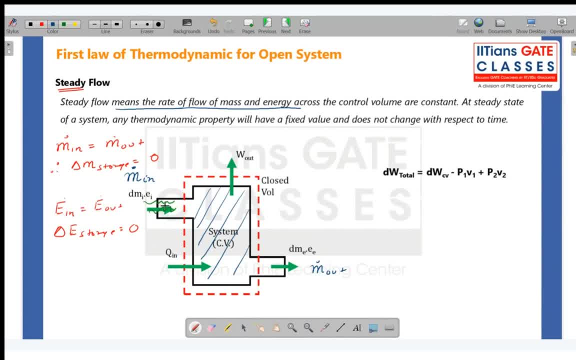 OK, Now, when this green mass is coming from outside, it is going to push. See, I have mass still here. OK, This is completely filled. I have already filled this mass and it is also filled here. Now, then this new mass will come in. 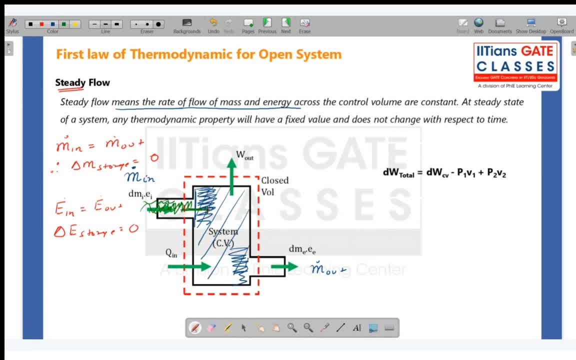 So it will try to push this mass a little bit inside. Yes, It will try to come in Right, So it will push the boundary Of that blue mass which is already inside. OK, Now, when it is pushing the boundary, that means when boundary is changing, that means what? 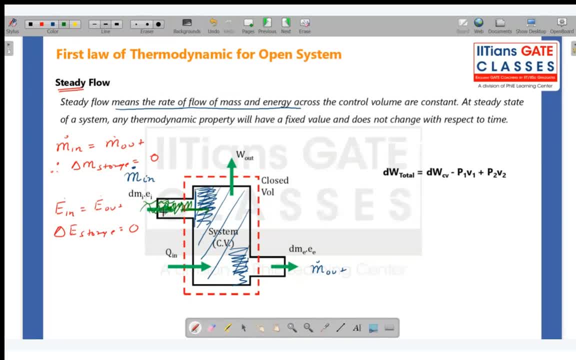 When boundary, yes, work is happening. So when this mass is coming in, it is pushing the boundary inside, So it is a compression work. It is type of a compression work. It is compressing the mass inside, So that is called as negative. 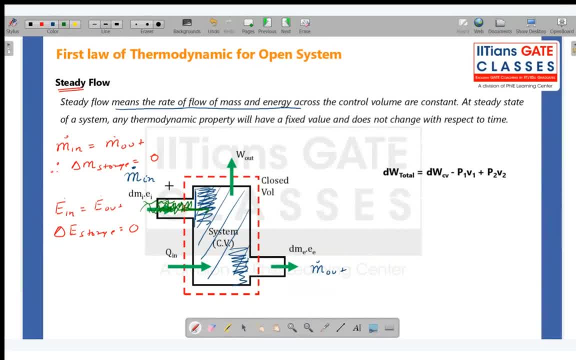 If you are pushing the boundary inside, It is negative. So the work that it is doing to come inside is minus P1 V1.. So this is the work Done by mass entering At the boundary. OK, Now, Now, what is happening now? 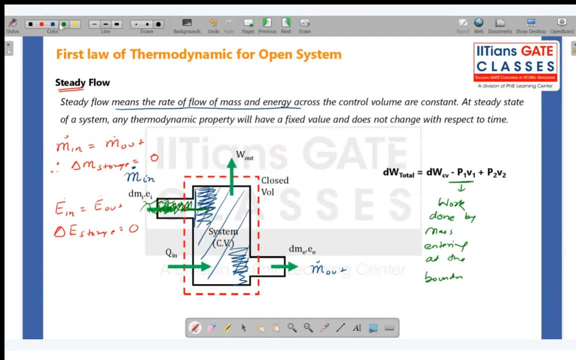 There is some mass here, You see. Uh, let me look, it is here. We have a boundary, right here We have a boundary. OK, now this blue mass is trying to go out. It will try to flow out. When it is trying to flow out, it will try to push the boundary outside. 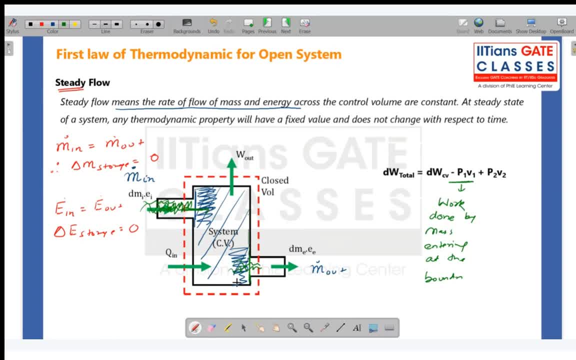 It will try to push the boundary outside. So if it is pushing the boundary outside, volume will increase and it is kind of an expansion work. Expansion work is what Positive? okay, it is work done by the system on the boundary or on the surrounding, by. if this 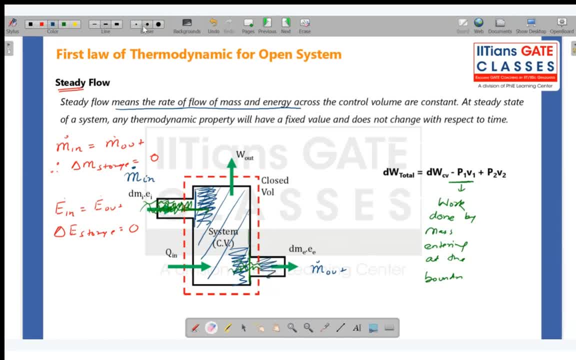 is my boundary, so outside anything is just one second. if this is my system inside, then outside anything. i am just, you know, running out of colors. so outside anything is what surrounding. so this: when this mass is going out, it is pushing the boundary outside towards the surrounding. 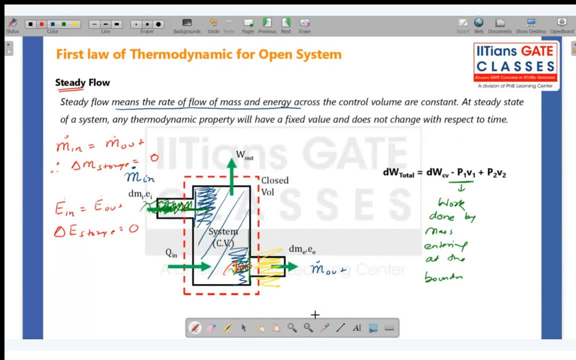 so it is work done by the system on the surrounding. and what was this? this was work done by the surrounding on the system or work done by the mass on the system. okay, so this mass, when it is going out, it is going to push the boundary outside in this kind of expansion work and this 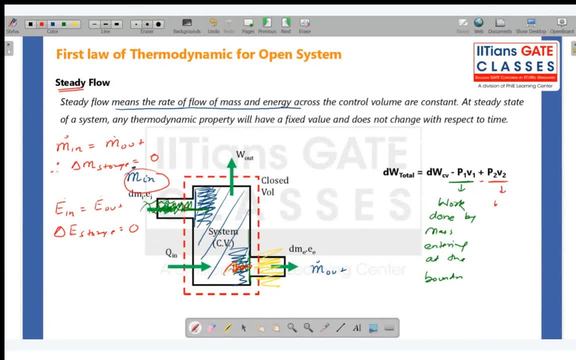 work is given positive and it is p2, v2, so it is basically work done by mass exiting outside the system. okay, so these are two extra one. now there could be one other type of work. for example: what do you have? let us say you have, you have a turbine. okay, so turbine is. 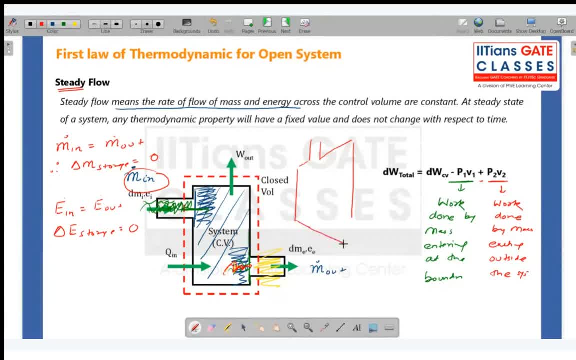 something like this: okay, so when this turbine, when mass is coming in, then this will happen. when mass is going out, this will happen. okay, because you see it is pushing the boundary. this is the boundary, but one shaft is also attached with it, so this mass that is coming in is trying to rotate this. 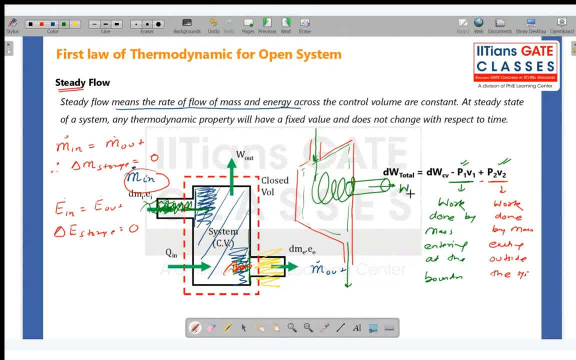 shaft and this is called a shaft work. so it is called as shaft work, or the work obtained by the system, and this is called as control volume. but the extra work that the system, from the system that you are getting is called as control system work. so the total work during this process when the mass is coming in and mass is going out and 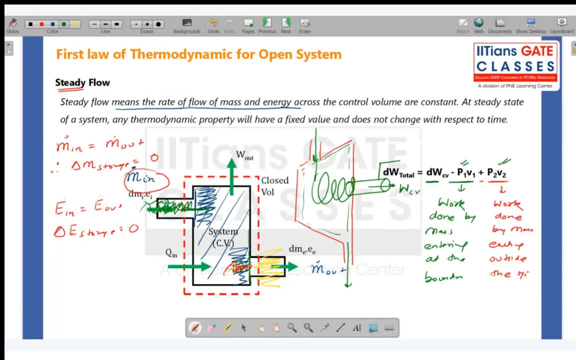 also system is giving you some work, then it is called as: the total work is basically this: now, this work you not, you will not always get. for example, if you know, like you have this nozzle, you have this nozzle, so only mass is coming in and going out. there is no control volume work. 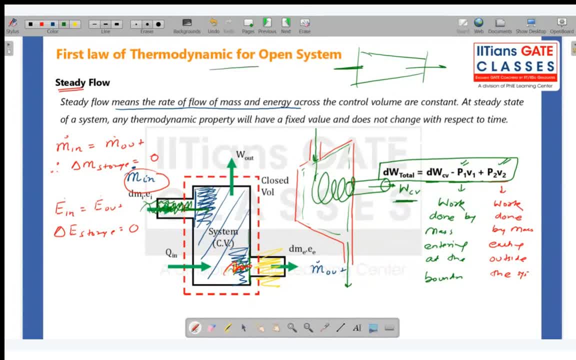 so this work will depend upon what type of system you have. for example, if you have heat exchanger, we will talk about everything, but only mass is coming in and going out. coming in and going out- no work. so sometimes it could be zero as well, but basically total work is this, is it clear? 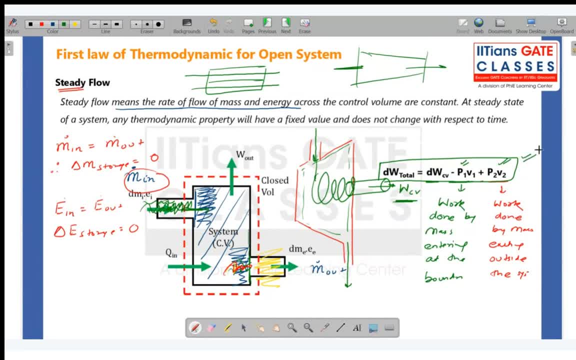 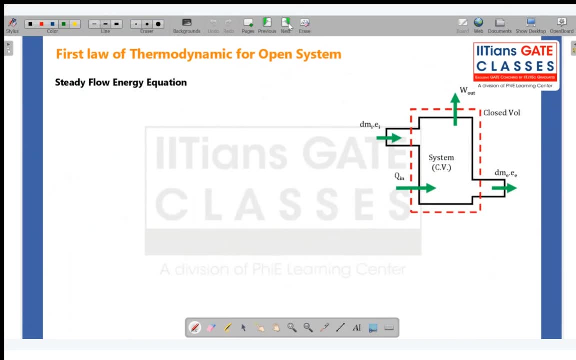 till now is it clear? then we will move ahead, okay now. so let us define our steady flow energy equation. let us define our steady flow energy equation. okay, so, as i said, always start with the first law of thermodynamics. now i am not saying for closed system, for open system, for this, for 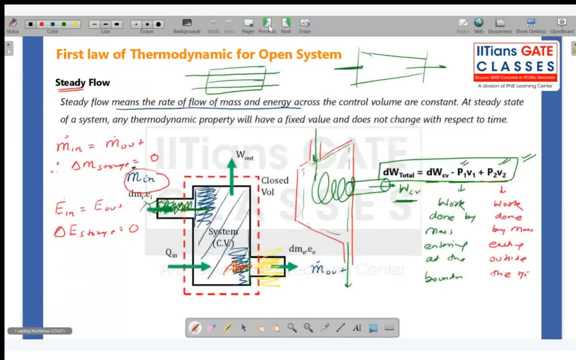 steady flow work. okay, look, you see we have a boundary here. okay, so when this mass from outside will come in, it will try to push this boundary inside. so it is basically the work done by the mass on the system. so it is basically work done on the system, and work done on the system is negative. 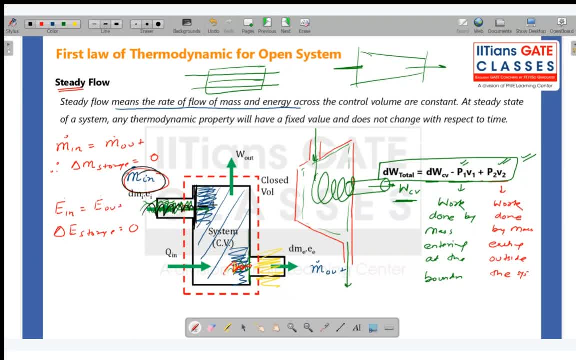 so this mass that is entering it is doing some work on the system. and what is this work? it is minus p1, v1. similarly, when this mass that is going out- and this is your boundary, let us say so- it is trying to push the boundary outside. so it is kind of expanding the volume, and volume is expanded. it is kind of an expansion work. 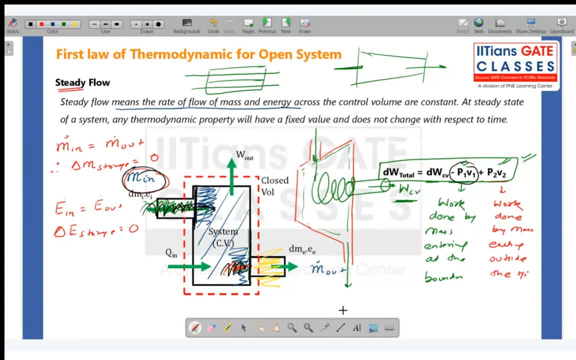 okay, so it is basically work done by the mass or work done by the system on the surrounding, so it is positive work. this is pv, p2, v2. so this is that. now there could be a different kind of work depending on your system. so, for example, you have a turbine, so turbine- this is minus p1, v1. this is 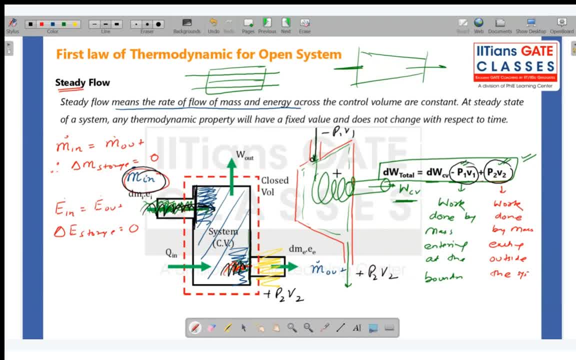 plus p2 v2. but something else is also happening. what is happening? this fluid is rotating your shaft, the shaft work you are also getting, so control volume work. it is called as. which is happening due to the system inside, due to the mass inside the system. okay, and it is crossing the boundary. of course that is called as. 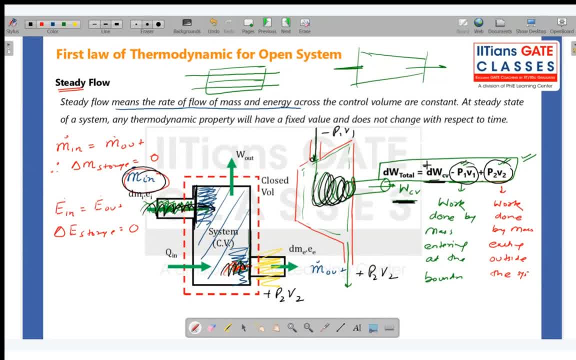 control volume. if it is compressor, then it will be minus dw. if it is nozzle, then dw control volume will be zero, because only mass is coming in. mass is going out, that's all. heat exchanger: mass is coming in, mass is going out. dw control volume will be equal to zero. got it? 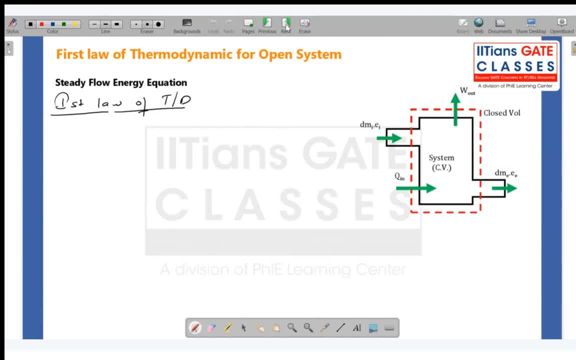 okay now. so you always start with first law of thermodynamics. and first law of thermodynamics, everyone knows it is the energy conservation equation. i am not saying for open system, closed system, whatever. it is just first law of thermodynamics, it is energy conservation, and that means energy in is equals to energy out, plus change in energy of the system. 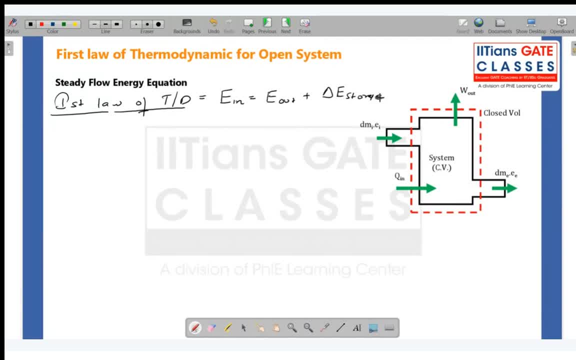 or the storage. now, i have already talked about the energy conservation equation i told you. for its td state, mass flow rate in is equals to mass flow rate out and therefore, change of mass of storage will be equal to zero. similarly, energy. okay, just wait, let me write it here because i need this space. okay, mass flow rate in is equals to mass flow rate. 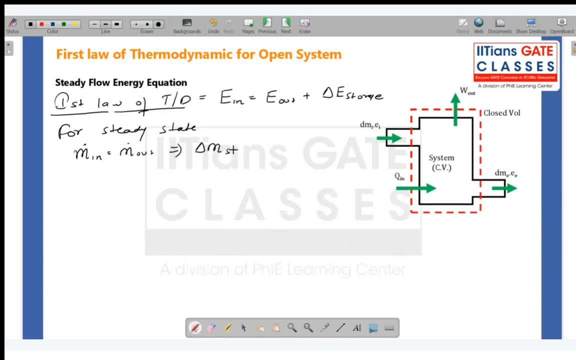 out and therefore change of mass inside the system or the storage mass is basically zero. similarly, energy dot in. whatever energy is coming in, same energy is going out. therefore there will not be any change of energy of the system and it is equals to zero. so by that, 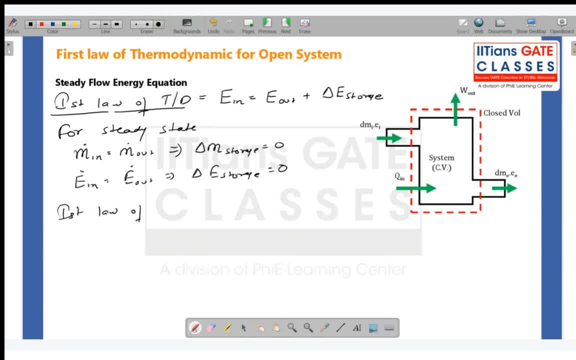 logic now if i say: first law of thermodynamics for steady flow: okay, so first law of thermodynamics. so steady flow means open system. okay, steady flow. so now i can say e in is equals to e out. why? because delta, e storage is equals to zero. is it clear to everyone? first of all, tell me till now. 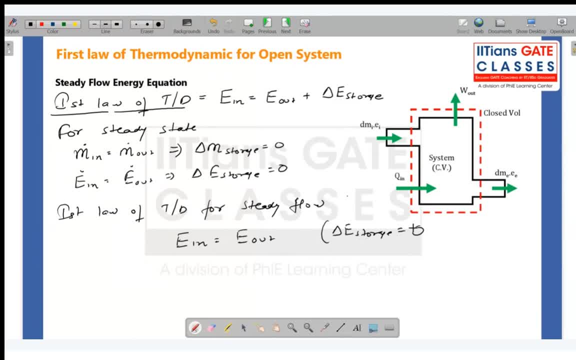 is it clear, okay now. so, as i said, so what do we have energy in equals to energy out. now, how this energy is coming in, energy is coming in two ways: what? some heat is going in and some mass is going in, and that mass is carrying some energy. you see, 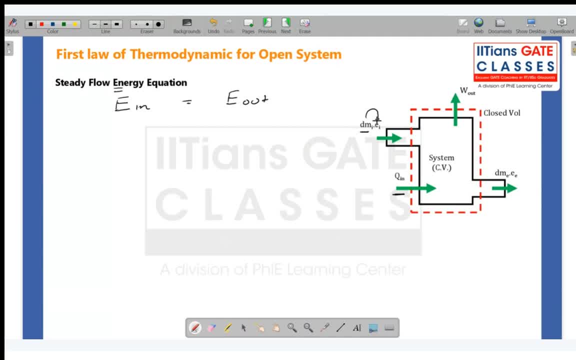 mass can store energy in. how how can it store energy? tell me very quickly how a mass can store energy very quickly. tell me. no one is telling me really today. explain this. yes, internal energy, potential energy, kinetic energy- very nice, okay. so some mass is going in and it is carrying some energy with it. also, what is what energy q in is going? 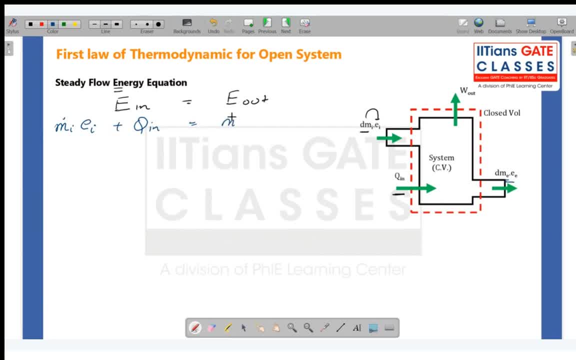 okay, what is going out? some mass is going out and it is carrying some energy with it plus some work output, if you may be getting out from it. okay, so i know that this mass can store this energy in the form of internal energy, kinetic energy and potential energy. q in this mass that is going out, it is storing energy in. 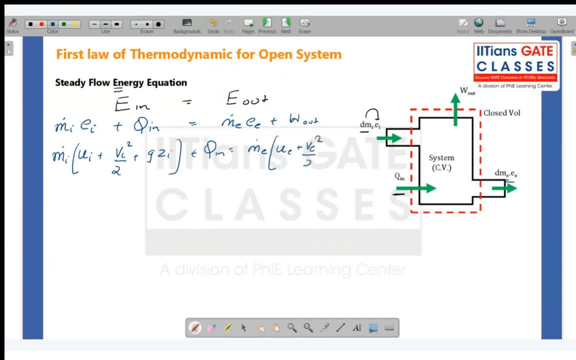 the form of exit plus v, exit square by two, plus g, z, exit plus work out. okay, now i know what is this work output. i have already defined it for you, so let me write it here. plus what is this work output? control, volume, work. so whatever this volume is doing work, then what work is coming in and what work is going out? so what? 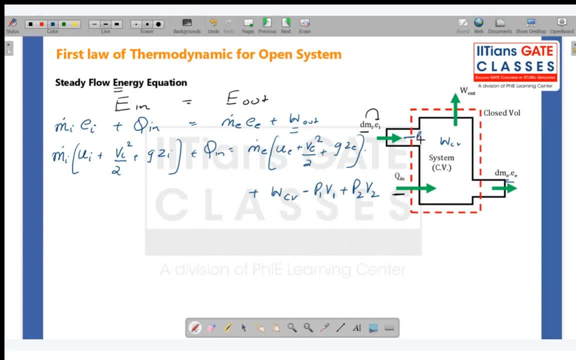 okay, so here it is. work is coming in minus p1 v1. here it is going out plus p2 v2. okay, now i can write m, dot, i ui. let me take this p1 v1 here, so i can write plus p1, capital v1 plus velocity. now this is volumes. you see, this is volume, this is velocity. 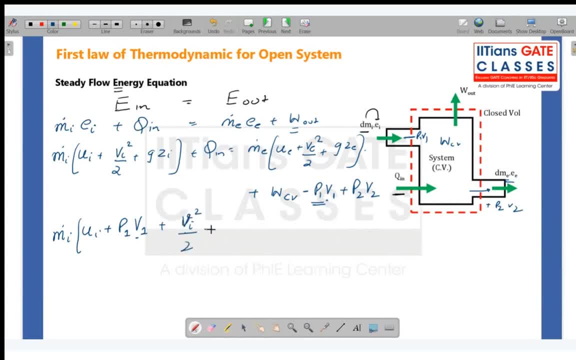 let me write it like this: can anyone tell me, am i doing anything wrong here? just in this equation? have i done anything wrong? quickly tell me. i will be very happy if you can find out what mistake i am doing. you multiplied yes, very good, very nice. yeah, that is what i was expecting from you. 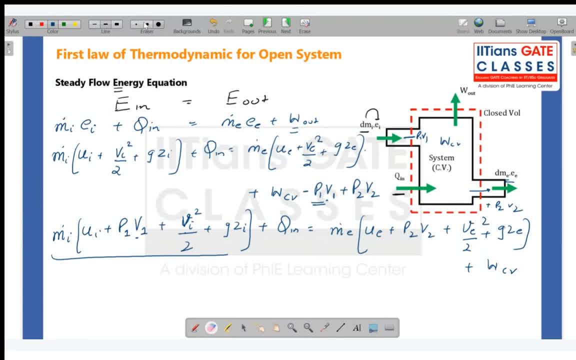 so you see, i cannot write capital v here. why it should be small v? okay, because here it is capital v. here it is capital v, but here mass is outside. okay, so i have to write a small v. here that is specific volume, okay. similarly, here also i have to write a small v because mass is outside, okay, clear. so i have. 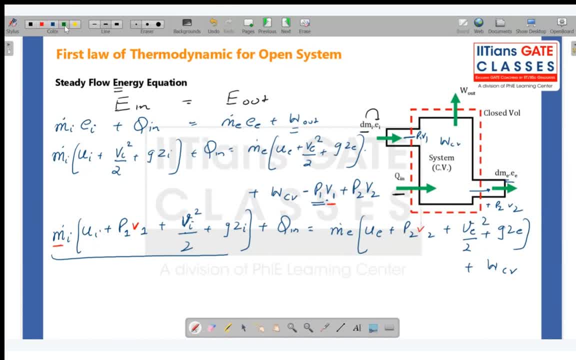 given you a big, big equation. now i can write m? i. now this is what enthalpy: h? i plus v? i, square by 2 plus g, z i plus q, in, is equals to m, dot e u e. sorry, sorry, sorry, sorry. h e plus v? e square by 2 plus g, z e plus work of control volume. 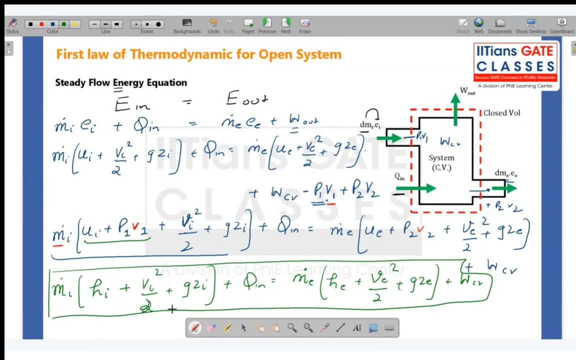 anyone need any explanation. but rate should be balanced dimensionally. yeah, yeah, i mean okay, yeah, you can do this, that's fine. i mean you can do this, okay. if you can't see, i'll do it with red. you can do this, this, this, okay. is it clear? 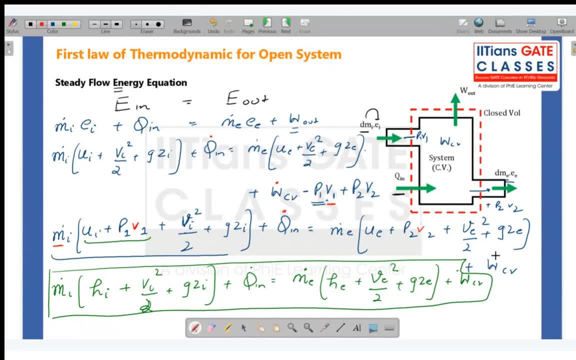 okay, okay i mean, yeah, that was my mistake. actually you have to do this because you are taking mass flow rate here, so this you have to do. dot dot, that means per unit time, okay, so basically this is our steady flow, this equation is our steady flow, energy equation. okay, very frequently you 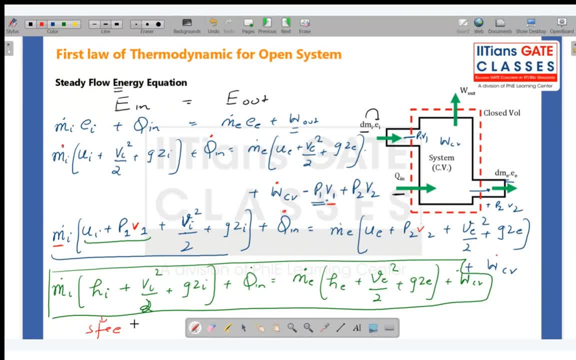 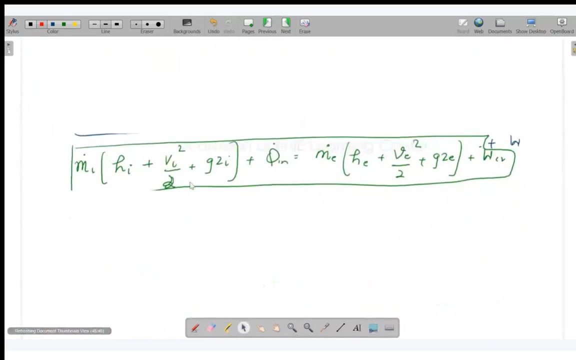 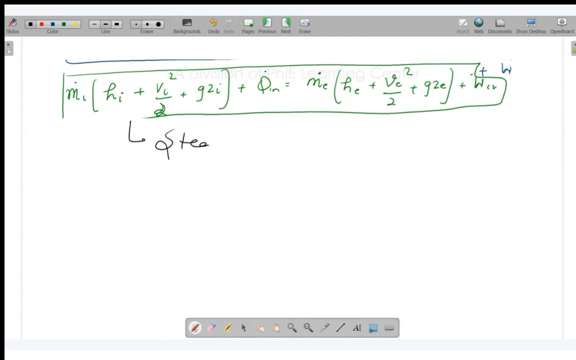 will be using that when we solve our questions. okay, so you will be using this equation and it law of thermodynamics for open system for std flows. okay, so this is my first law of thermo. let me okay, so this is basically a steady flow energy equation. or you can say: first law of thermodynamics for open system, but for what? 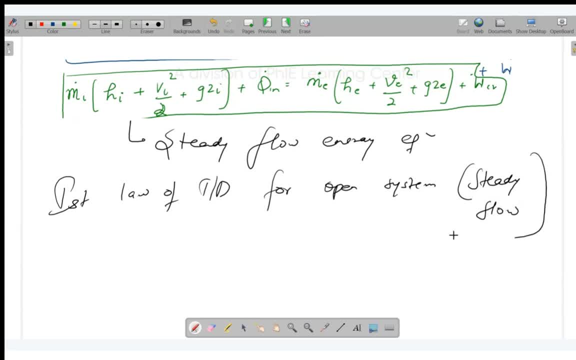 steady flow, honestly, not an unsteady flow, a steady flow. okay, now someone was saying that enthalpy and all, and what is open system? let me explain this that now. i think now we are on the stage that we can discuss that. so now you see when i take this. 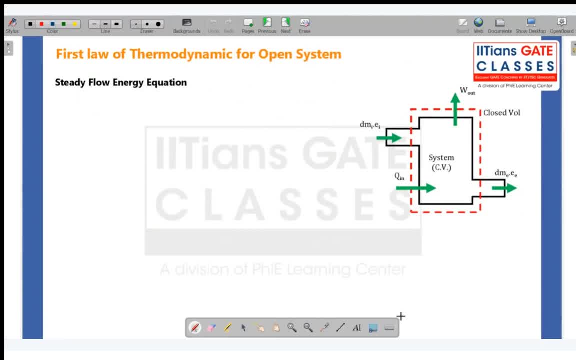 okay, when i take this system, if i have, let us say, if i have this, and this is constant volume. okay, so whatever heat i am giving, whatever heat i am giving, that heat is basically stored in terms of internal energy only. so internal energy is basically energy processed by mass in a 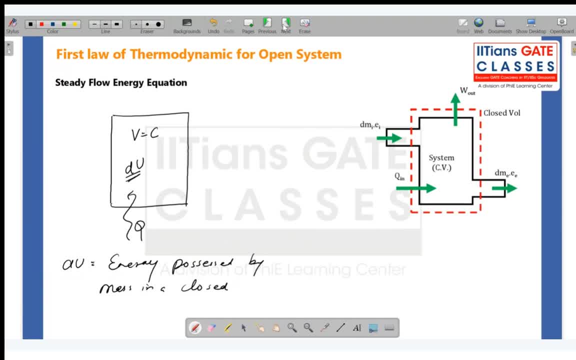 constant volume or a you know like closed system. or a closed system, okay, where there is no extra mass that is coming in. how much energy du, energy it is possessed means the mass that has that energy. whatever mass is there, it will only store du. but here, here, what will happen? whatever mass is there, 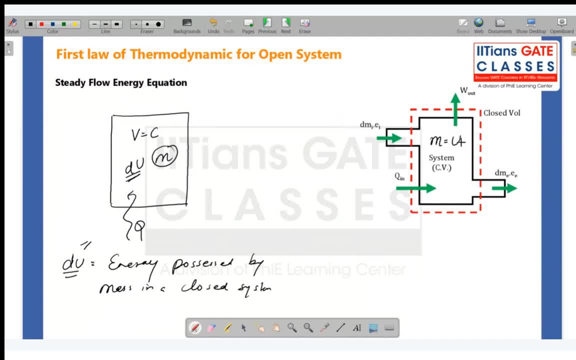 that will store energy in the form of u. and then you see, here p1 v1 is coming, here p2 v2 is coming. so basically u plus pv, so basically d, and change in mass will be du plus p1 v1 plus p2 v2. so basically, oh change. i'm sorry not change in. 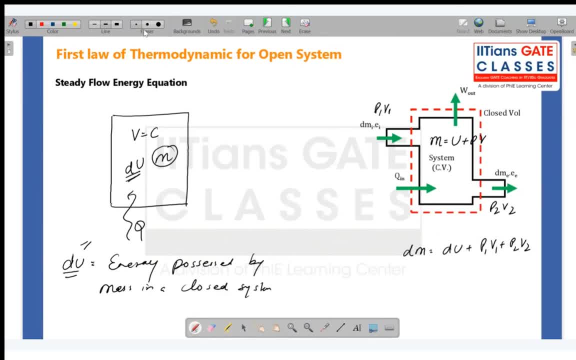 mass. i'm really sorry. it is basically the energy that is possessed by the mass. this is d e that is possessed by the mass. so here you have just du, here you have du plus p1 v minus p1 v1 plus p2 v2. so you can say: energy possessed by a open system is u. 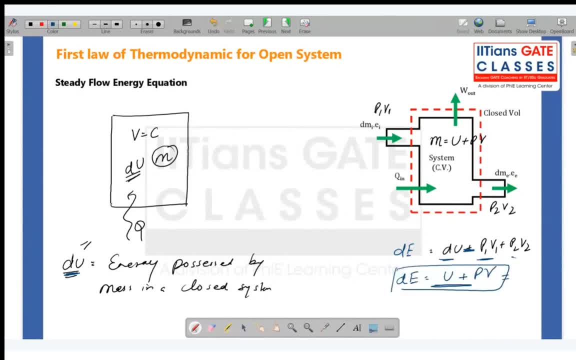 plus pv, so u plus pv, which is also dh. it is the energy by that energy that is coming in in the form of work is absorbed. what? by what? it is absorbed by this mass, only right, and this energy that is going out, it is mass that is sticking out. 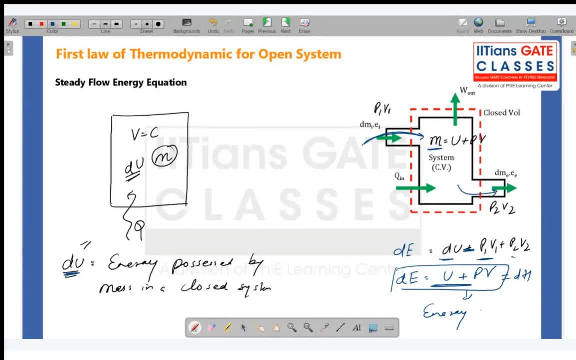 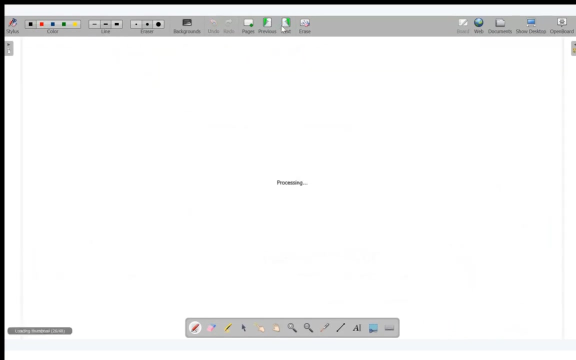 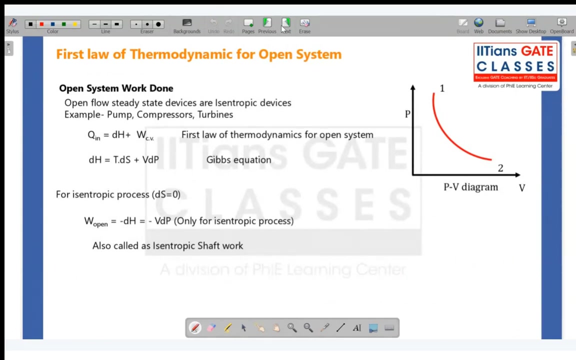 that in terms of work? where is it going from? it is going from mass only. okay, so it is energy possessed by open system. okay, yes, but energy of what system? okay, fellow, now let's come to open system work done. so open system is so most of your, you know, like. 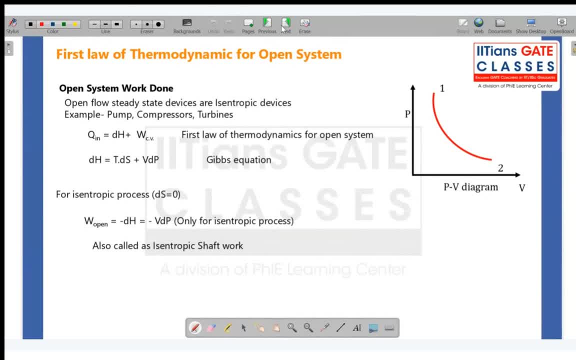 whatever uh application applications that you have in power plant, most of them are isentropic. But is this PV internally stored energy with us? Yes, it is stored internally. Yes, it is the energy possessed by the molecules. I mean again, it is a, it is work or it is heat, but it is energy only. 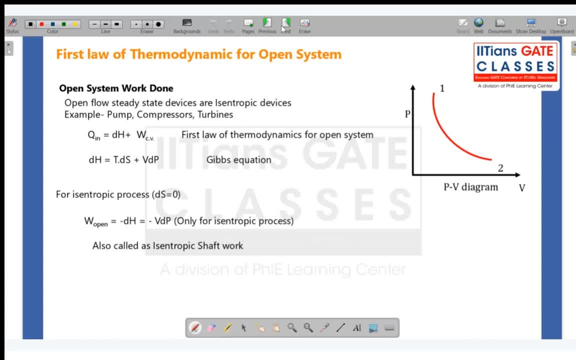 No, So PV is basically the energy that is given to the mass. OK, that mass is. where is that mass going? Mass is going inside only right. OK, so you see, most of the systems are. you see, wherever you solve your questions. 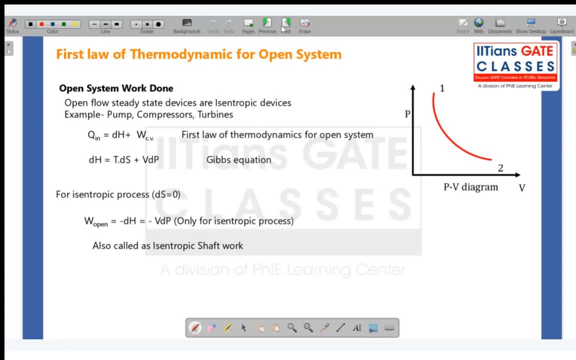 you will see isentropic turbine or isentropic compressor, So most of the processes are isentropic. Now, this is what this first law of thermodynamics for open system Right, And how will you get this? How will you get this? You? 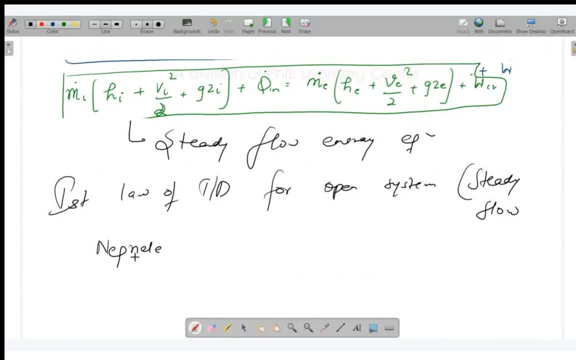 You neglect, Neglect, If you neglect Kinetic And potential energy changes. So MIHI plus Qin is equals to MEHE plus control volume. So Qin is equals to MEHE, HE minus HIY, because ME is equals to MI. 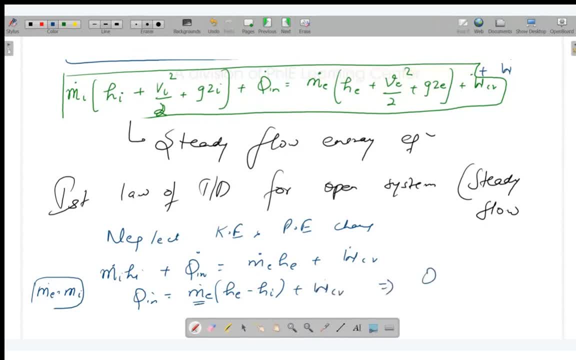 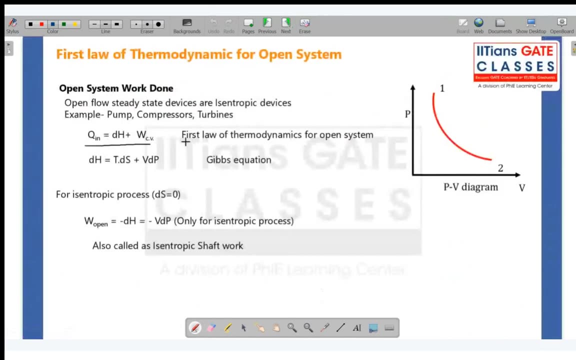 OK, plus work of control volume. So you can write: Qin is equals to DH plus DW. So this is what. open system- OK, So this is your first law of thermodynamics for open system and steady flow. And there is one more Gibbs equation that anyway I'm not going to cover. 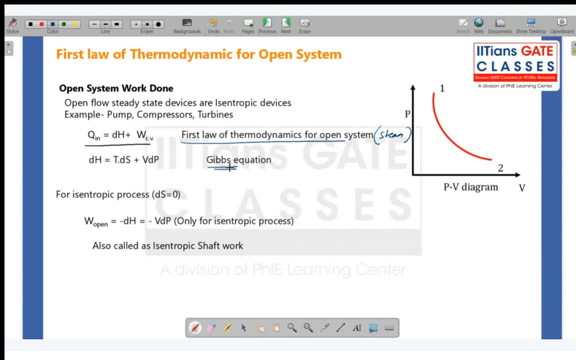 but it comes in very end. OK, so it's Gibbs equation which relates temperature and maybe I'll cover in entropy. Probably I'll cover OK And VDP, But it's not as important because you don't have to derive it. 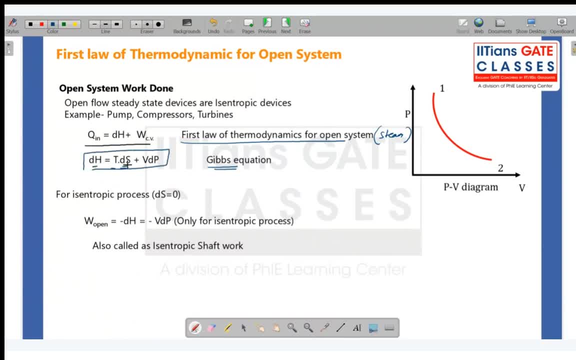 It. just you have to know that, how enthalpy and entropy are related. How enthalpy and entropy are related, Now, most of our systems, turbine compressors, they are all isentropic. Now what is isentropic? Isentropic is reversible adiabatic. 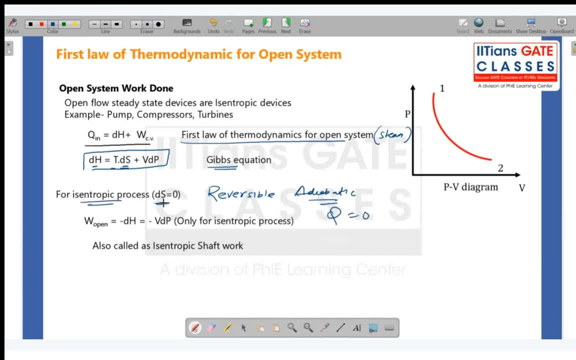 So adiabatic means Q is equals to zero. Isentropic means DS is equals to zero. OK, so in this equation if DS is equals to zero, and in this equation if Q is equals to zero and if I replace DH, 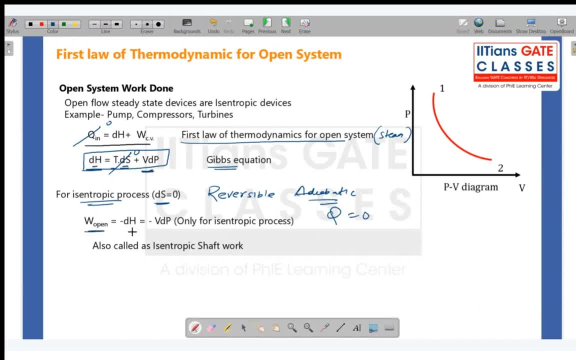 by VDP. so open work is equals to: From this equation I can write, Control volume work is equals to minus DH And then by this equation I can write, is equals to minus VDP, minus VDP. But you can only apply this in case of turbine. 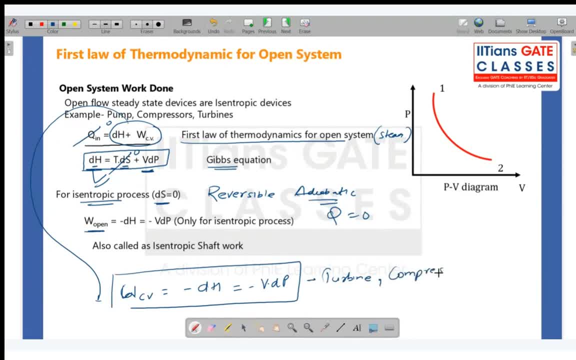 And compressors, because turbine and compression ninety nine percent, they are isentropic. in the question they will give you isentropic, OK. So if you remember closed system work was what, Can you tell me what was closed system work? 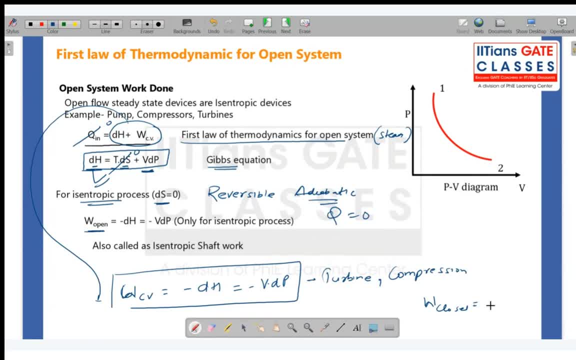 General equation, general equation, quickly, Quickly, PDV. Was it not one to two? Now you remember? Yes, so basically, at a given pressure, at an intermediate pressure, change in volume. so what did we do? We took a small pressure and we defined it like this: 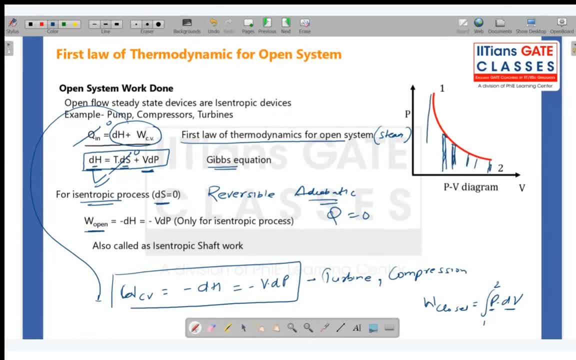 And then we did it infinite number of times And we said that this area of an extended on volume axis gives you closed system work. Now, same thing we are going to do with open system work. So here it is VDP. it is VDP. 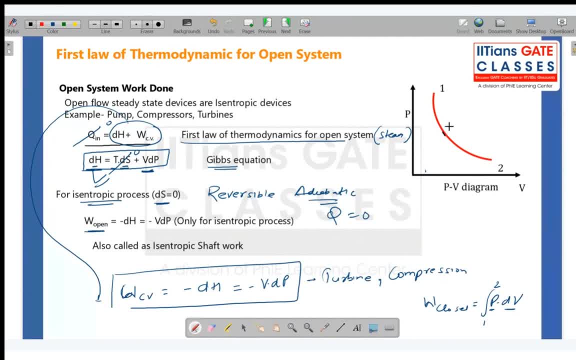 So what we are going to do, we are going to take a very small volume, intermediate volume- And See what is the change in pressure here. So this is what we will take. It is P Dash. Sorry, we dash. 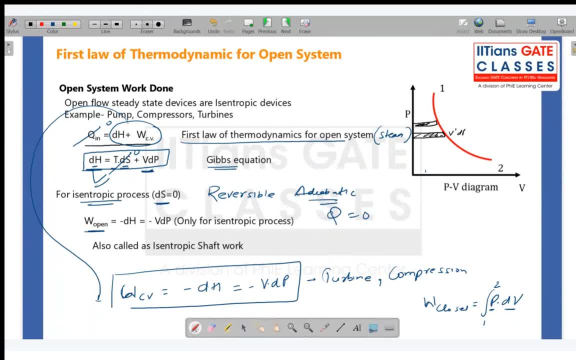 We dash DP, then we will do it infinite number of times, very, very small. We double dash DP, then we will do here, then we will do here And basically we will cover this whole area. And this is basically Area. 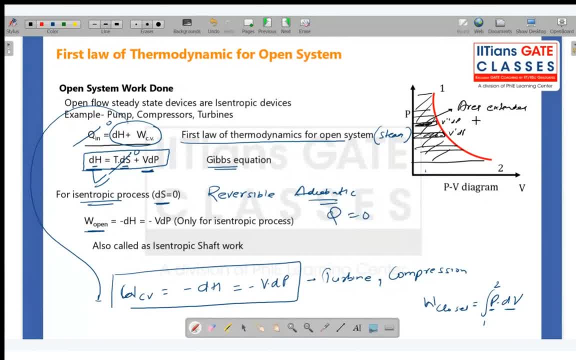 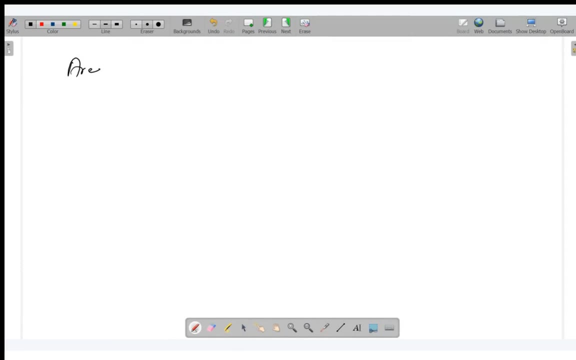 Extended On pressure axis On PV curve, is what Is open system work? Open system work Again. if you don't remember, let me write it: Area Under Curve: Open Curve When extended On volume axis. 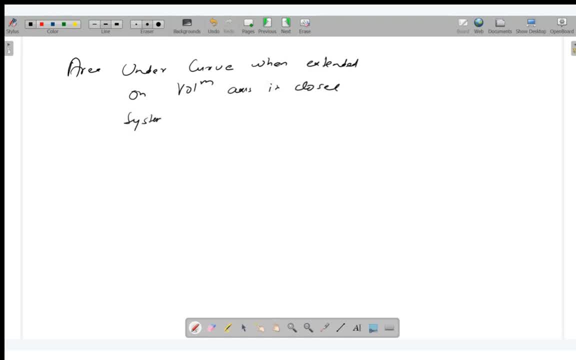 Is Closed, System Work. OK. PV: Where are you going to extend it? Volume axis? So this is your work: Open, Closed, OK. Then area Under curve, When extended On pressure axis, Is open system work. 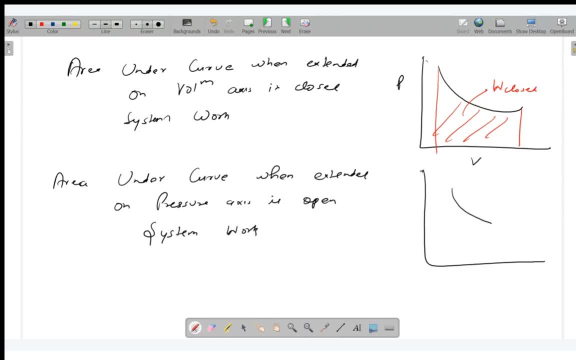 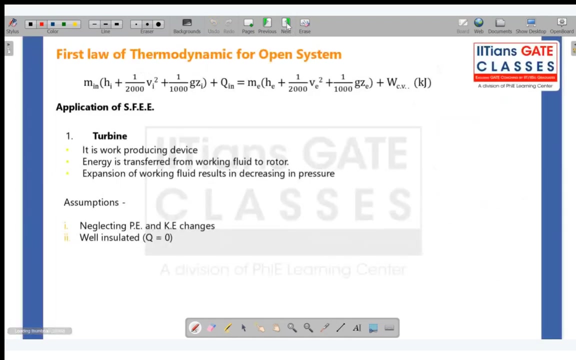 Open System Pressure Volume. Where are you going to extend it? Pressure axis? So this is work Open, Am I clear? Quickly, OK, Now let us see the applications. Let us see the applications of a steady flow. 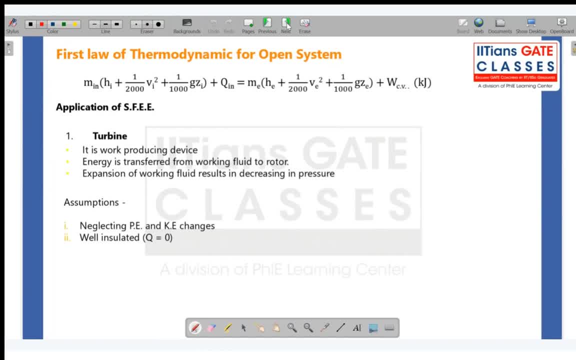 All the devices that you have in power plant. they are all steady flow. OK, They are all open system and a steady flow. So this is my main equation. I'm going to apply all my assumptions based on this. OK, So turbine: 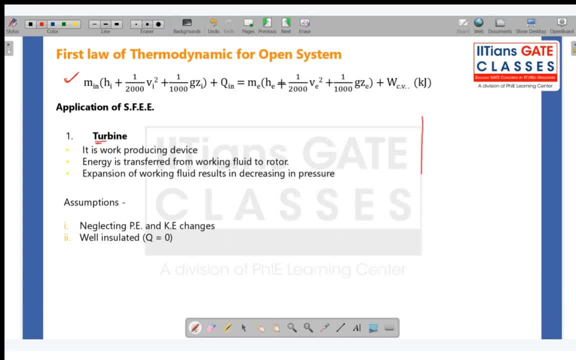 We all know what is turbine. What does a turbine do? Turbine is a work. Turbine is a work producing device or a work absorbing device. Work producing. So mass is entering here, Mass is going out, Work. What we are getting 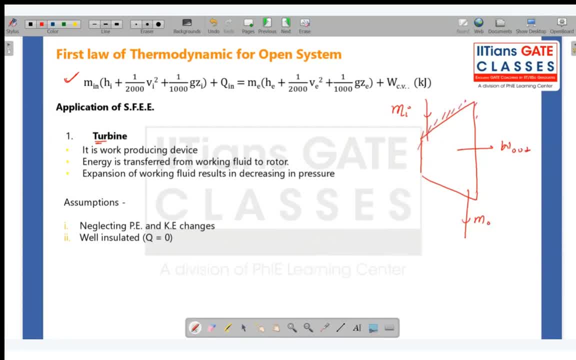 OK, And all the way it is isentropic. It is isentropic. So isentropic means what? How much is DQ? How much is DQ Is Zero, Yes, So it is well insulated. that means Q is equals to zero. 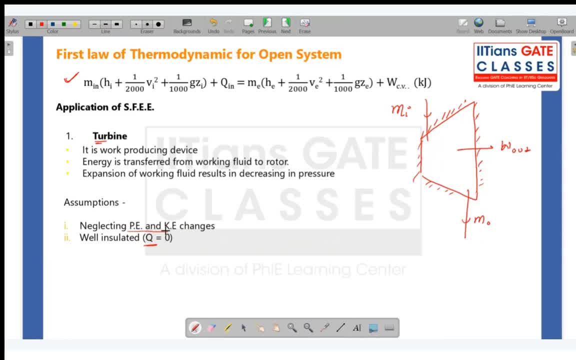 And I'm also going to neglect kinetic and potential energy changes. So if I neglect kinetic energy potential energy, kinetic energy potential energy. also well insulated, It means isentropic is basically. So this is zero. So I have M dot I H. I is equals to M dot E H E plus control volume work. 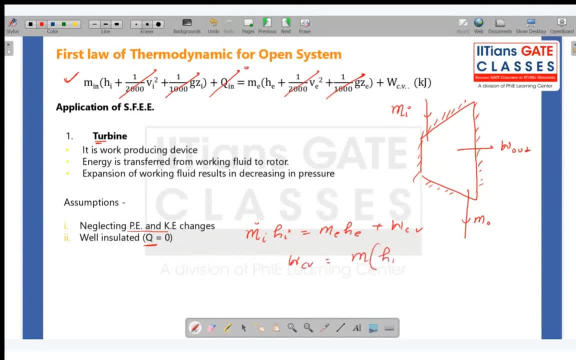 So control volume work is equals to M H I minus H E. So this is how you can calculate work transfer for a turbine. You can directly apply this And kilojoule OK, I don't think there is much to explain here. 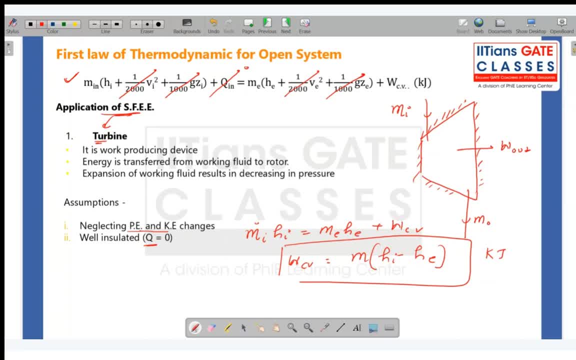 It's just the application of steady flow in a turbine. OK, if kinetic and potential energy are given, then you have to put it the values. I am assuming that we are taking it at zero, But in question they might give you kinetic and velocity and that they will give you. 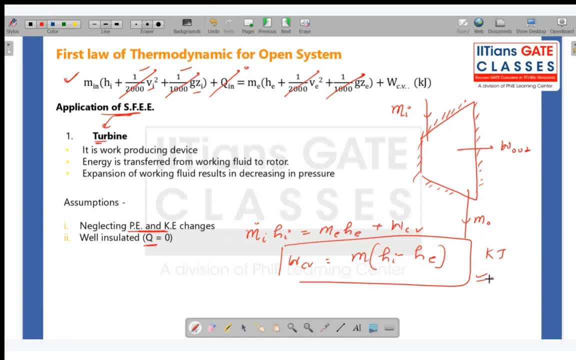 So you have to take it. That's all. Do not blindly assume that this is the formula that you are going to use. Clear, I don't think there is much to explain here. Then we have compressor. quickly, I'll go up to everyone. 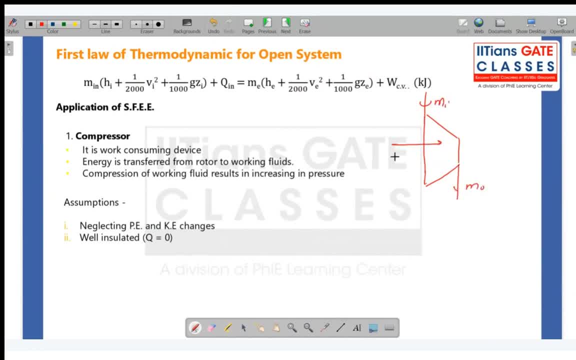 So here, mass in, mass out, their work is in the Yankee. It will be negative. OK, again, it is a work consuming device, Compressors of work consuming device, So I will neglect kinetic and potential energy changes. Well insulated, So this is zero. 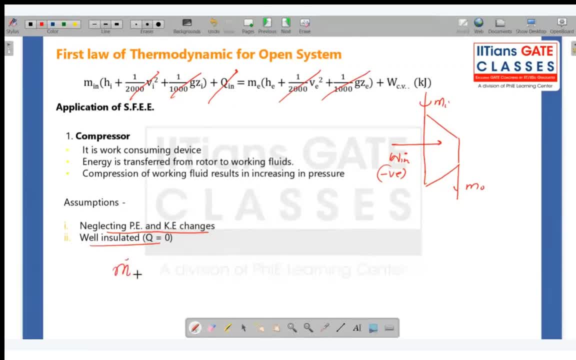 This will go away. This will go away. This will go away. Mass in H I is equals to mass exit, H, exit. Now you see, this is basically we have taken. If you remember, we have taken it on the energy out. 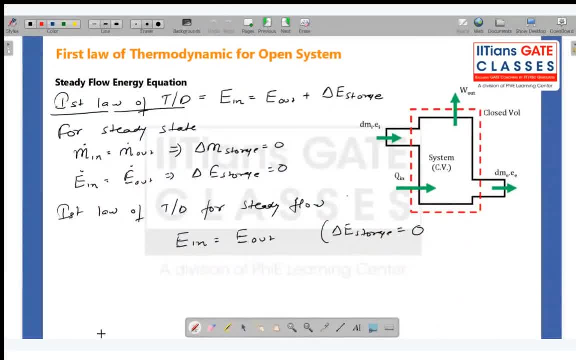 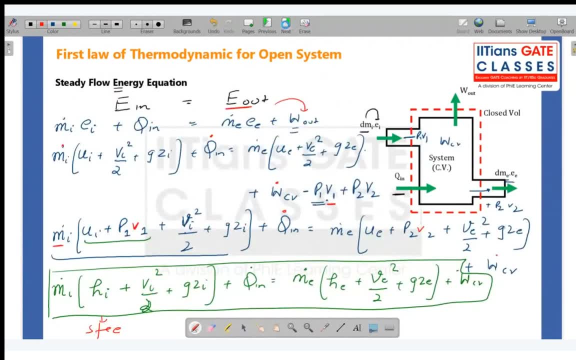 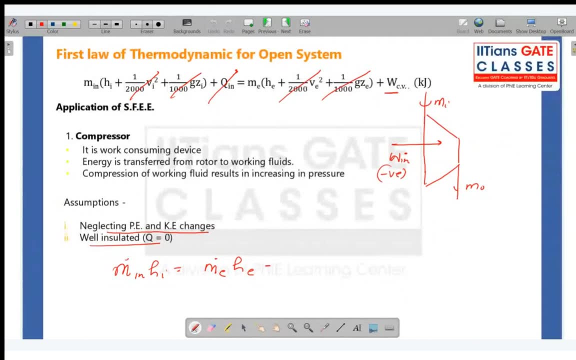 I hope you remember this. OK, we defined energy out. Where is it OK? next page. We defined energy out and we took it as work output, But here, in this case, it is work input. in the term In compressor, it is work input. 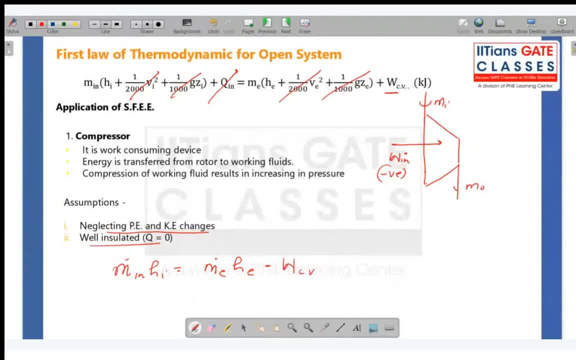 So I will write minus work of control volume. OK, so work of control volume is equals to M H exit, minus H I for a compressor. So you can calculate it like this: Every question is applicable for this particular scenario. OK, next is what I'm just quickly going. 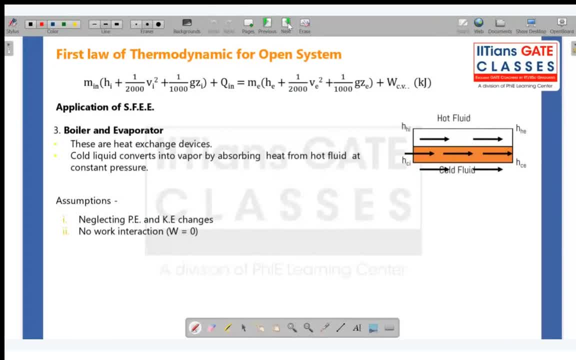 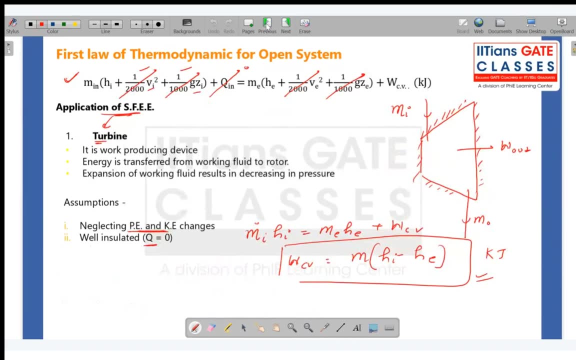 through it because there is not much to explain here. OK, now, if you have heat exchangers, Yes, of course. OK, you want to explain me how that is basically? you know, like more of applications part, but you see what is what is and what is enthalpy. 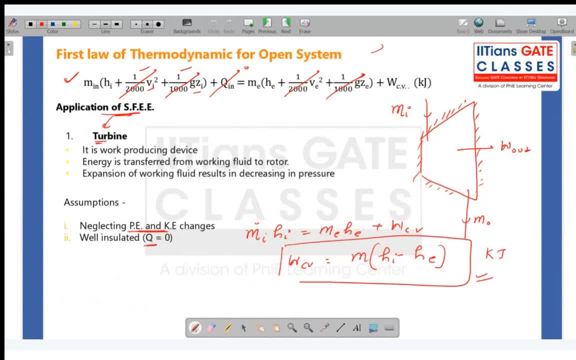 Can you tell me what is enthalpy? Enthalpy is the energy, U plus PV, So it is basically the energy that the mass has. Now, when this mass is coming in, it is a very high temperature and very high pressure. 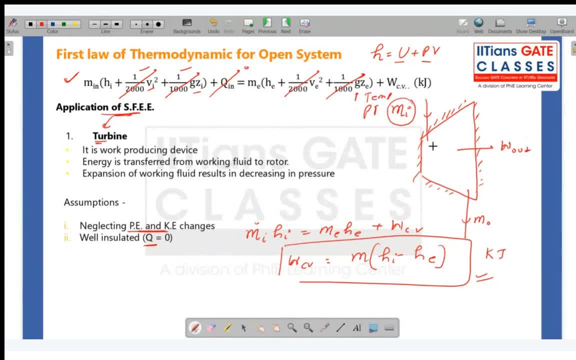 OK and yes, and then you have rotors here. OK, you have rotors here. Now, when this coming at a very high pressure, this pressure is applied to the rotors and these rotors. this energy is utilized to rotate the rotors. 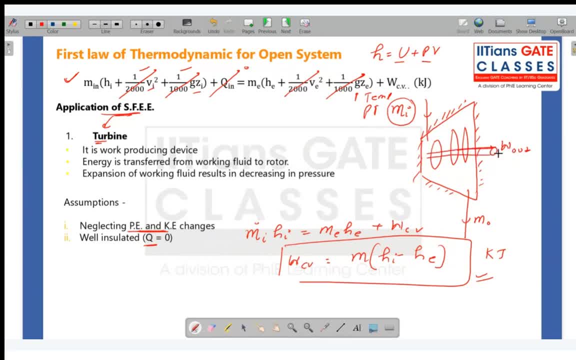 OK, and this rotors are connected to the shaft, So you will rotate the shaft, You will connect the shaft and you can. you know it is the output. basically It is the mechanical work output, but the energy that this mass has has been given to the rotors. 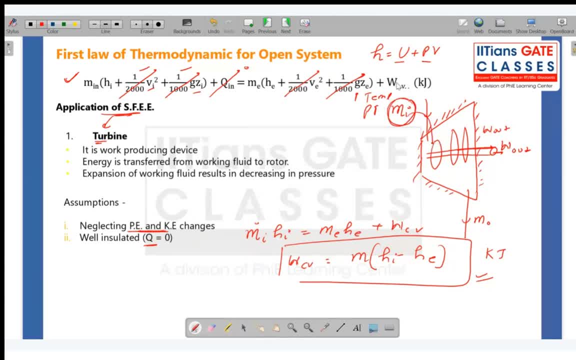 This pressure is given to the rotors, The pressure will reduce, temperature will reduce. So if temperature will reduce, You will reduce, this will reduce to: basically: enthalpy will also reduce. OK, simply, in simple words, I would tell you that the energy 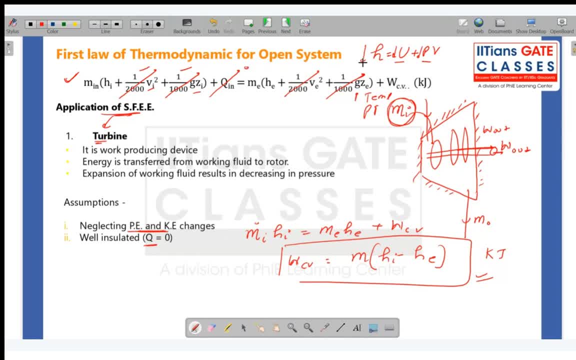 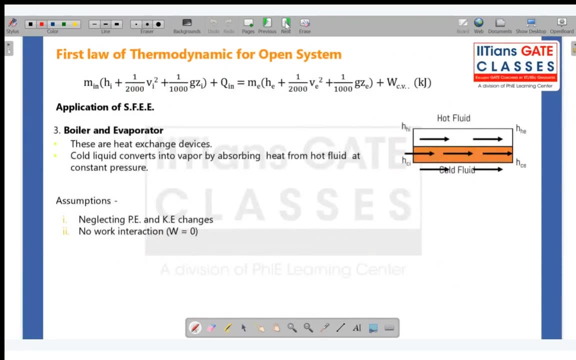 that the mass has is basically given to the rotors and that energy is reduced when the mass comes out, and that's the enthalpy reduction, Enthalpy energy reduction. OK, clear, Yes, I mean you can say that. yes, because temperature is also. 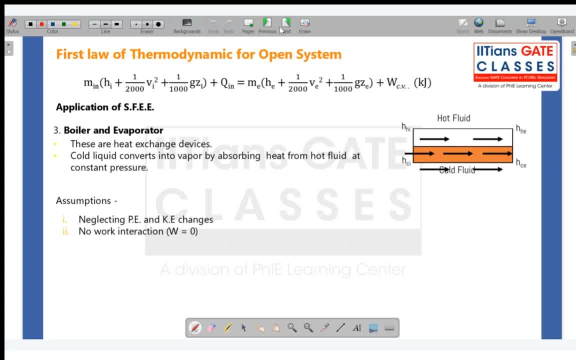 you know varying in the inside, the inside the turbine. Are you relating it with the heat transfer? Do not say you want me to consider heat transfer. No, really, I mean, it's not heat transfer. heat transfer is what Heat transfer basically should happen from the 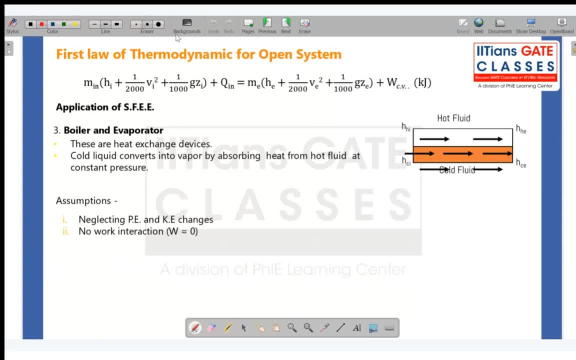 boundary. This is the more. this is the energy contained by the molecules. You see, the thermal energy that you are talking about is basically energy contained by the molecules. So it is an internal phenomenon. It is not outer, It is not crossing any boundary or something. 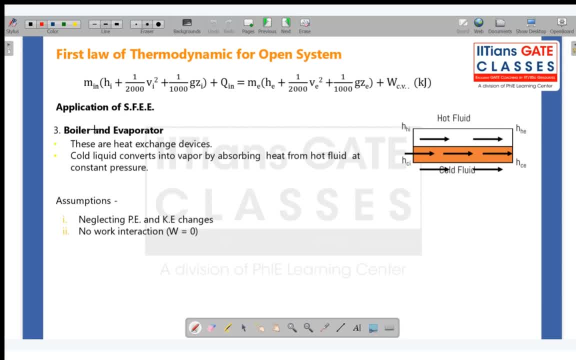 OK, Hello. Now let's go to boiler or evaporators. OK, basically a heat exchanger. let us say Now what is happening: Hot fluid is flowing through here, Cold fluid is flowing through here And heat transfer is happening between them. 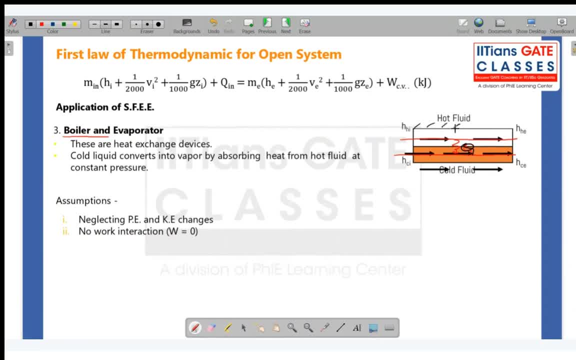 Q. Heat transfer is happening between them, But the outer area of the heat exchanger is basically insulated, So no heat exchange is happening between system and surrounding, So Q will be zero. Q will be zero, Or OK, this is Q in. it is taking just one second. 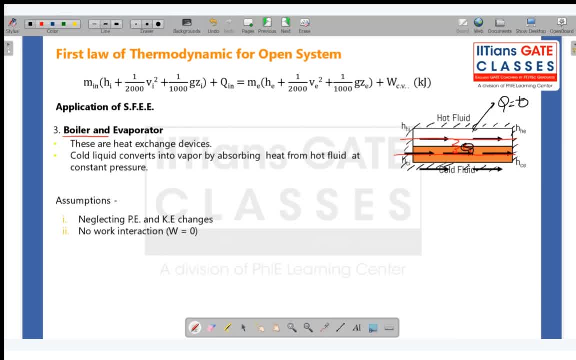 OK, OK, Here, what we can do is we can take one system, So You cannot take the whole system. then, Actually, you can do this two ways, OK, let me. let me explain you both the ways, So so that 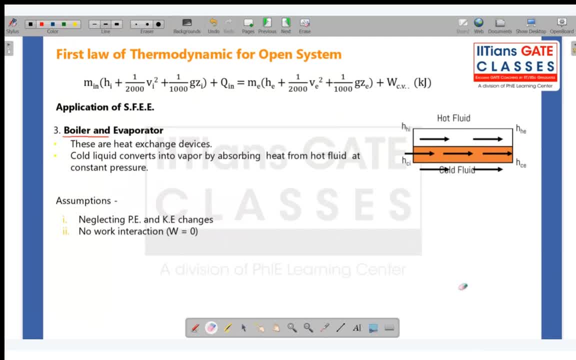 I mean just one second. OK, let me explain two ways. First, let me take the whole boundary. Let me take the whole boundary as a system. So what is happening here? Hot fluid is flowing in, cold fluid is flowing in. heat transfer is happening internally. 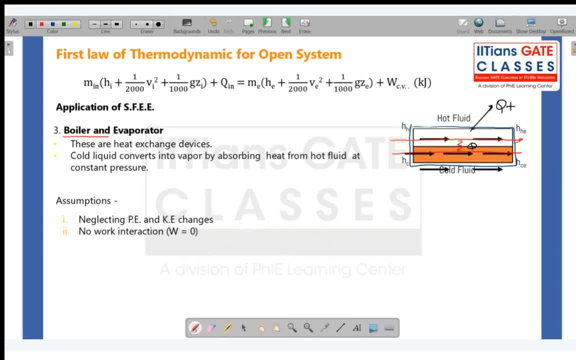 But there is no heat transfer between the system and surrounding, So Q is equals to zero. OK, so in that case what will happen is in that What will happen is that this kinetic and potential energy we are neglecting anyway. OK, and in heat transfer, we all know that there is no work done. 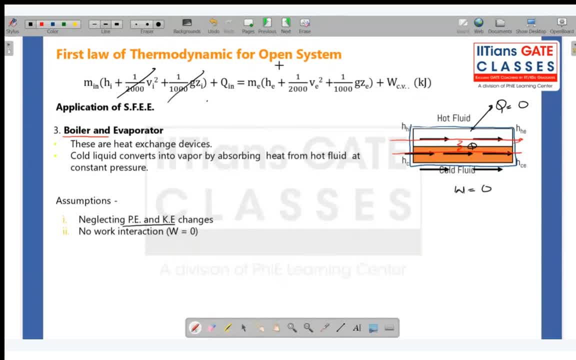 So work is equal to zero, So this is also zero. This is negligible. This is negligible. This is negligible. No work transfer, no heat transfer. So basically, what can I say? in this particular scenario, M dot in H I is equals to: 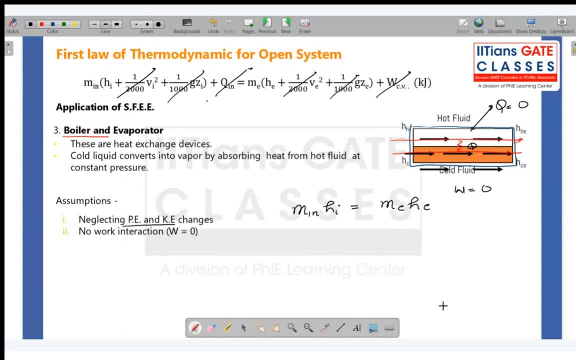 M dot E, H E. OK, now what mass is coming in? Mass is coming in: M. mass of hot fluid. H of hot fluid in. OK, mass of hot fluid out. sorry, mass of cold fluid in. Cold fluid in. enthalpy of cold fluid in. 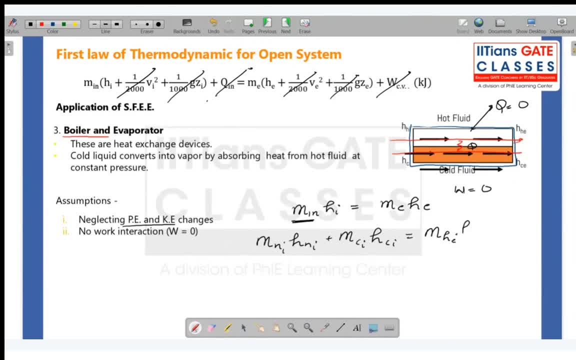 Mass of hot fluid exit: enthalpy of hot fluid exit Plus mass of cold fluid exit: enthalpy of cold fluid exit. So this equation you can use to calculate your heat. Basically it's you have, you are equating. 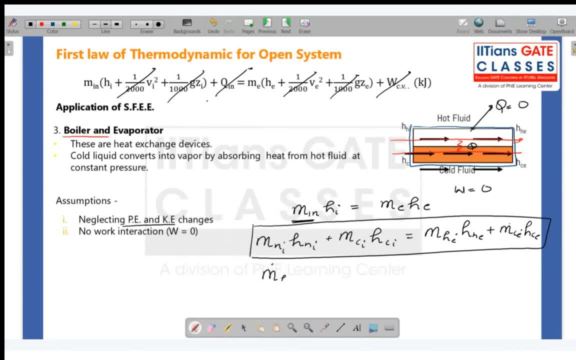 This is: if I say M dot H H H I minus H H E is equals to M dot C H C E minus H C I. So this is basically the heat rejected By hot fluid And this is the heat absorbed or heat gained. 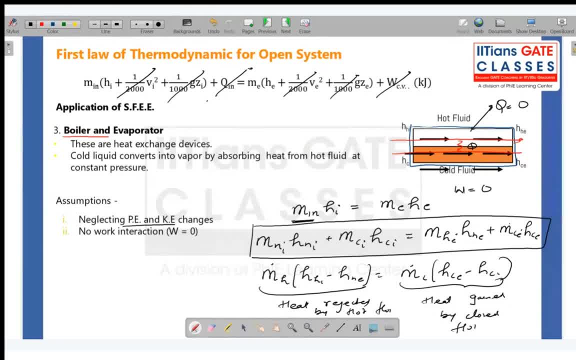 By cold fluid. OK, this is something that you will use in heat exchanger as well, OK, so this is the scenario when we are assuming that the- I mean we are assuming that this is my boundary, OK, now. Now, what can I do is let me take one more page. 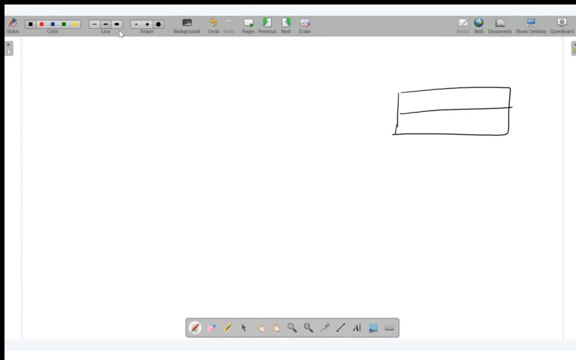 And if I say, only This is my boundary, Only the hot fluid is my boundary, OK. so heat in, heat out is happening here, from hot fluid to cold fluid, OK, and hot fluid is coming. M dot H Cold fluid. 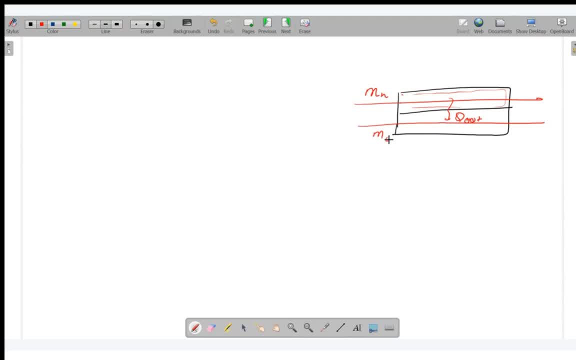 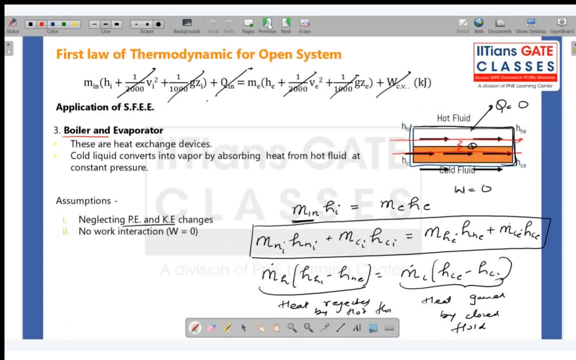 So now, what will happen now? Which one? the last one, This one? OK, it's, it's actually simple, it's not? I mean, OK, let me explain it. Look, Let me assume that this is the Boundary of the system. OK, now. 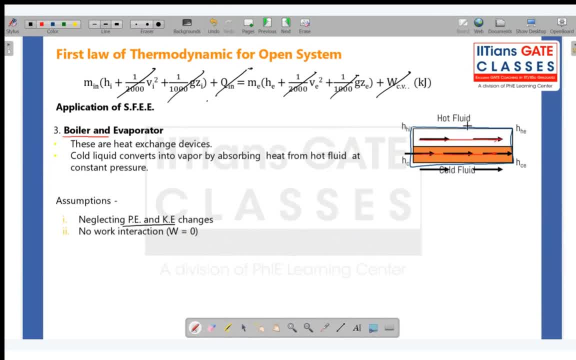 when the hot fluid is flowing here, cold fluid is flowing here, heat transfer is happening internally. it is not crossing the boundary, So it is not crossing the boundary. That means Q is equals to zero. Now, work is anyway zero for a heat exchanger. 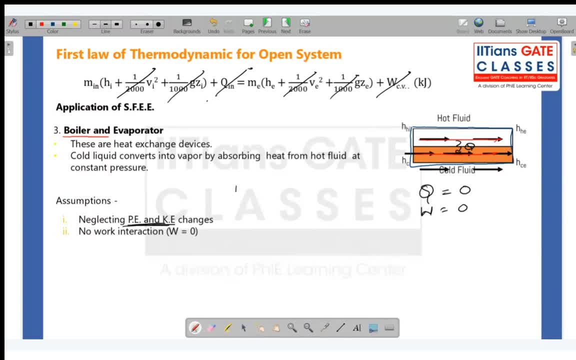 I am neglecting kinetic and potential energies. So what is left in the equation? It is simple: M I H I is equals to M E H E. OK, now, what is entering? You see, this is entering, and this is entering. 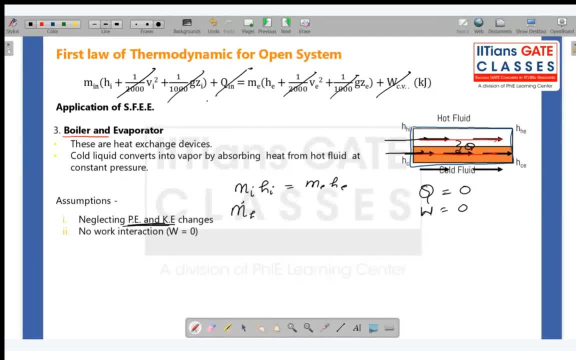 So hot fluid is entering, M dot, H, I and enthalpy of hot fluid. in plus, what is entering here? cold fluid is entering. So M dot C entering and H dot C entering. Now what is going out? Hot fluid is going out. 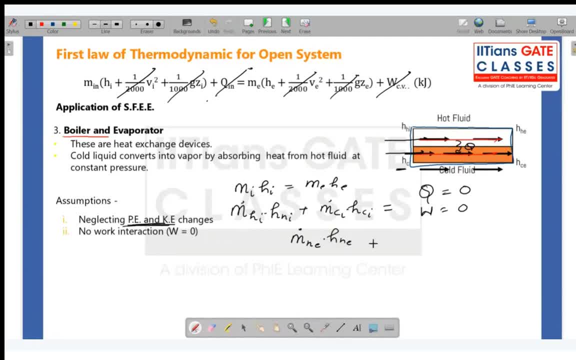 M dot H exit into H dot H exit. Then you will do questions, then it will be more clear. OK, Plus what is going out? Cold fluid is going out. OK. so it is a general equation. Now, if you want to simplify it more, 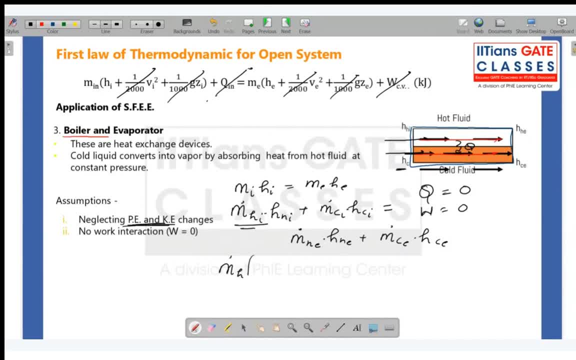 what you can do is you can bring all the hot fluid one side, So H I minus. you will take the other side, H H E cold fluid. Then you will take the other side. OK, M dot C, H C E minus H C I. 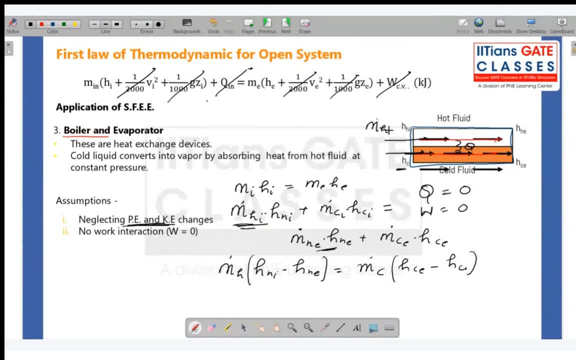 OK, again, by whatever is entering, M dot H is constant, Right. So M dot H, entering and leaving, will remain same. Similarly, M dot C, entering and leaving, will remain same. Now, what is this? This is basically energy, This Q. you see, this hot fluid is losing some energy. 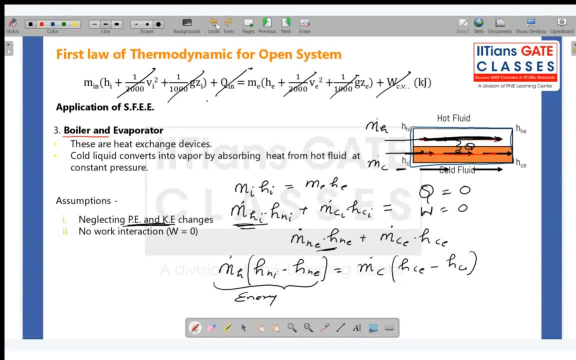 That energy is going to the cold fluid, so it is the heat. Let me write in short: OK, what did I rub? So this is basically Heat rejected by hot fluid And this is Q absorbed by cold fluid. OK, I hope it is clear this time. 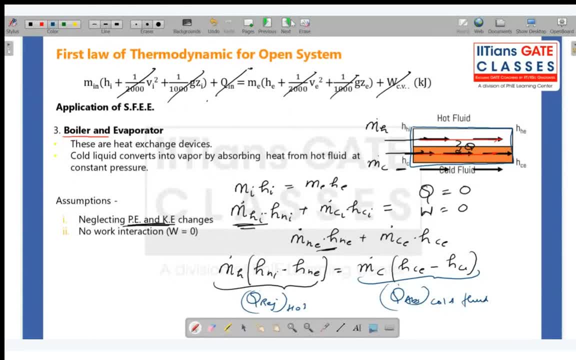 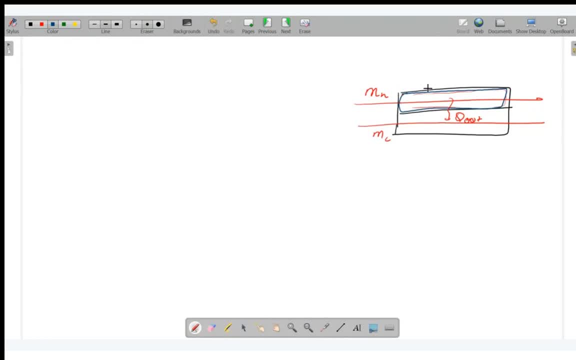 When you do more questions, it will be clear: OK, now, Let me take one example. Now, this is this time, This is my system. OK, So in this scenario, I will have M dot I, H I Plus Q in. 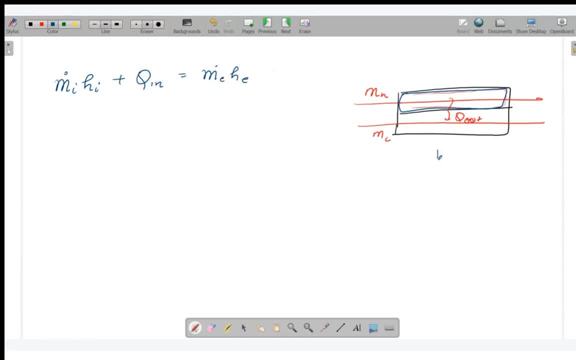 Is equals to M dot E H E, because work is zero kinetic and potential energy are Neglected. OK, so in this case, M dot I H I Minus Q is equals to M dot E H E. OK, now here: Q is equals to M dot I H I minus M dot E H E. 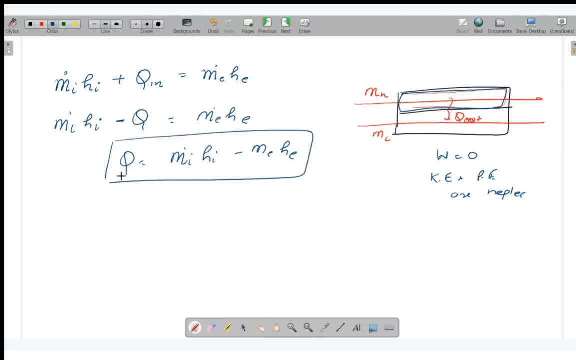 OK, now this is for what This is for, If you want to calculate how much heat is gained by the cold fluid. so Q absorbed is equals to M dot C, H I minus H E. So you can calculate it using this formula. 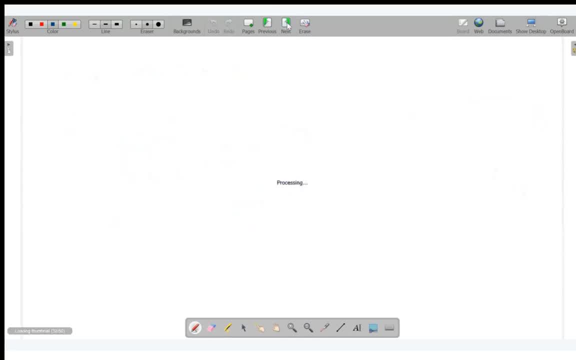 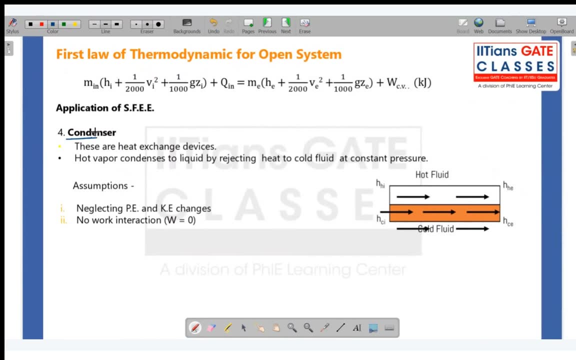 OK, Now Same thing applies for a condenser. It's again a heat exchanger, OK, But condenser. what happens? It is Rejected. OK, sorry, heat is absorbed. actually, hot vapor condenses to liquid by rejecting heat to cold fluid. 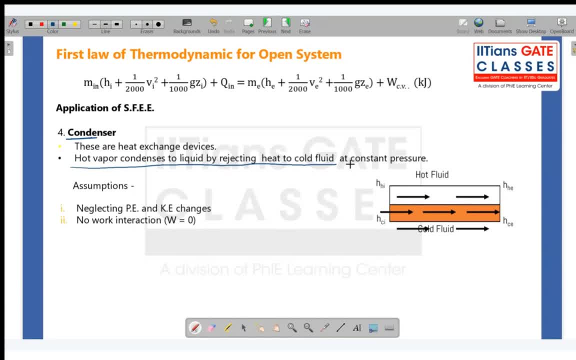 OK, so here cold fluid will be rejecting heat. This heat to cold fluid at constant pressure. OK, so condenser. what happens in condenser anyone? What is the purpose of what is condensing? I think we discussed this as well. 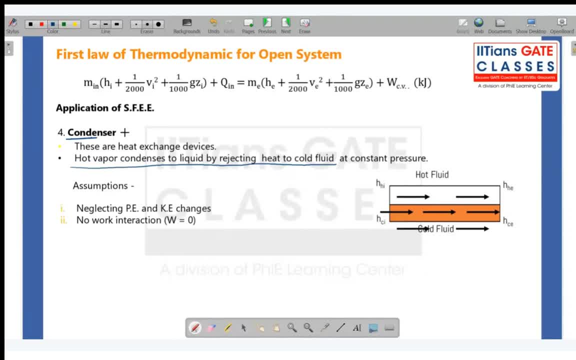 What is condensing? Condensing is basically Condensing is basically conversion Of vapor To Liquid. so that means If I have a fluid And I need to condense this, then it need to reject some heat. OK, it need to. 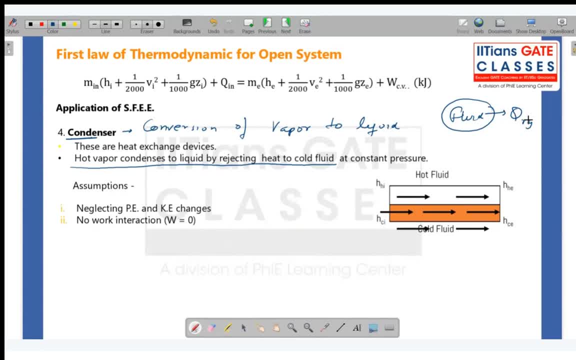 Yes, hot condense. You know, condensation is the process of converting Vapor to condense, vapor to liquid, OK. evaporation is the process of converting liquid to vapor, or boil or boiling, OK. so same thing you are going to do here. 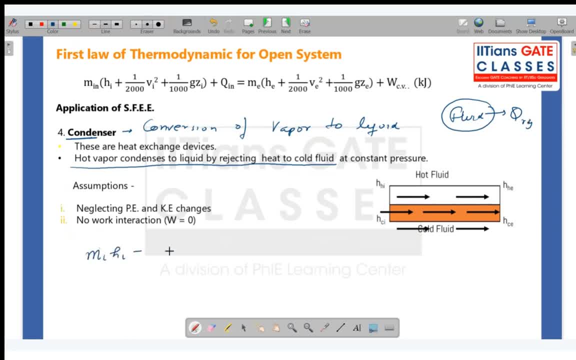 You can. M dot I, H I, Q in is equals to M dot E, H E. So Q in, You know condenser- is equals to M dot H I minus H E. Simple, OK. so basically you have to apply this. 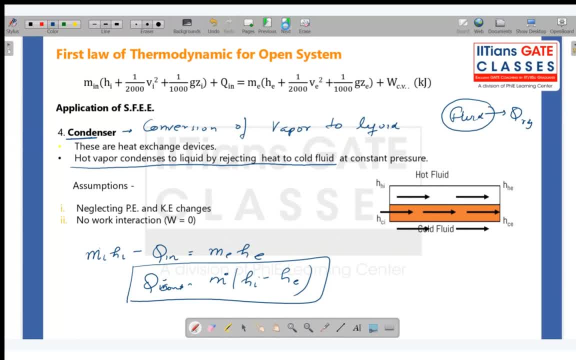 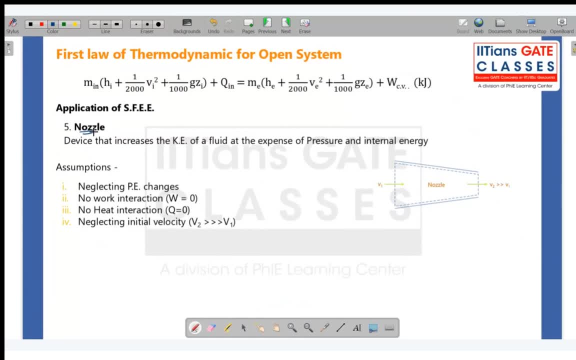 steady flow energy equation based upon what is given to you in question. There are other applications as well. for example, you have nozzle. So what is the purpose of nozzle? The sole purpose of nozzle is to increase the kinetic energy of the fluid. 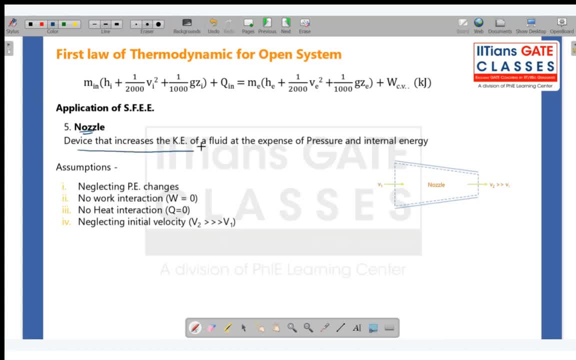 OK, the Device that increase the kinetic energy of the fluid. OK, so all other changes. Now it does not do any work. It is insulated, So Q is equals to zero. Also, the purpose is to increase the kinetic energy means. 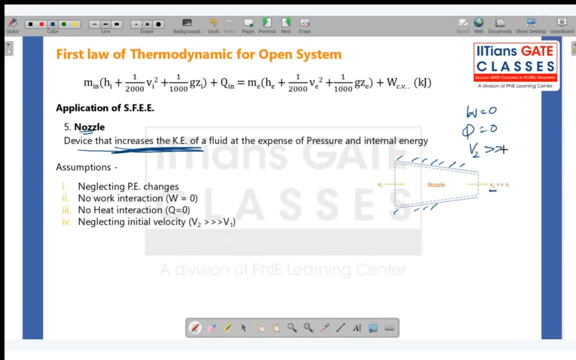 Exit velocity, which is V2.. It is much, much greater than V1.. Yes, to accelerate the fluid. So if I apply this in our equation, what will I have? M, I, H, I plus I can write V. I square by 2000 here, but I am not writing it by because V1 is. 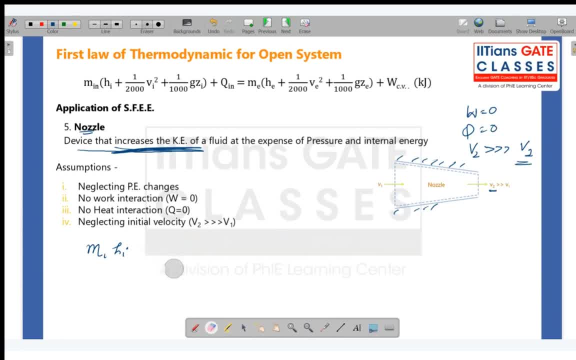 negligible. so I am not writing this because it is neglected. OK, Plus- This is also zero- is equals to M dot E plus V, square by 2000, plus work is zero, So exit velocity will be equal to under route 2000.. 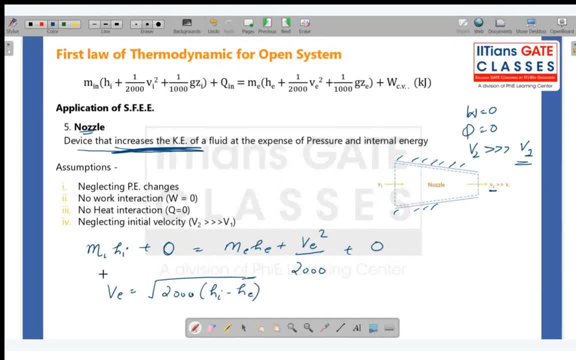 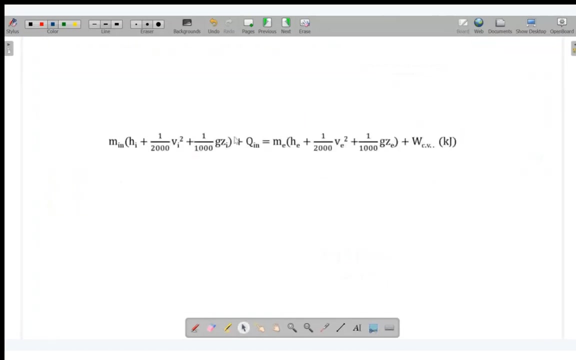 H, I minus H. Now I know that you will have some doubt that where this, this 2000, came from. Do you have this doubt or someone can explain me? OK, M I and M E is same. right, Whatever is entering, same is going out. 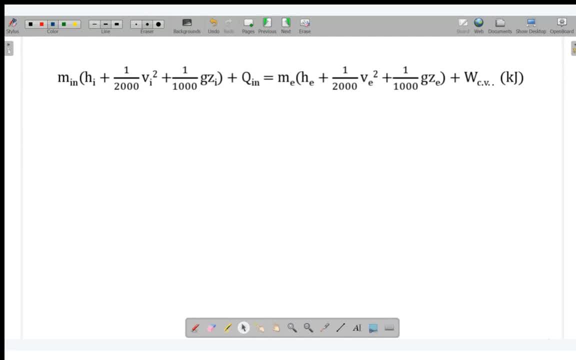 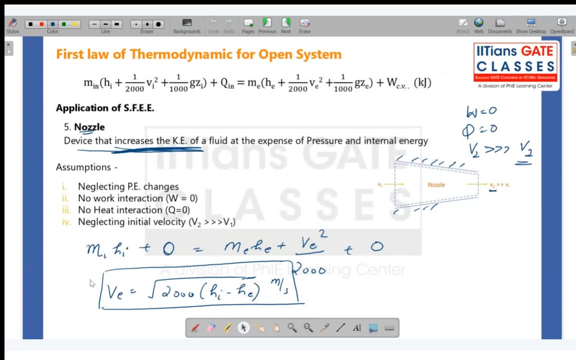 That is the basic nature of steady flow. Right, You can cancel that, You can, you can cancel that. OK, Now Also, basically here also: you will have me, sorry You're also, you will have M E, and then it can get cancelled. 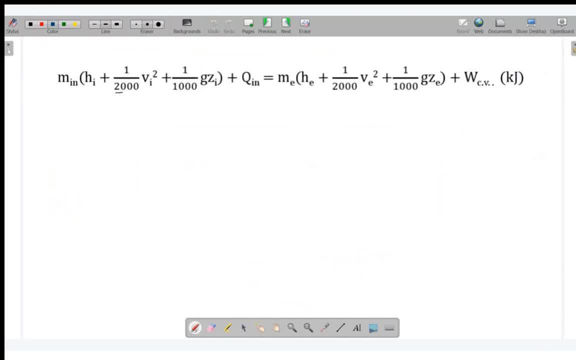 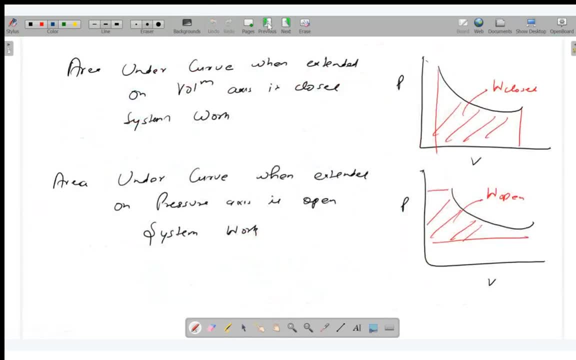 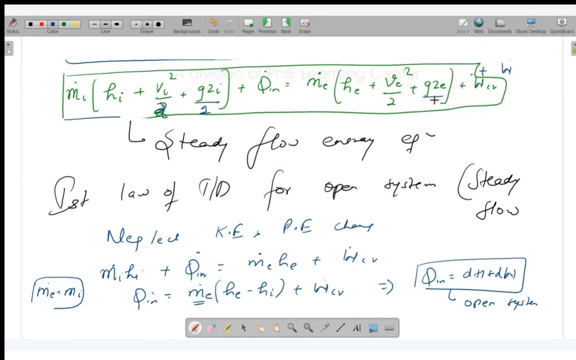 OK now. So does anyone had this doubt? where does this? 2000 came from? One thousand came from, because our question was this. This was my question. I write it to here and I write one here. I write two here and one here. 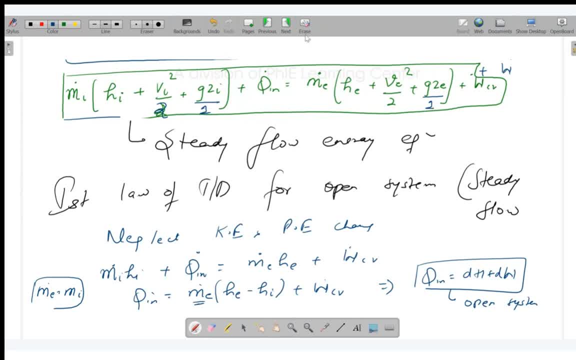 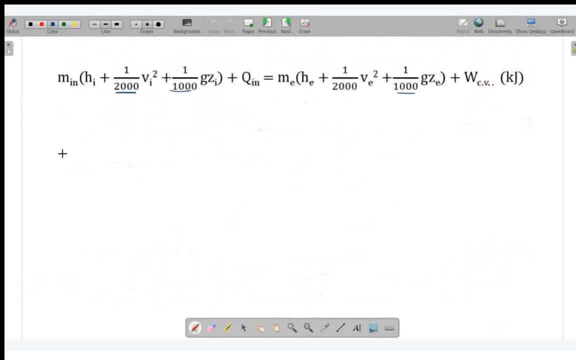 Yes, very nice, Very good. OK. now the problem here is: you see, If you are using this equation, if you are putting this enthalpy in joules, then you will use V1, square by two and GZI. 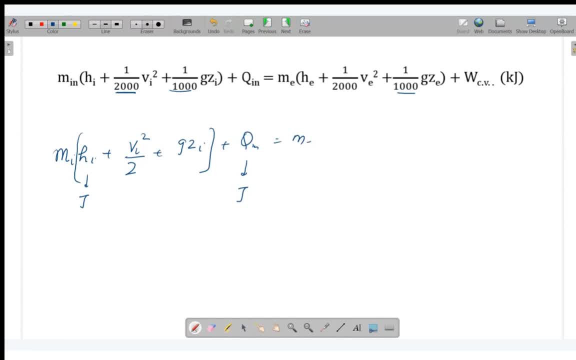 Plus Q in this should also be in joules, OK. M? E- this should also be in joules. plus V, square by two plus GZI by one, And this should also be in joules, OK. so if This equation is in joules, you can use this equation. 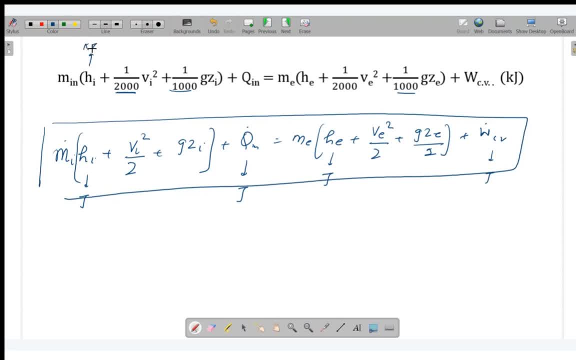 but you see, sometimes enthalpy value is given in kilojoules, heat transfer is given in kilojoules, Again, this is given in kilojoules. Or this is given in kilojoules. But you see, if you multiply mass with velocity, mass and velocity. 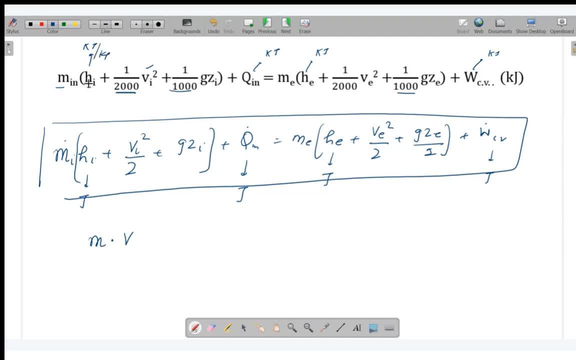 OK, so basically this will be given in kilojoules per kg, because it is small, h. OK. now mass and velocity is basically what Kg meter per second? OK, so if we, if we explore more, I can do that here as well. 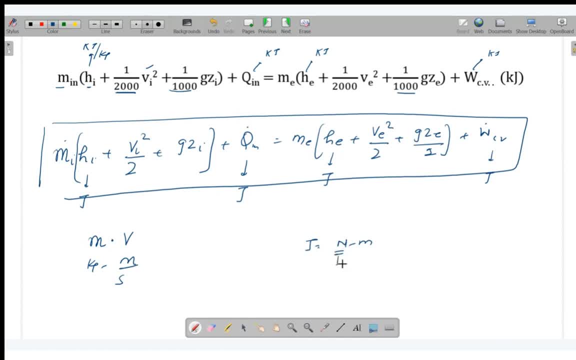 So basically joule is Newton meter, Newton is what Newton is, force into acceleration. So force is what? No one second Force into acceleration, No one second. one second Joule is Newton meter and Newton is what Newton is force and force is mass into acceleration. 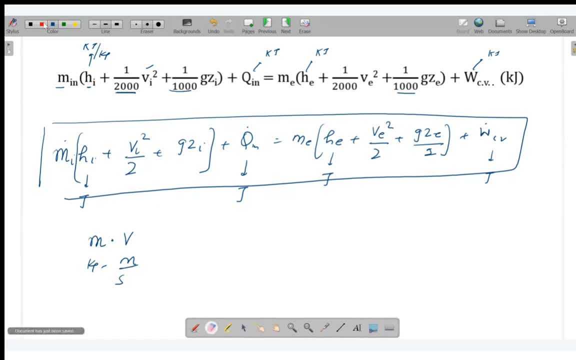 Yeah, just one second Again, do not get confused with this. Just one second. I just want to show you something. Joule is what Joule is Newton meter. OK, now Newton is what Force? We explain force by: 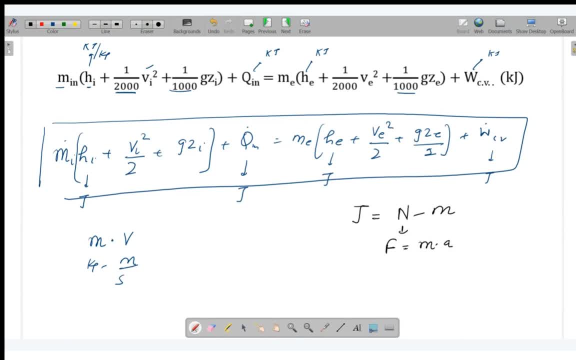 We express force by Newton. Now force is equal to mass into acceleration. What is mass? Mass is kg, Acceleration is meter per second square. Now I take this meter as well here. So kg meter square, second square. So this is equal to basically joule. 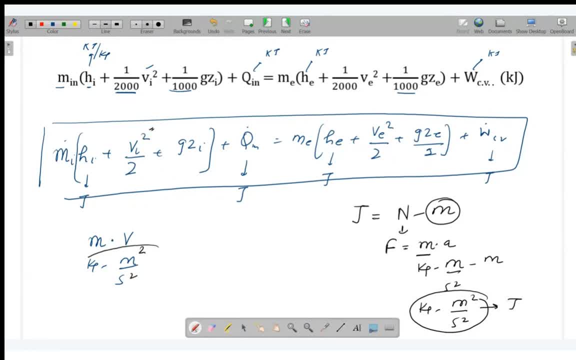 OK, so here also we have vi square. So this is equal to joule. Now to convert, because this is given in kilojoules, to convert this value, also in kilojoules, I have to divide by one thousand. So basically, instead of two you will take it two thousand. 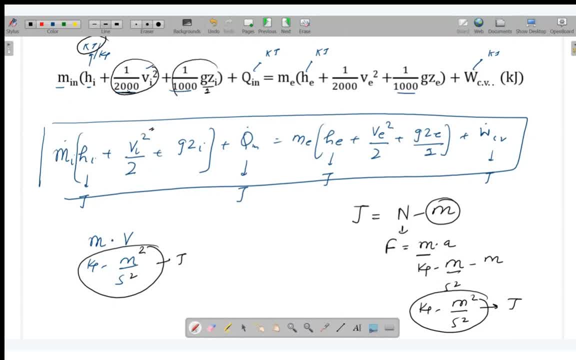 Similarly here, instead of one, you will take it one thousand, because this is also in joules. This is also in joules. So if enthalpy is in kilojoule, you will use this equation. Is it clear? So this is kilojoule equation. 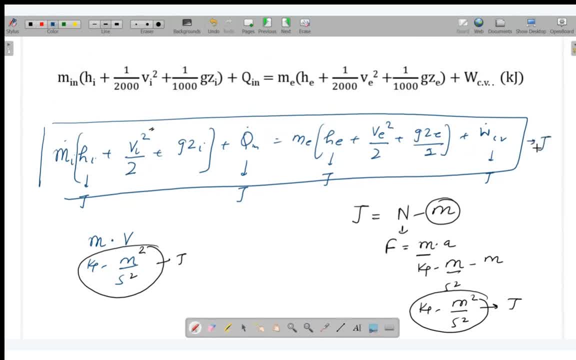 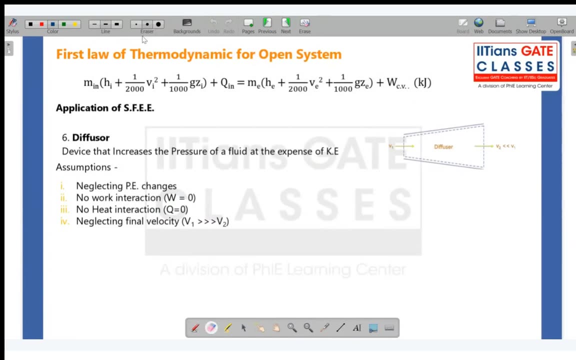 OK, And this is joule equation, Is it clear? OK, very nice. Next is diffuser. diffuser, I mean diffuser. what does diffuser do? It decreases the velocity and increases the pressure. OK, it increases the pressure. 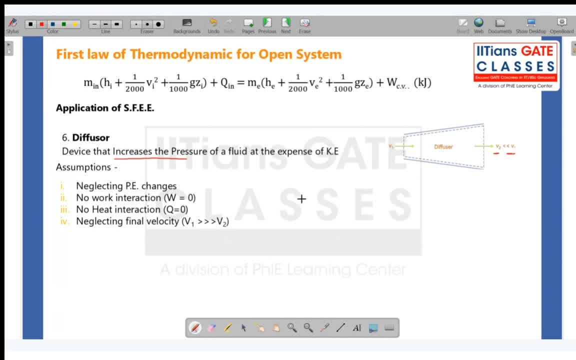 But velocity means exit velocity is much less. So now I can neglect exit velocity again. Work is zero, It is insulated. Potential energy and kinetic energy you cannot neglect. OK, so basically, what do you have? m dot i, h i plus v i square. 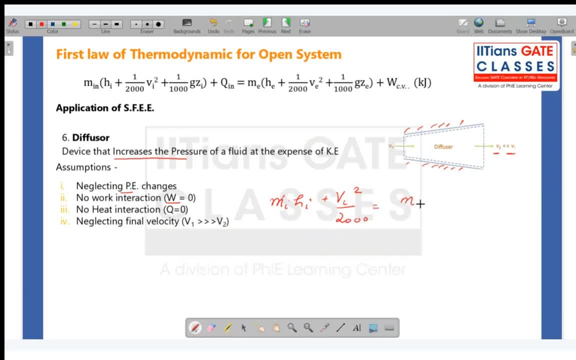 v? i square by two thousand is equals to m? e h? e. OK, Here also you will get, here also you will have plus m? i. Now m i you can take common or OK, just one second plus v? i. OK, so you can cancel m i. m i v? i is equals to under root two thousand. 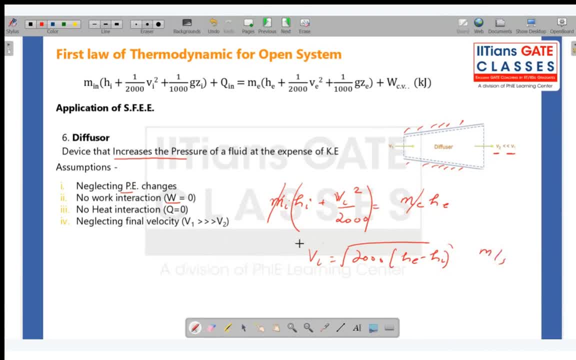 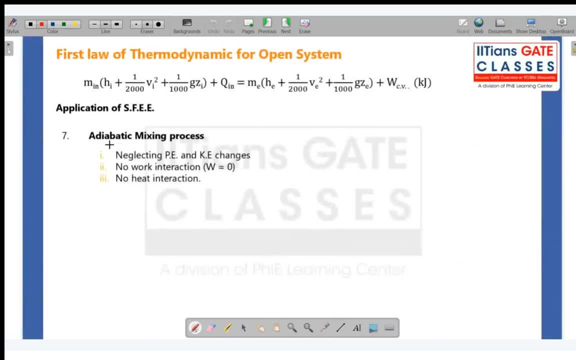 So you can calculate what is the inlet velocity. So you can calculate what is the inlet velocity. OK, so you can calculate what is the inlet velocity. OK, similarly, there is adiabatic mixing process. So it is same thing. 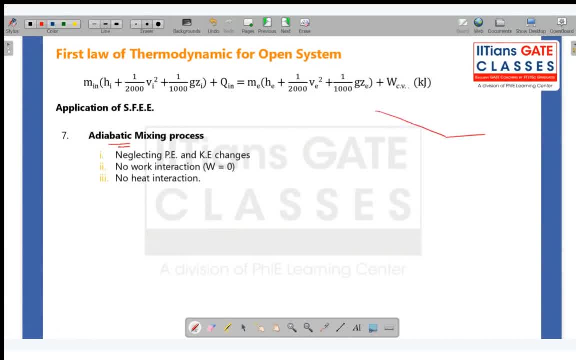 It is what we have discussed earlier. So it's like Fluids: Three fluids are coming in, one fluid is coming in here, one fluid is coming in here and this fluid is going out. OK, let us say m one is here. 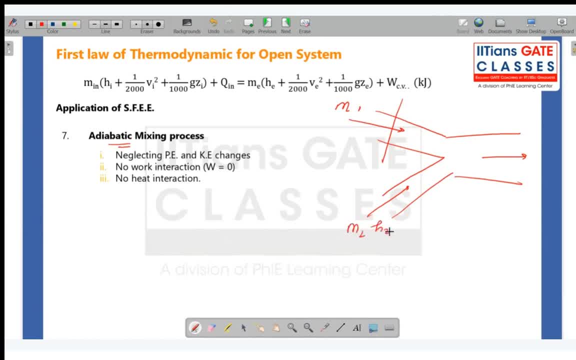 OK, One is here, M two, h two, h one at temperature T, one at temperature T two. And here what is going out? M three is going out. So what do we know? I know that m one plus m two will be equal to m three, because mass conservation. 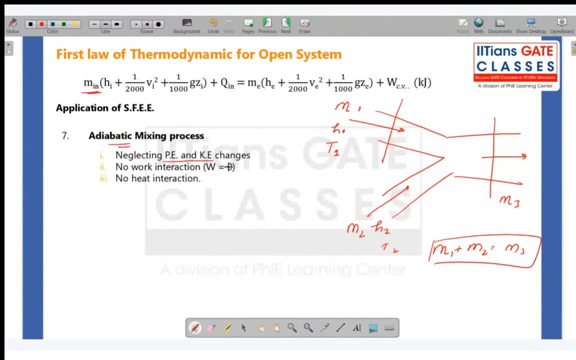 But if I apply this here, so what is? I can neglect kinetic and potential energies. no work done, and again it is insulated, So no heat interaction. We are just applying the energy question here, nothing else. OK, so m one, h one. this is entering. 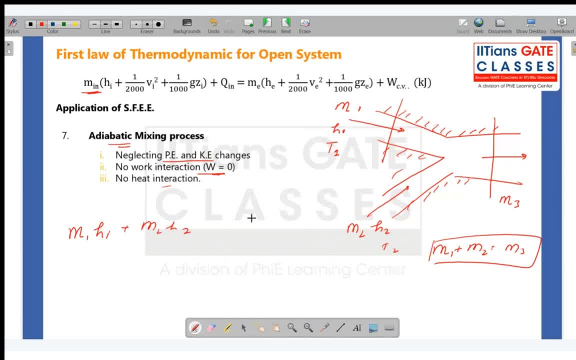 What else is entering? M two, h two is entering What is going out: M three h three. I can write: m one h one plus m two- h two is equals to m one plus m two H three. So we can use this equation to calculate enthalpy of the final exit fluid. 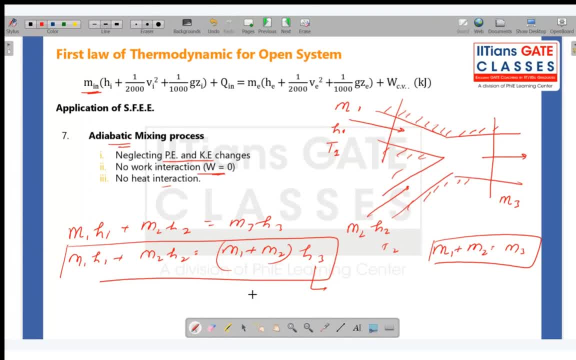 OK, now again I know, look, I do not need to do so many applications and I don't think anyone does so many applications in the class. They usually. what you do is they will teach you a steady flow energy equation. They will give you two, three applications. 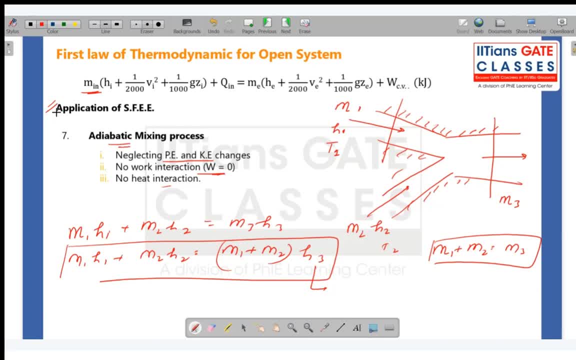 maybe a heat exchanger, nozzle, turbine compressor, and they will be done with it. Then, once the question comes, then you will struggle with. you know what concept I can apply here, But I am giving you questions in the form of application. 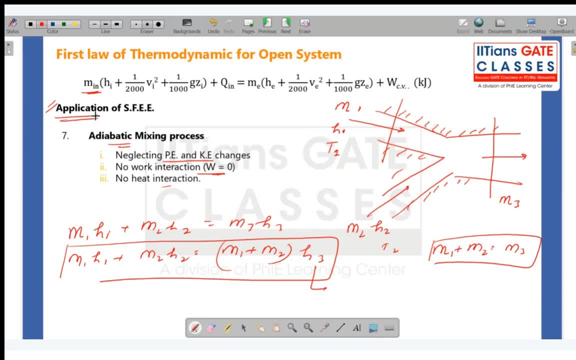 So these are all questions that they have asked earlier, But I am just giving you everything in terms of applications. OK, just writing the application and giving you that thing, But now you can directly. whenever you see these type of questions, you can directly apply. 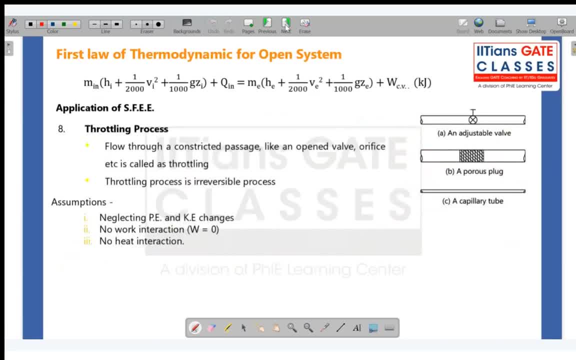 OK, The next is throttling process. the throttling process I hope you all know. throttling process is basically then, you know, like when you let the fluid pass through a very small hole, so like here, it is filled with fluid, and you open this wall a little bit and the fluid drop by drop, drop by drop. 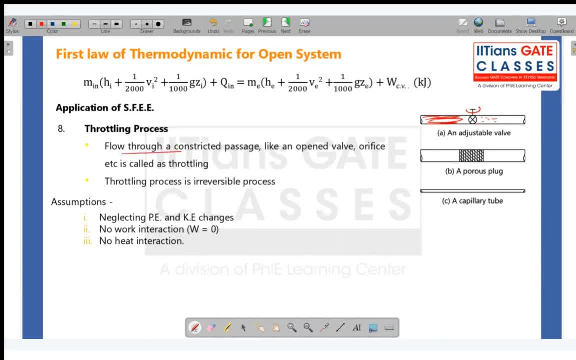 It will come here, OK, so this is called as throttling, So flow through a constricted passage like an open wall, or if it is called a throttling, And of course, you see, Here the friction will be highest because whatever is coming in, it is in contact with this wall. 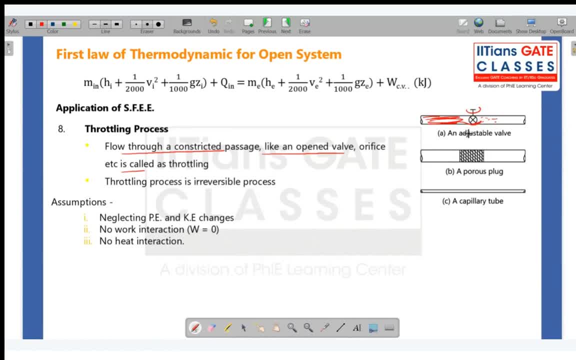 There's a solid body. So here you cannot neglect friction. OK, because you see this is pipe here and the fluid is flowing, So only friction. This fluid is going to experience friction here at the boundary, not in the middle, OK. so here maybe you can neglect. 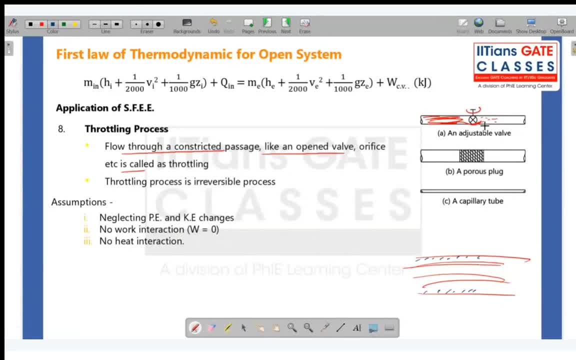 Friction and you can assume it is a reversible process. but in throttling process, whatever is going to come in it is going to cross. There is a little space, it is going to rub in this wall and therefore you cannot neglect the irreversibility here. so it is an irreversible process. 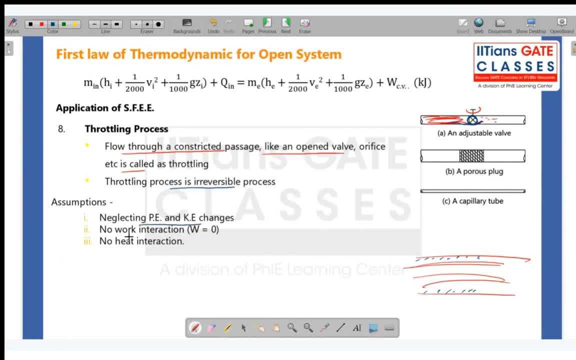 OK, Now We are neglecting kinetic and potential energy. no heat interaction, no work interaction. So this is zero. This is zero. Everything is zero, This is zero. So basically, M-I-H-I is equals to M-E-H-E. 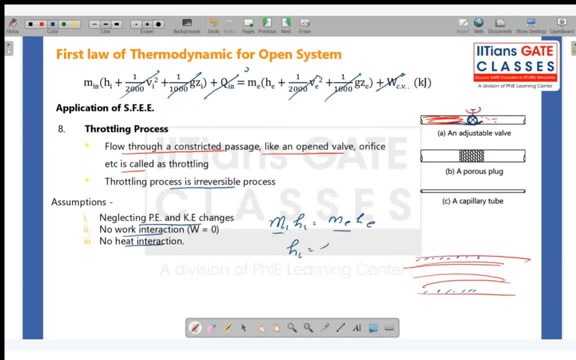 OK, So we also know that M-I-M-E is same, So enthalpy is same. So basically I can say that throttling is an iso-enthalpic process. Enthalpy remains constant, Iso-enthalpic, Iso-enthalpic. 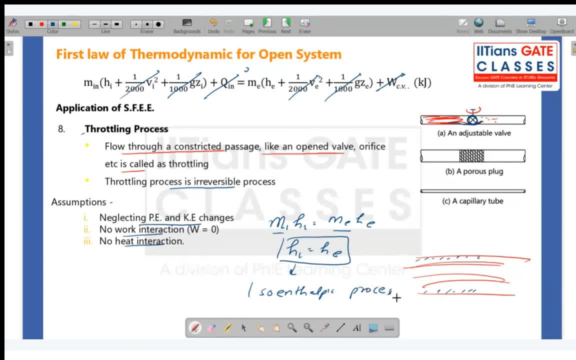 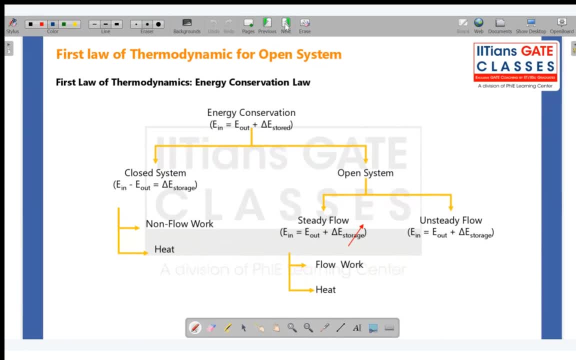 It is again an objective question. OK, it is again an objective question. OK, so I hope we are good Till here. Are we fine? Again, we will solve so many questions that everything will be clear. OK, I know that in this class I am little. 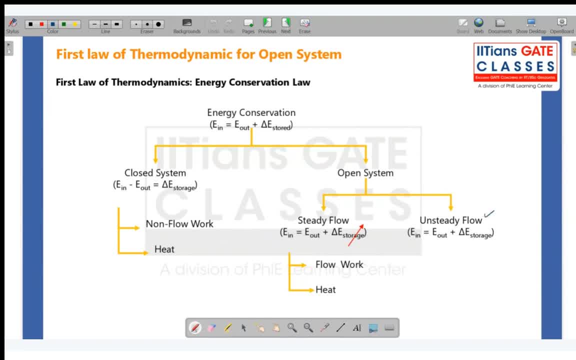 fast because I want to cover the concepts. So now unsteady flow is left. We will cover next 15-20 minutes, But we will compression expansion process in open system analysis. What do you mean? compression, expansion in open system? Turbine or compression, are you asking? 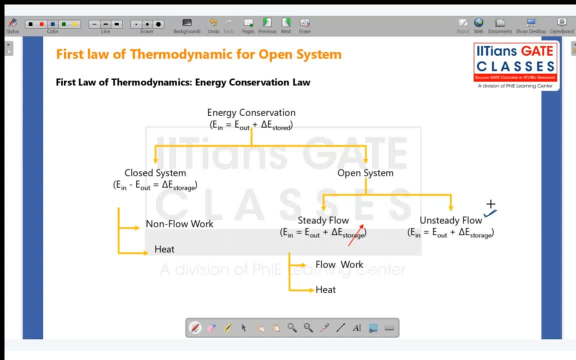 Mass in and mass out. I have. I think I have explained in general. I mean, look, it's a very wide question that you have asked. I am. I'm really finding it hard to narrow it down, But what should I explain you? 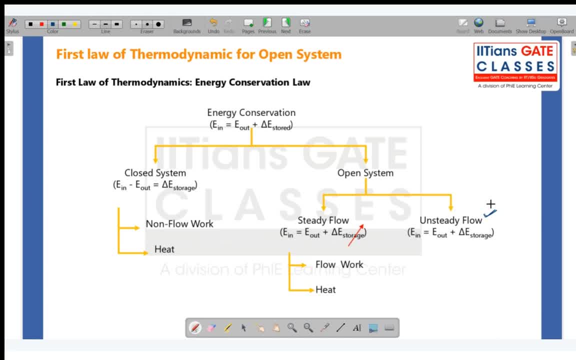 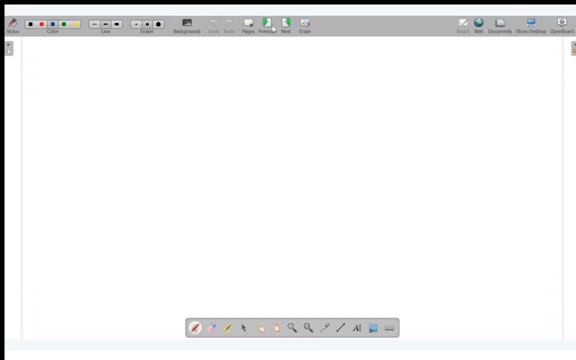 OK, ask something specific and I can explain that. But if you just ask, explain mass in and mass out, It's really difficult for me to narrow it down. I think what you are trying to ask is. No, I think I got what you are trying to ask. 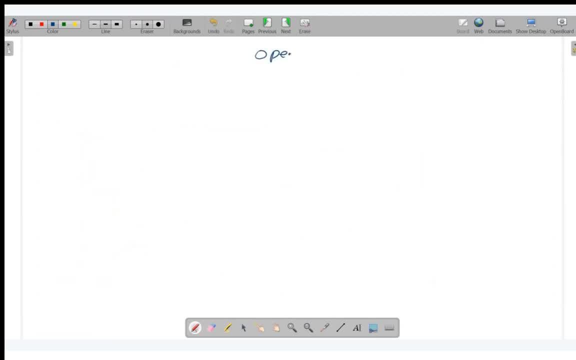 You see, this is open system: Steady flow, unsteady flow. Now, steady flow mass was entering the boundary compression phenomena. OK, look If what I've explained to you- I really request you to, because I have explained that two times- 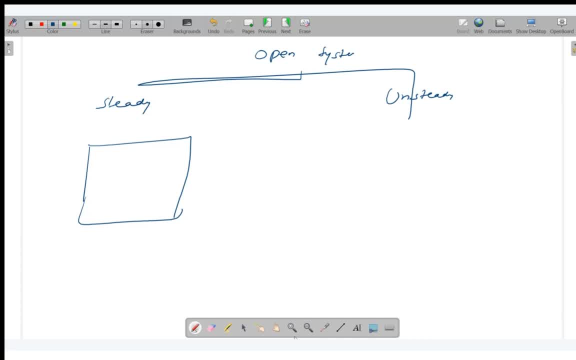 OK, now what I want you to do is you go whatever I have explained to you- I know that you want to. You're asking me to explain that in detail, but that is absolutely not required. Whatever I've explained to you, I've explained in very detail, and that is more than enough. 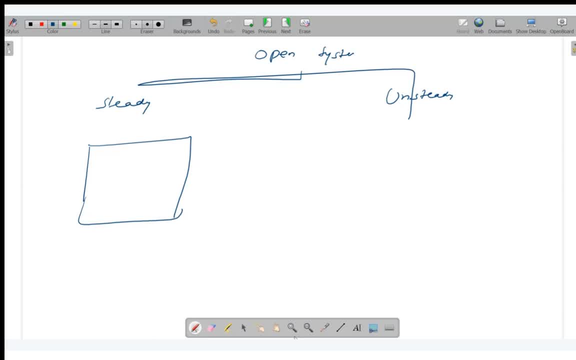 OK, but what you can do is you will get this. If you have a recording in the night or tomorrow morning, you can go back and try to go through it once. If you have any doubt. we have next class on Friday. You can ask any doubt, because if I go through that again, 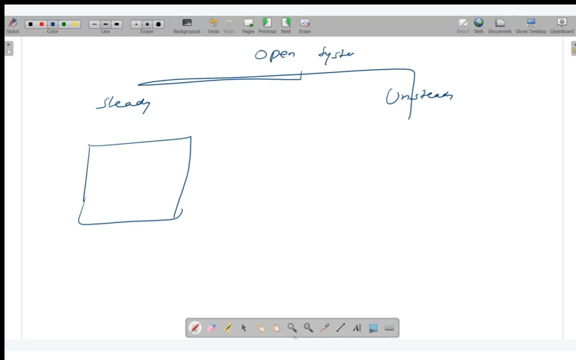 I think I already explained that two times in class today itself. OK, so if I go that again, then I think we will have time issues. Please just go to the recording. but I do. I have explained more than enough that Whatever is required, of course. 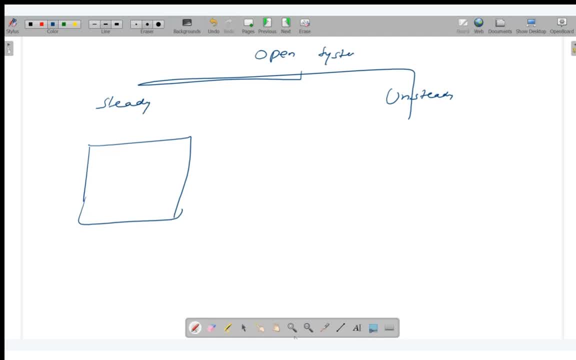 we can go in much detail with each and every topic and I can go. believe me, I can go. OK, I have done from IIT Kharagpur and I have done projection thermal engineering. I have worked on convection. 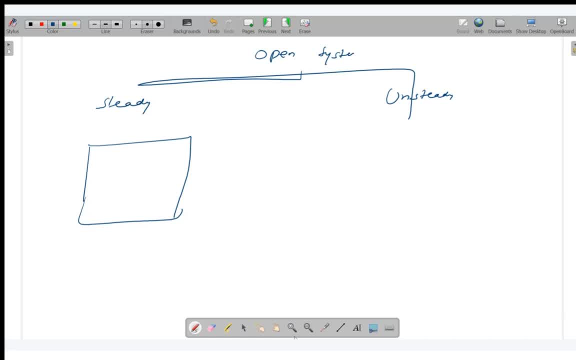 I have worked on open systems, So it's not that I don't want to go. I really want to go, But it's just a waste of time, for I mean based off your time as well as mine, because we are here for a particular objective. 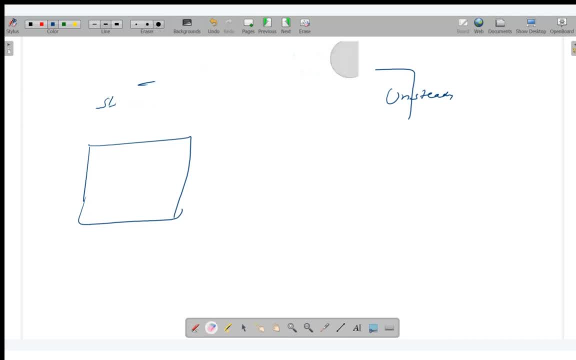 OK, So I think then we can move ahead. Let's finish unsteady state systems and then tomorrow we'll focus on- I mean, next time we'll focus on questions and we will see each and every type of question. So whatever doubt you have today, it will be clear. 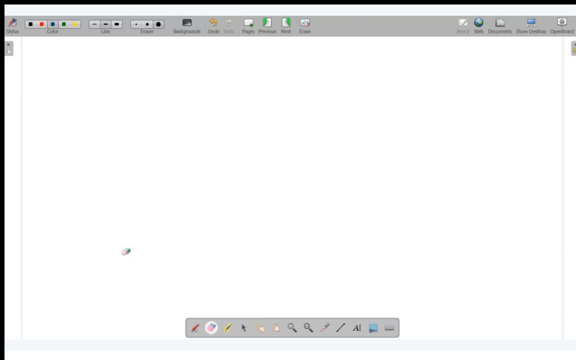 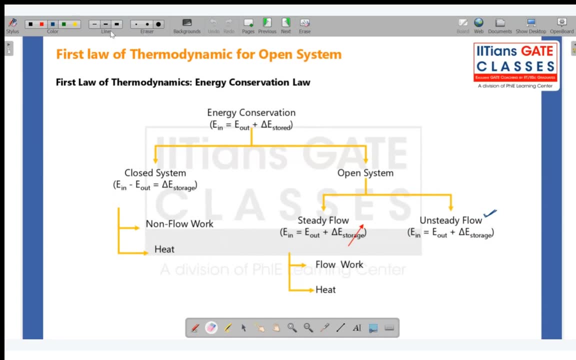 OK, and I would request to revise also before the last next class, because we will be using each and every formula that we have discussed today. OK, So now our focus is this: unsteady state. Our focus is unsteady state. Now here is steady state. 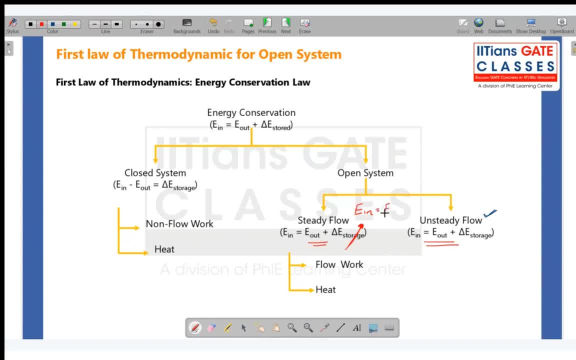 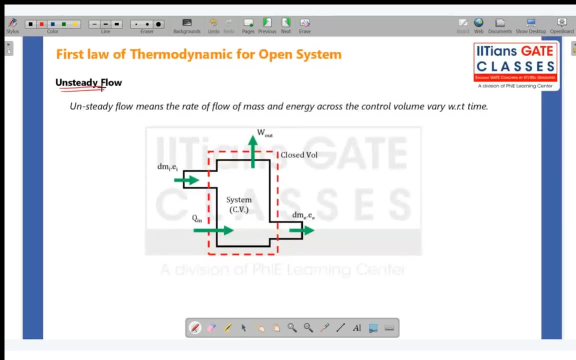 This was zero. Why? Because energy in was equal to energy out and mass in was equal to mass out. So this was zero. But here it is non zero. Here it is non zero. So what is unsteady state? Unsteady state flow? unsteady flow is basically rate of flow of mass. 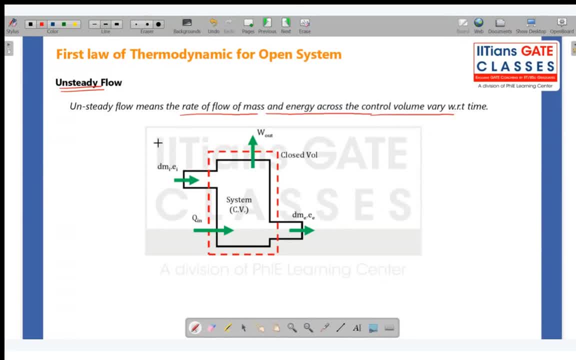 and energy across the control volume very with respect to time. Simple meaning is: Mass entering, let us say, is 10 units or 10 kg per second, And mass that is coming out is five Units. So that means mass of the system is bound to change. it will increase, right. 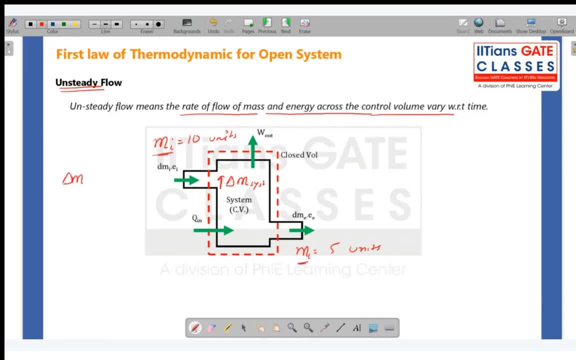 Because more mass is coming in, less is going out. So mass of system, The mass of the store, is the rate of change of mass. of storage is not equal to zero, Yes. Similarly, energy that is coming in is not equal to mass. is bringing energy right? 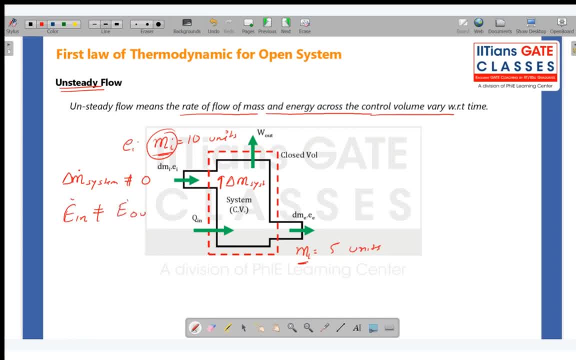 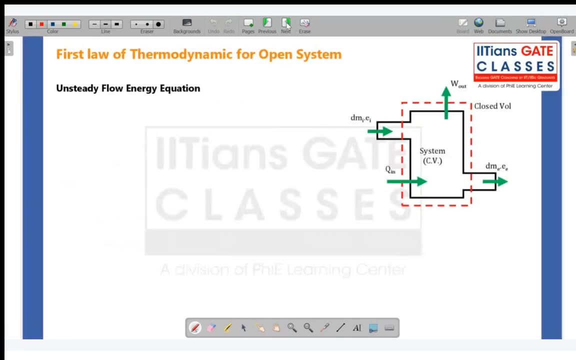 So if mass is not equal, that means energy is also not equal. So energy out, and therefore energy of storage or energy of system is also not equal to zero in this particular case of unsteady flow. OK, now I would request each and every one to be very focused. 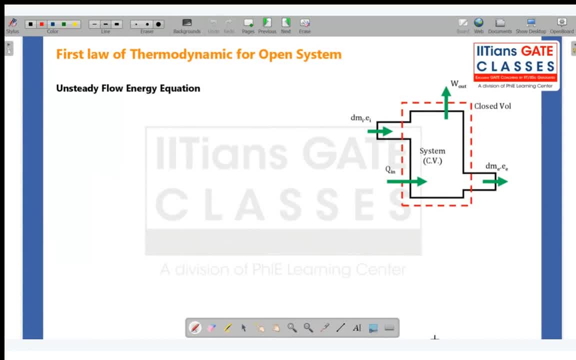 whatever you are doing, because I am going to give you a very big question And I will try to explain each and every word out of it. But if you do not focus, then you will ask me three times to explain that again and again. 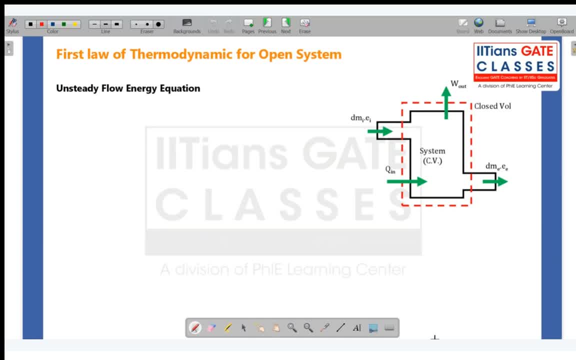 But I will explain no problem. But I would ask you to, for 10, 15 minutes, be very, very focused And I will explain each and every point and you will understand also. But if you don't understand now, I think you will not understand it again. 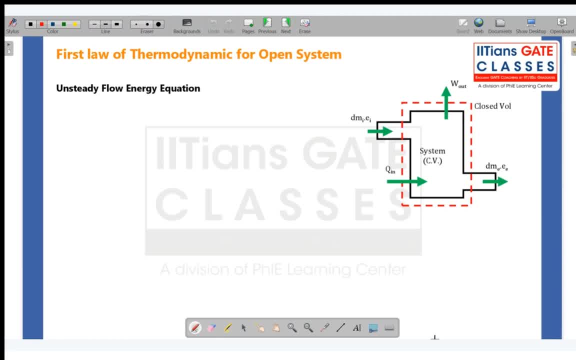 OK, because I cannot explain it again with that efficiency with which I am going to explain it in the first time. OK, So again, like we started with the steady flow energy equation, we will start with the first Law of thermodynamics. what is that? 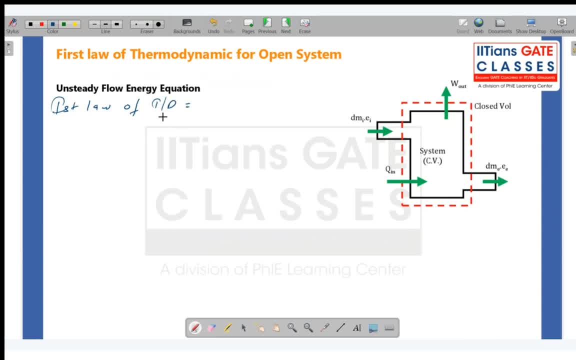 What is first? law of thermodynamics. Quickly, Energy conservation. That means energy in is equals to energy out, plus change energy of stored into the system. OK, steady flow. we took it at zero, but this time we cannot take because it is not zero. 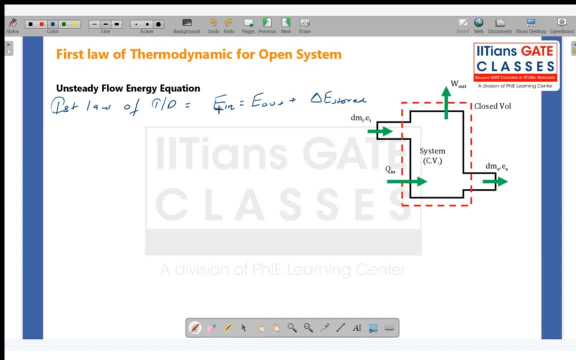 It is not zero. OK, now let's see what is going in. What is going in? So you see Again. I'll explain you two or three things here. Let us assume that the initial mass of the system is MI. 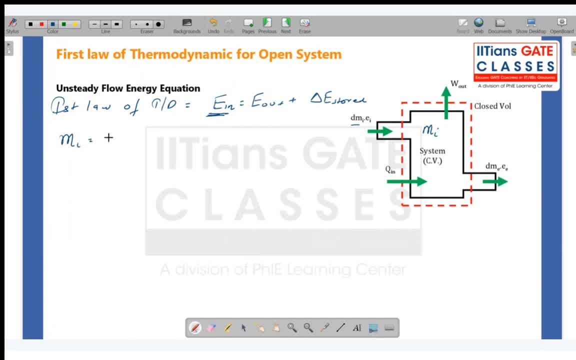 So am I very be, very focused- OK, so am I. is initial Mass Inside control volume. every point is important inside control Volume. What is M final? You see, some mass is coming in, some mass is going out, but it is not same. 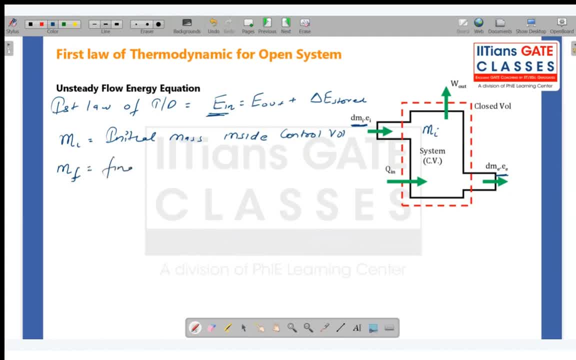 That means M. final will be something else And that is final mass Inside Control Volume. What is M1? M1 is mass entering the control volume. entering The control Volume. What is M2? M2 is mass leaving the control volume. 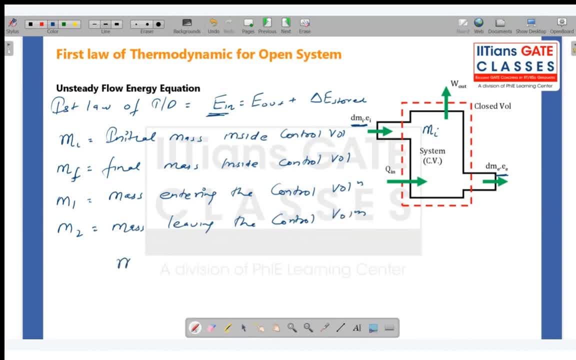 Mass, leaving the control volume, So whatever mass, OK, OK, OK, OK, little, little, little little. Just one second, Just excuse me. I have messed up with the conventions and I we are always taking As in: 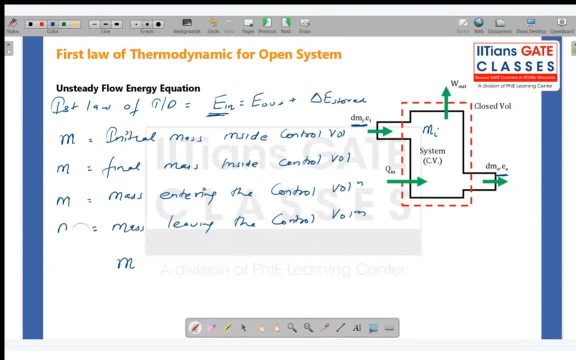 OK, let me. MI is basically, we are always taking mass entering in the control volume And exit. we are taking mass leaving the control volume. This one- M1. Is basically the initial mass inside control volume and M2 is the final mass. 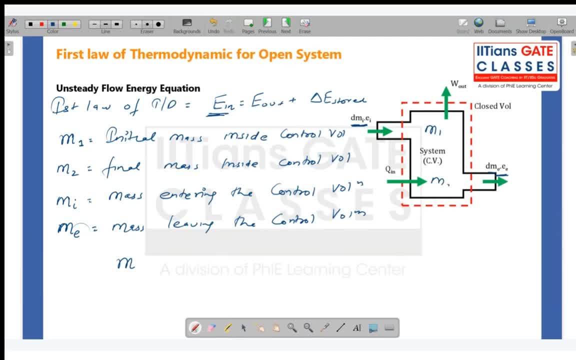 M2 is the final mass. This much is clear or not? This much is clear: just convention, just convention. and it is very important I'm telling you, because you will get confused. OK, Everyone, is it clear convention. I'm already warning you, you will get confused. 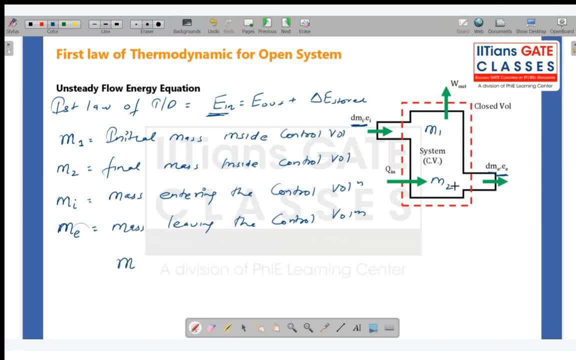 That's why I want to make sure it's very clear. OK, So I can say that M- what is entering minus what is exiting- is equals to change of mass of control volume, which is M2 minus M1, M2 minus M1.. 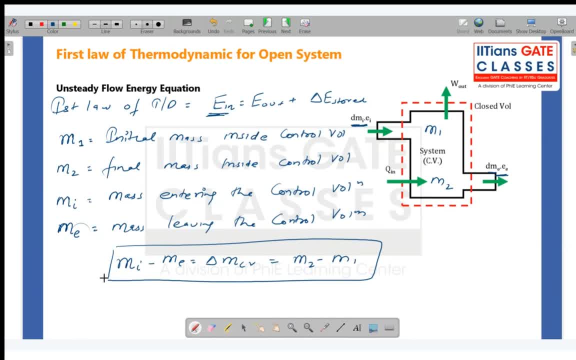 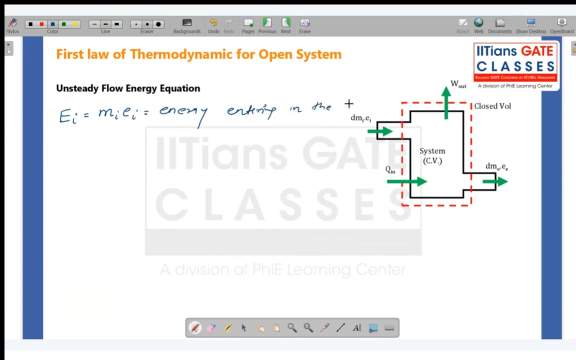 OK, Same thing we are going to do with energy. Same thing we are going to do with energy. So you see, EI. EI Is equals to MIEI Is equals to energy Entering In the system. OK, 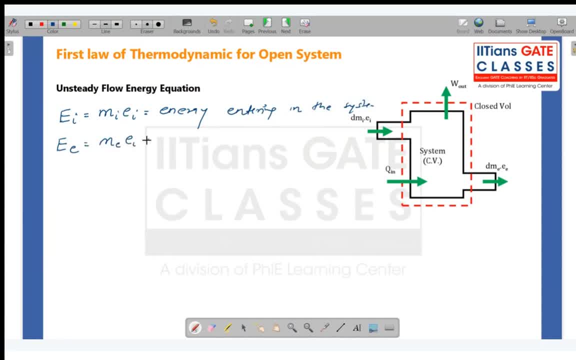 M. exit. MEEE Is equals to energy leaving or exiting the system. E1 is equals to M1.. E1. Is equals to energy or initial energy. Let me write Initial Energy Inside That control volume, whatever the mass here. 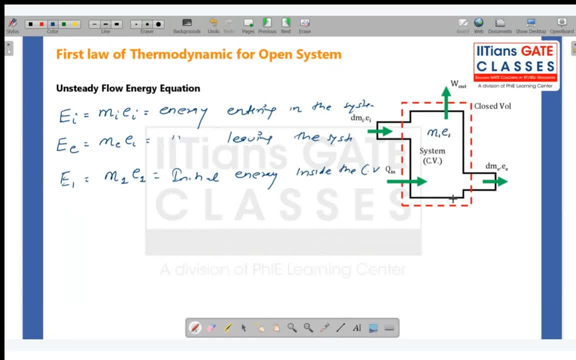 is, due to which it will have some energy, even OK. Now, this is because M2,, E2, it is the final energy, final energy. Every point is important. Be very aware of the convention. So this is I, this is E, this is one and this is two, initial and final. 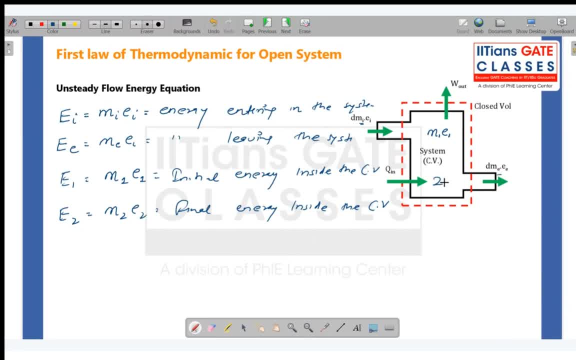 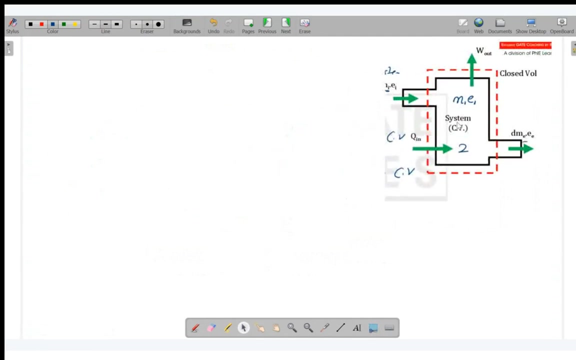 Is it clear? I want answer from everyone. Is it clear? OK, now, as I said, OK, as I said OK, I have exhausted the pages previous. OK, I have exhausted the pages previous. OK, So, As I already explained to you that, when I apply a first law, I will get energy in is. 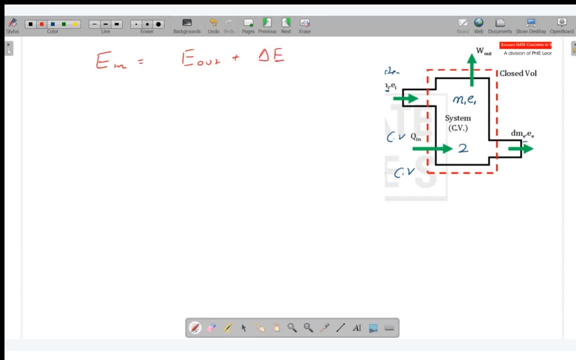 equals to energy out plus change of energy of the system. OK, now what is entering? MIEI? EI Is entering, Plus Q. in is entering. Now what is going out? M exit, E exit plus work out. This much we have seen in the CD flow. 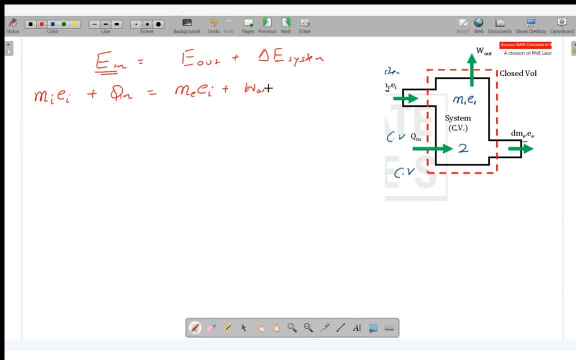 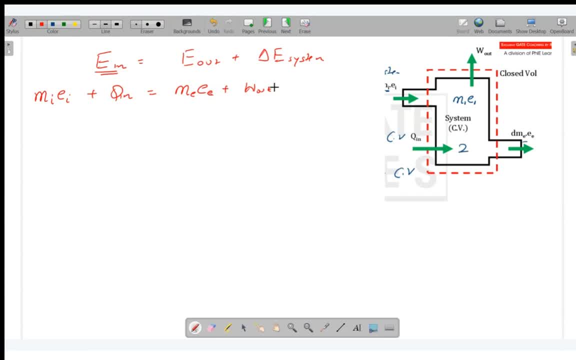 OK, work output. So this much we have seen. But their mass was same, mass in and mass out was same, So this term was getting zero. But here it is not same. So some mass will be changing, Some energy of the system will be changing. 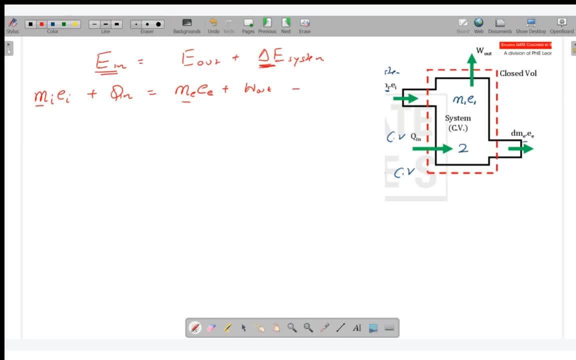 And what is this? So it will be equal to Plus By final energy inside the system, minus initial energy. OK, so what is final energy? What is final energy? Final energy is M2E2 minus M1E1.. 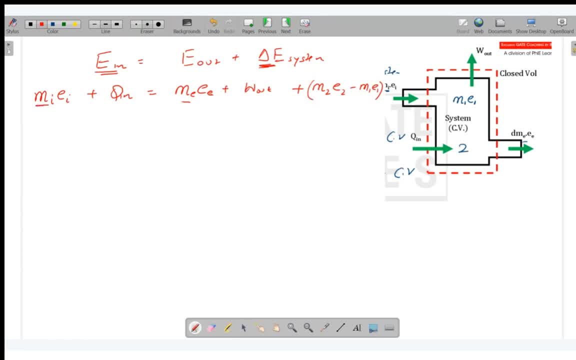 OK, now let me explain. I have already explained to you how does the mass store energy MIEI? MIEI plus VI2 by 2 plus GZI plus QIN is equals to MEUXZ plus VXZ2 by 2 plus GZXZ plus work output. 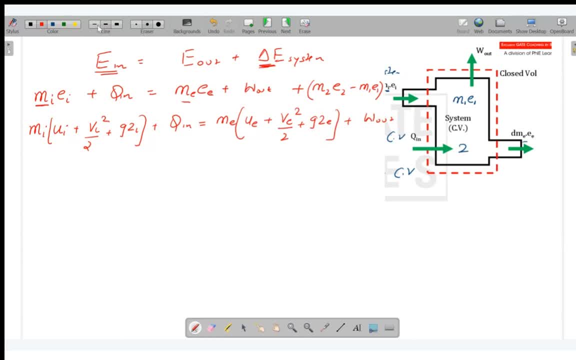 OK, now, what is this work output? Already explained to you. It is Plus Work of control volume, Plus or minus P1V1 plus P2V2.. OK, OK, one second, It is OK. I mean, I just want to. 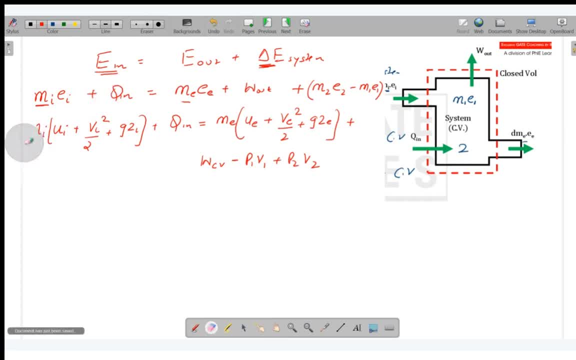 Let me write it in a way that is much clearer, And let me write it again one more time. Let me write it here, so that OK, So MIEI, MIEI plus VI2 by 2 plus GZI. 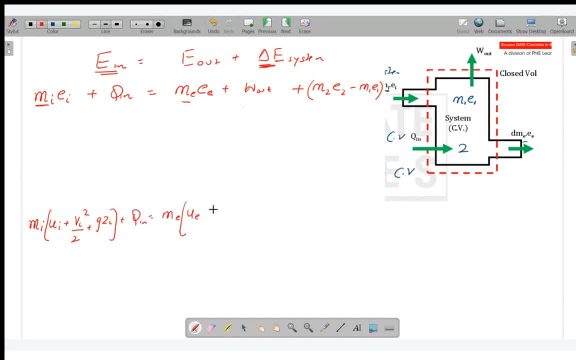 Plus QIN is equals to MEUXZ Plus VXZ2.. Square by 2.. GXZ plus control volume, minus P1V1 plus P2V2.. OK, so this is basically this, which is mass and energy entering. 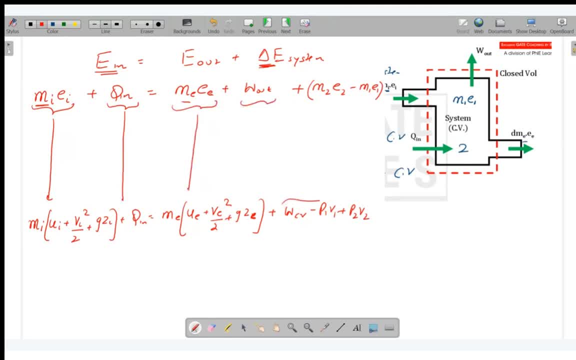 This is heat transfer. This is this, And this is work transfer. Now let us move to further part. This one Plus M2.. Now energy: U2 plus V2 square by 2 plus GZ2, minus M1U1 plus V1 square by 2 plus GZ2.. 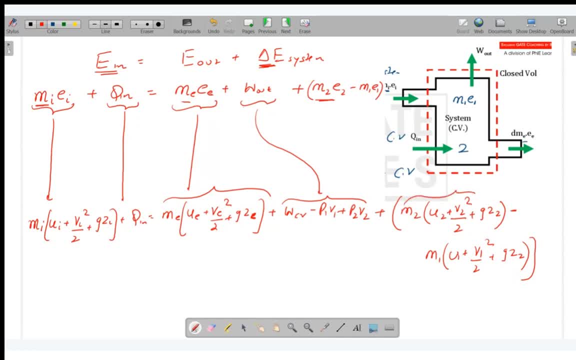 OK, so this is the very Now. this is what This is This. This is what This is This. Are you able to make sense out of this equation Z? Yeah, this one is Z1.. Yes, I'm really sorry, because I just you know. 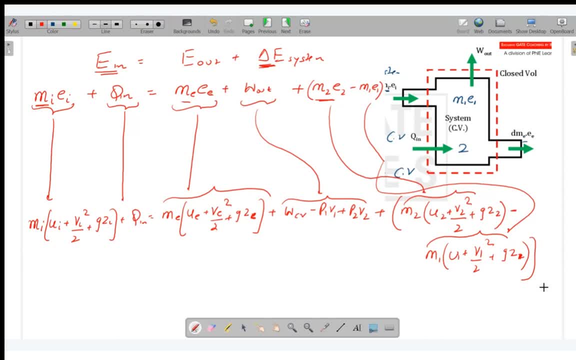 right, Right Right. Very fast to make my mistakes, But I think are we making sense here. Are you able to understand this equation? You have to check what we are looking at now. See what is this This is. Let me explain here. 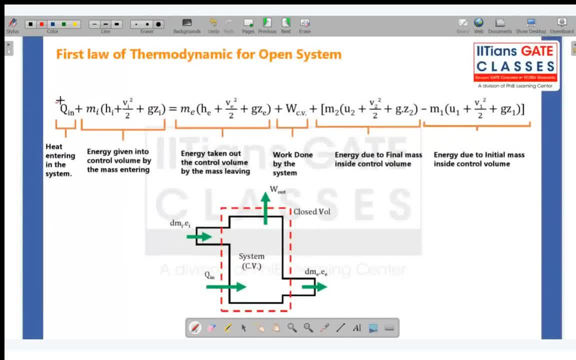 OK, so this is my question. Everything I've written here. Now, what is this Q in? It is the heat entering in the system. What is this? It is the energy given Into the control volume by the mass entering. So this mass that is going in it is taking this energy with it. 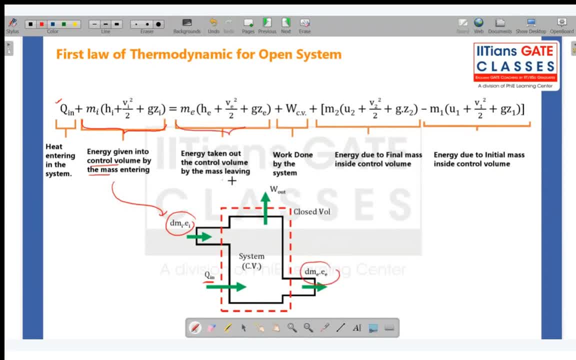 What is this? This mass that is going out. it is taking this energy out with it. OK, work done by the system. is this work done Now? energy due to final mass inside the system by initial mass was M1.. Final mass is M2.. 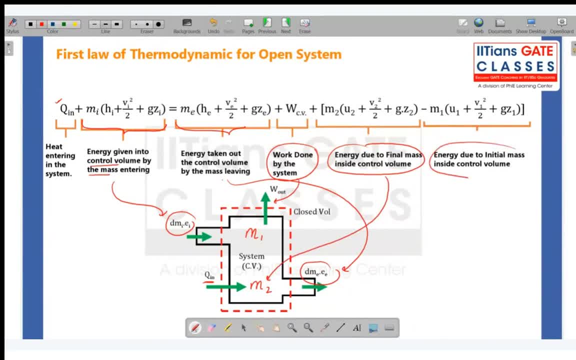 So, because of this final mass, what is the Energy? is this, and this is energy due to initial mass. So I hope this equation you have to write it at least 10 times so that it's absolutely clear to you. OK, don't make mistake in IE1. and to be very clear, 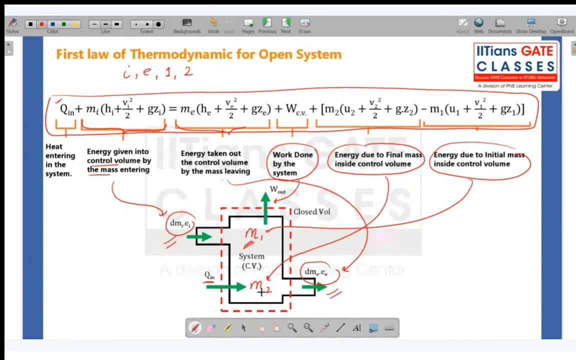 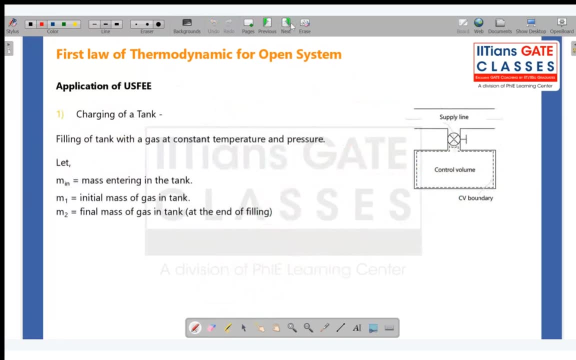 What is I? I is in, E is exit, One is initial inside, Two is final, inside Clear. OK, quickly, let us. I'll take five, five, seven minutes. So what is the application of this? charging of a tank. 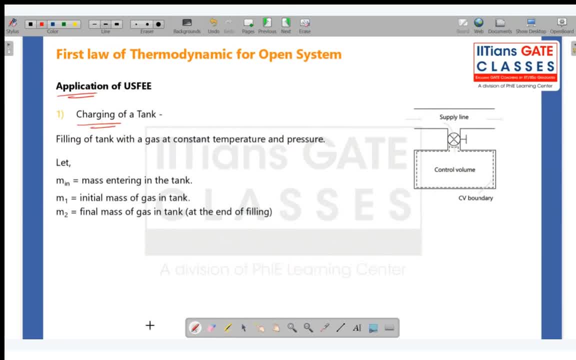 You see what is happening: charging, for example, when you fill your bucket right in your bathroom or anywhere. So what is happening? You just keep it, keep it feeling like you know, like it is going inside, That thing is coming out, or sometimes you even take it out. 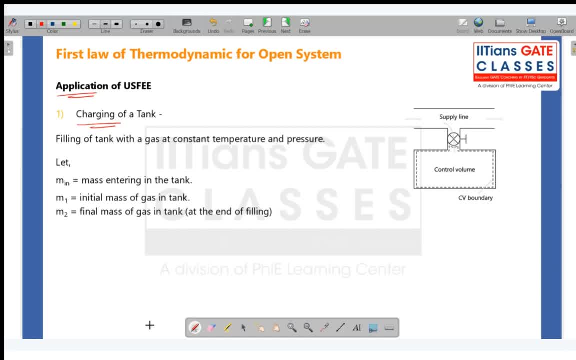 But you see, what is going in is not equal to what you are taking out. So sometimes the water level in your bucket increases or sometimes decreases, depending upon what is happening here. I mean what? how much is going in, how much is going out? 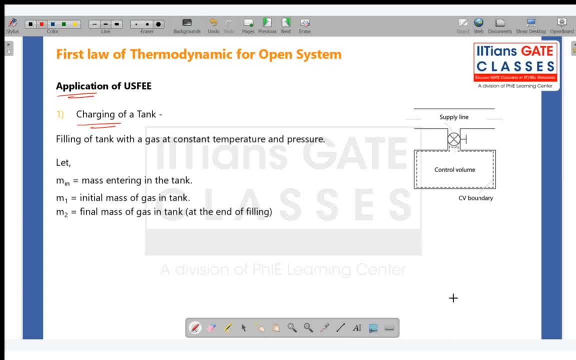 Similarly, charging of a battery. So when you, when the power is on, you charge your battery, So you don't use your battery, Only you give power and you charge your battery Right. So energy is going in, Only that thing is coming out. 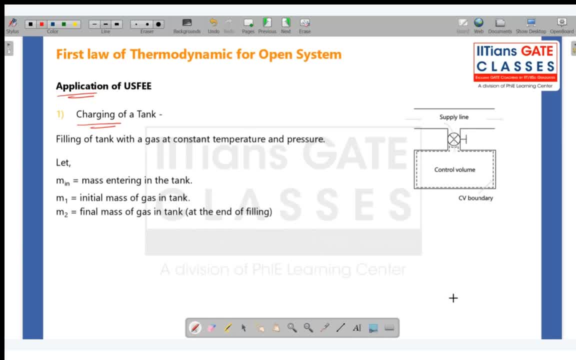 Then when the power goes off, then nothing is going in, Only power. only power from the battery is coming out. That is discharging, OK. so these are all examples of Unsteady flow energy equation. the first is charging of tank. 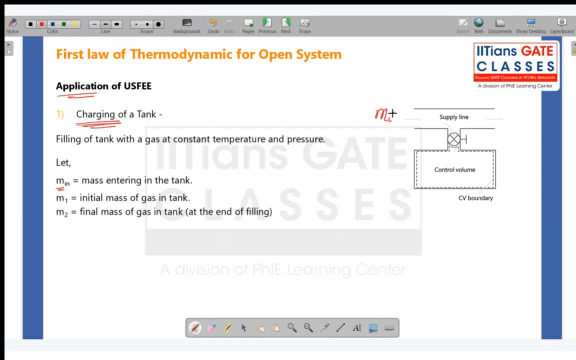 Now charging. what is mass in mass, entering mass in Initial mass is M1, final mass is M2.. Now, in this case, I am assuming that nothing is going out. Exit is zero. Exit is zero, OK. So What are the assumptions? 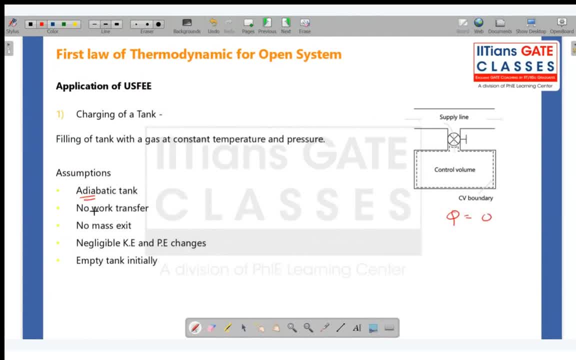 It's an adiabatic tank, so that means Q is equals to zero. Of course, only filling or emptying. you are doing so work will also be zero. I am assuming M exit is equals to zero. OK, kinetic and potential energy, I can neglect an empty tank. 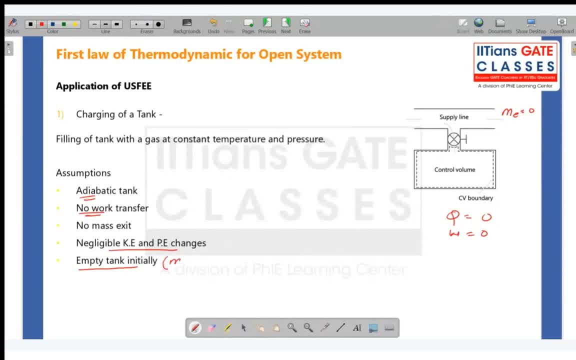 Initially, empty tank Initially. what do you mean by empty tank? initially That means M1 is equals to zero. Of course, these assumptions will always not be zero. You have to see what they are asking in question. Always start with the general equation. 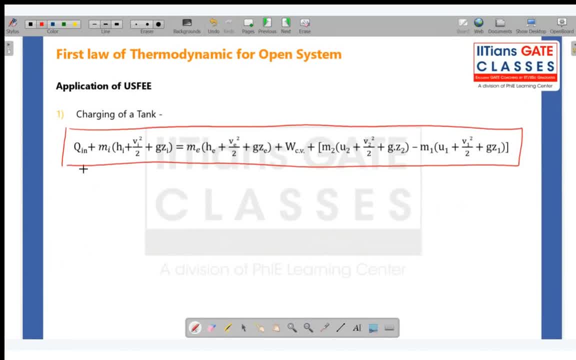 This is your most general equation, Unsteady flow energy equation. Then see what assumptions are valid. So assumptions you can apply. First assumption: Kinetic and potential energy are neglected. Second assumption: No exit. nothing is going out. that means M is equals to zero. 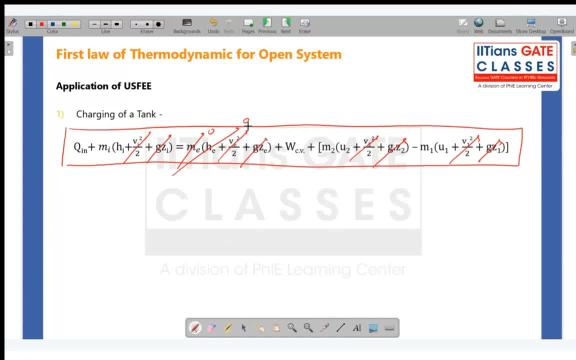 So everything this is zero. Next, initial mass: Initially it is empty. That means M1 is equals to. that means this is also zero. So everything here is zero. OK, also no work done. So this is also zero, adiabatic. 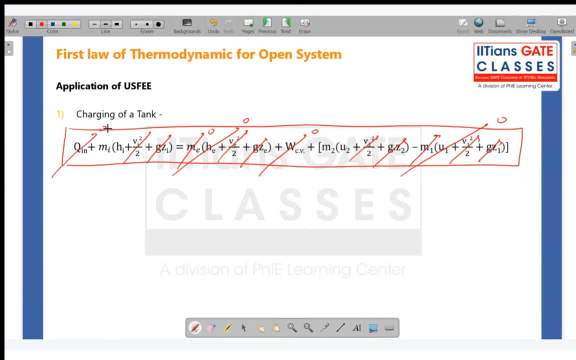 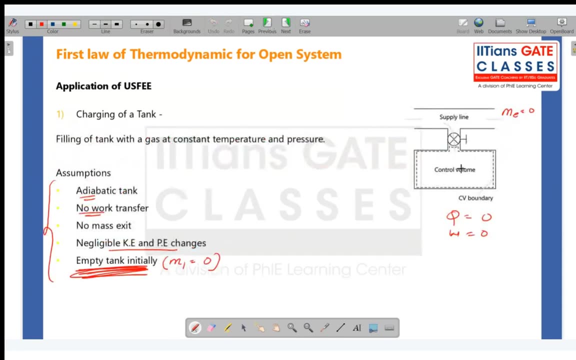 Yes, Shivendra Raj, this is zero. So what are we left with now? It is very simple: MIHI is equals to M2 U2.. And now see if. if you logically think, if the initial mass was zero and nothing is going out, that means whatever came in will be equal to M2.. 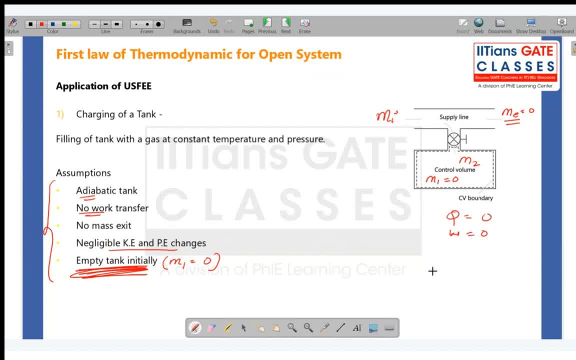 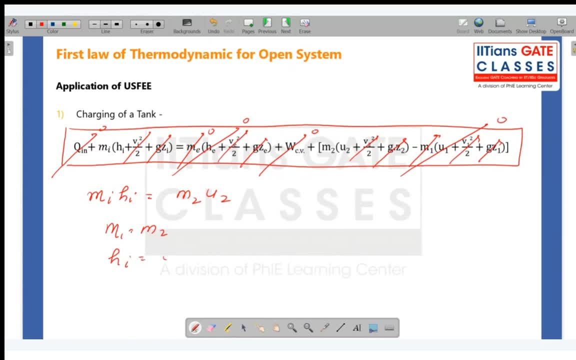 Yes, So I can. MI is equals to M2.. So basically HI is equals to U2.. So CP initial temperature is equals to CP final temperature. This is in temperature, This is final temperature inside the Control volume. So it is CP by CV TI. or you can say T2 is equals to gamma TI. 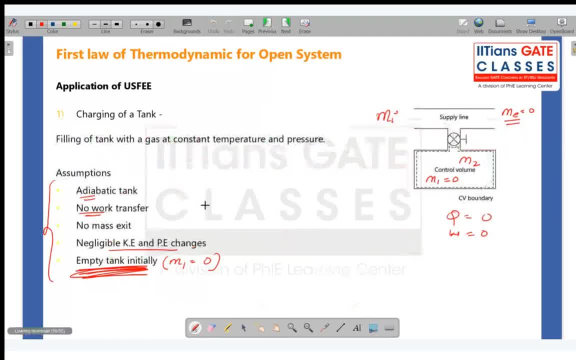 Again, make sure what are the assumptions that are applicable in the question. Do not apply blindly all the assumptions. But this is the most sought case. actually, this question has been asked in GATE. That's why I have- I have applied all the assumptions and given you. 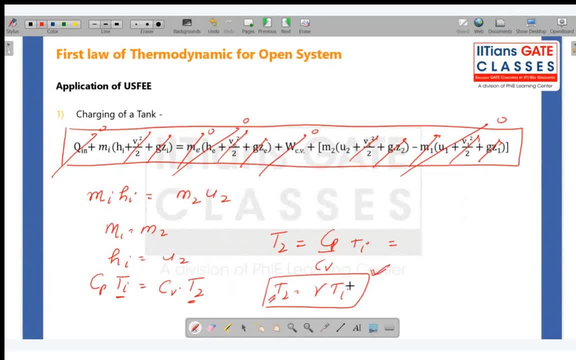 directly what, and they have asked this temperature, So you have to and they have given this temperature in the question And it's a very big question. If you see that question, it's like 10, 15 lines, But basically everything you need to cancel. 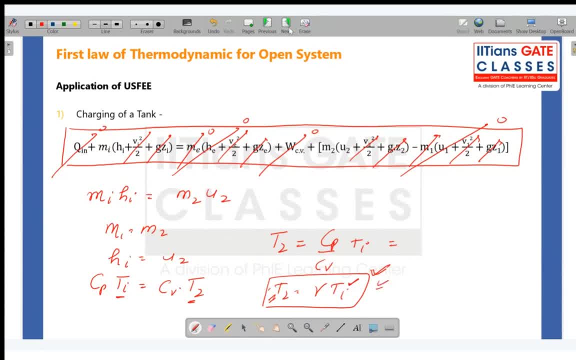 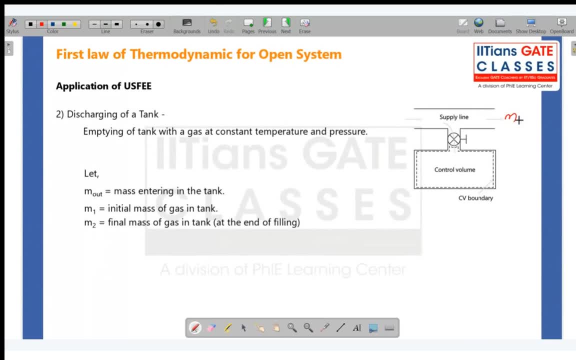 and T2. you can calculate by this formula: that's all nothing else. OK, quickly, what is discharging, emptying of tank. So now nothing is coming in. OK, so M out is basically what is going out. mass M E is mass exiting. 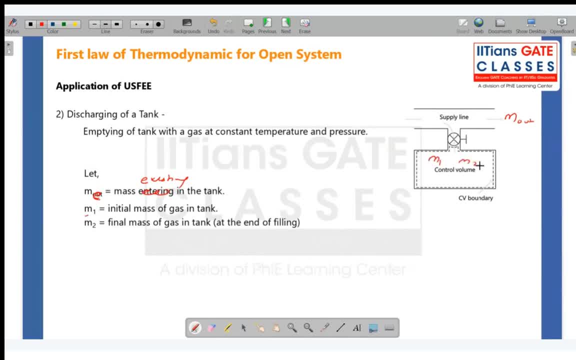 M1 is initial, M2 is final. OK, what are the assumptions? Adiabatic tank Q is equals to zero, no work transfer. This is zero. mass inlet: Nothing is coming in, Mass in is equals to zero and full tank initially. 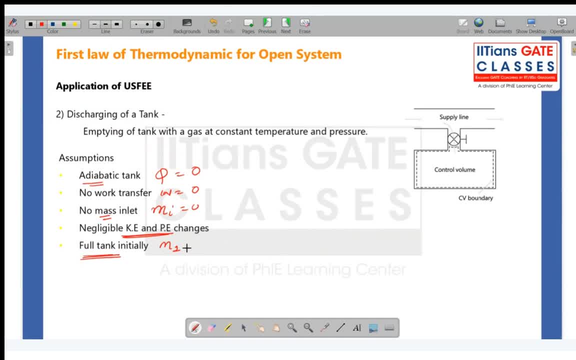 But it is M2.. M1- sorry, M1 is full. OK Now. so you see, Adiabatic, nothing is coming in. that means this: everything is zero, No work, transfer OK and What else. 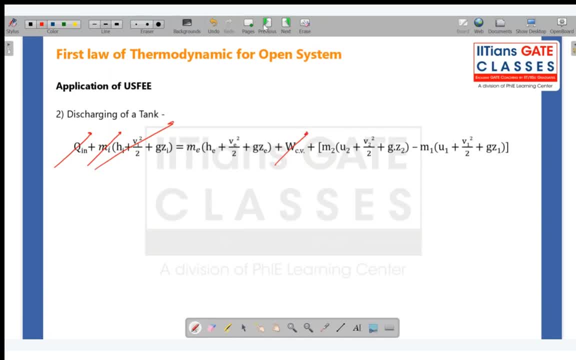 Finally empty tank. OK, I can assume one more thing here, if you want. I mean, if we can't, we can neglect it as well. Now, what is left? Zero Is equals to M, E, H, E, because kinetic and potential energy are also neglected. 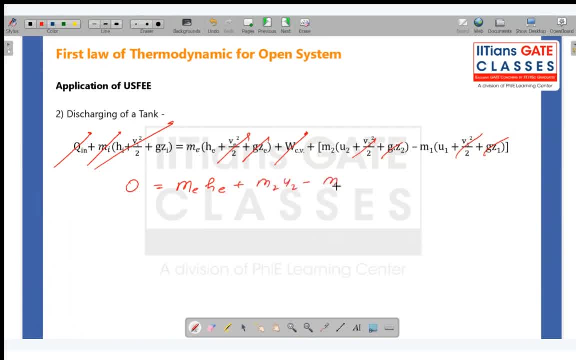 OK, Plus M2 U2, minus M1 U1.. So either you can use this equation: M1 U1 minus M2 U2 is equals to M exit H E. OK, so either you can use this equation or, if in question, 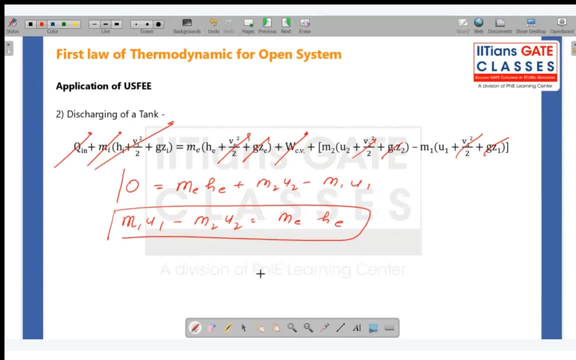 Yes, Yes, Thank you. Or if in question, they have given that finally Empty Tank, So finally empty tank. what does it mean? Yes, M2 is equals to zero, So this time M2 will also be zero. M1- U1 is equals to M, E, H, E. 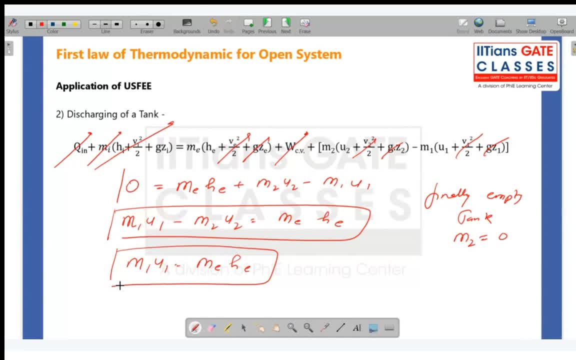 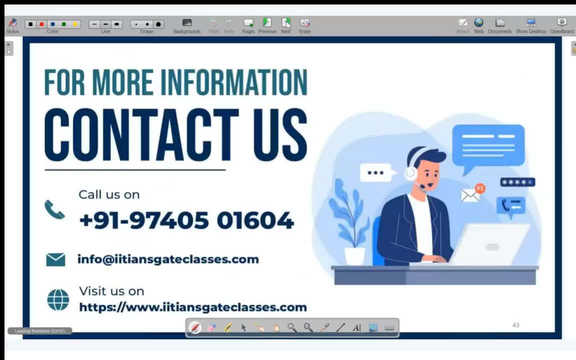 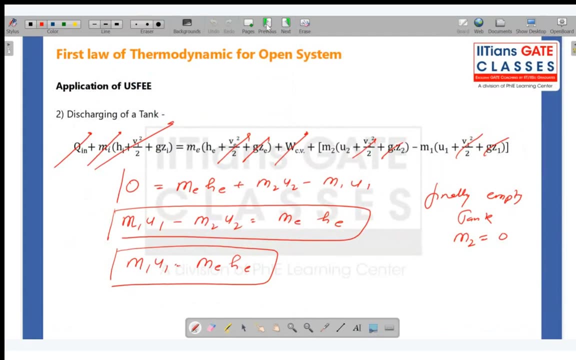 And you can apply the same logic we did earlier and you can find out your final temperatures as well. OK, So basically, this is, you know, the applications for On the steady flow energy equation. I know that I have gone a little fast because I need to cover so many things. 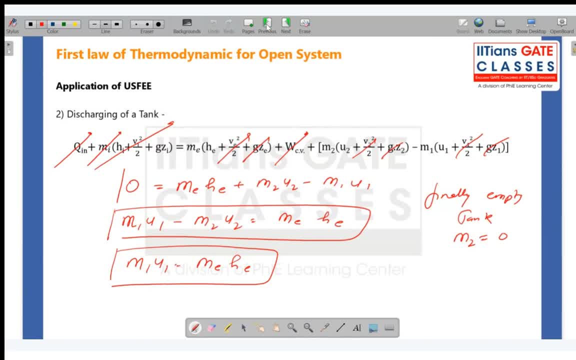 but I think I was at decent speed and I think we covered it decently. OK, So now in the next class I will come up with all the questions On first law- closed system, open system. So we solve so many questions that every